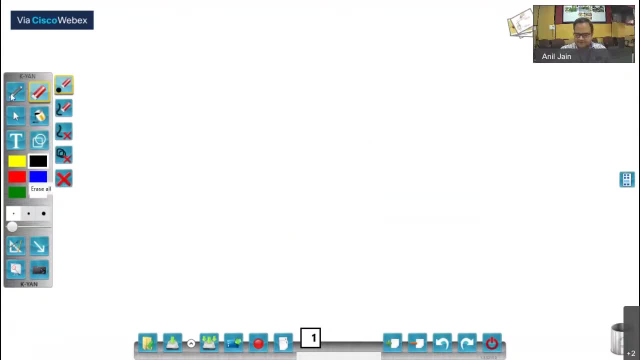 Sorry, I think it has taken some automatic format. So Nd, Fe, 0.5, Mn, 0.5 O3.. So now for this space group, this multiplicity of the side where neodymium goes is four and for this side where this iron manganese goes, also for oxygen has two side: oxygen 1 and 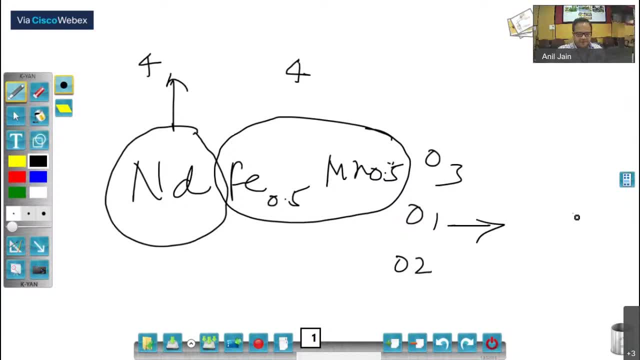 oxygen 2.. For the one side, where oxygen goes, multiplicity is 4 and for the another side, where oxygen goes, multiplicity is 8.. So for the one side where oxygen goes, multiplicity is 4 and for the other side, where oxygen goes, multiplicity is 8.. And the multiplicity of the general side is 8.. 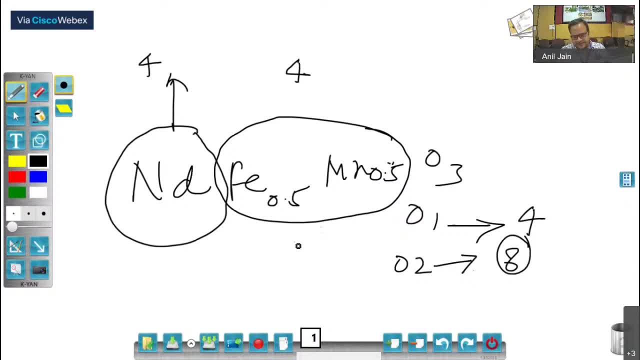 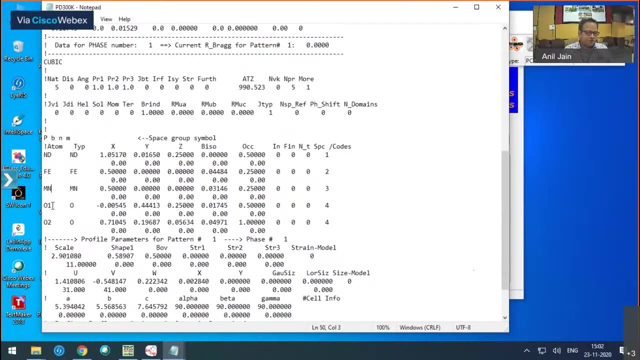 Now to get this occupancy correct, if site is fully occupied, we have to divide this occupancy of that side by this general occupancy and let us see how it looks like. So this is neodymium, iron, manganese, O1, O2.. So, as you can see here that 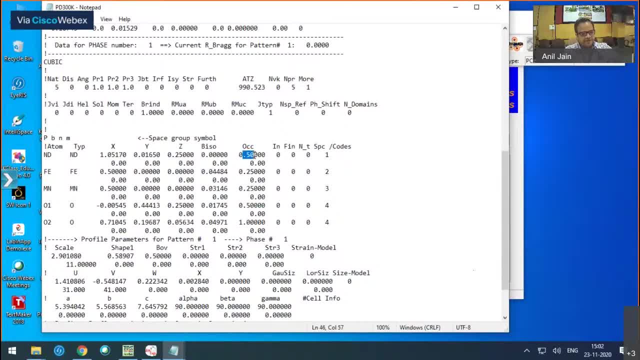 the occupancy for this neodymium is 0.5, because multiplicity of the site where neodymium goes is 4 and general site multiplicity is 8 for this space group. Similarly, in this material, this iron and manganese, So both of these ions. 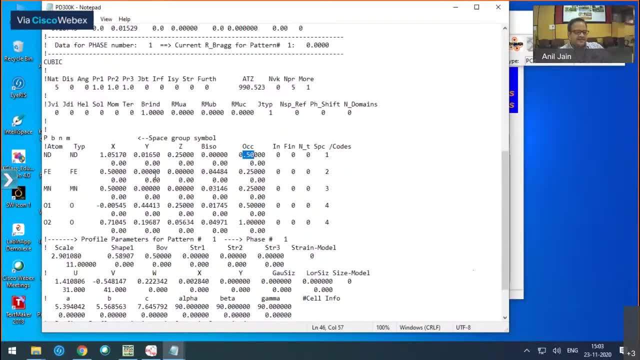 goes to the same site and the multiplicity of that site is 4.. So the total, if I take this summation of the occupancy of iron and manganese, it should be 0.5 and it is half Generation 2. So accordingly, the total occupancy for iron and manganese becomes 0.25.. This is half of channel of iron and manganese. M5m will become CO2.. The total- male- instead of the pilot, remember this- given to be 4.5.. So the total, if i take this summation of the occupancy of iron and manganese, it should be 0.5 and it is half half. so occupancy for iron and manganese becomes 0.25.. 347. agriculture of iron and manganese becomes 0, 25.. And higher food. in appearance, Koreans keep irons and manganese, for iron and manganese only memorized. Its insaccordance with this is zero point and uniformity makes 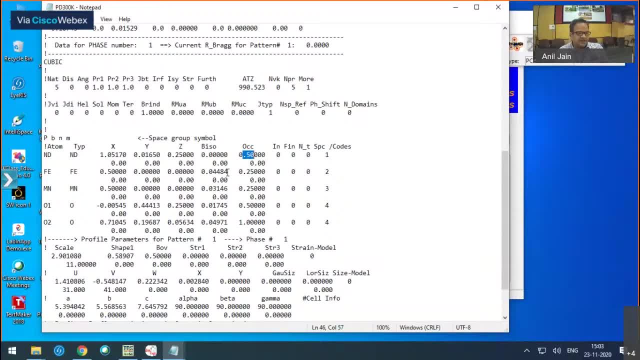 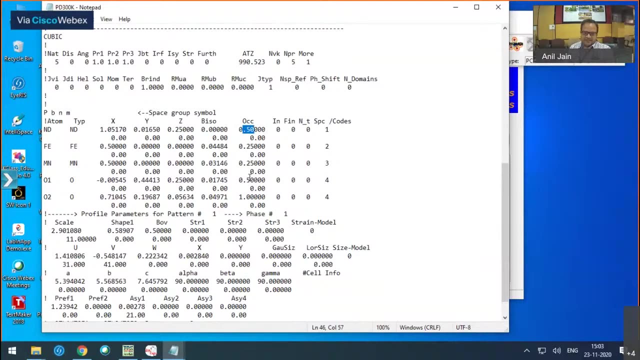 occupancy for iron and manganese becomes 0.25 and 0.25 oxygen. I told you there are two sides. for one side the occupancy is, the multiplicity is 4, and other side of the oxygen which is: I believe this is general side. so the multiplicity of this side of O2 is 8 and general site multiplicity. 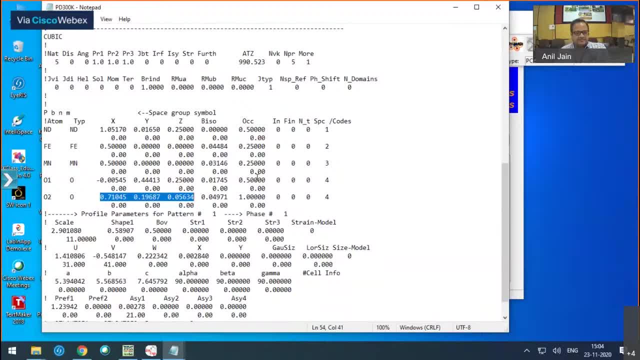 is also 8, for the occupancy for this side becomes 1.. So this is how we have the occupancy. Now, if I multiply this occupancy by the two, then I reach the formula unit. So this neodymium, I multiply this occupancy. if I multiply by half, it becomes neodymium 1, iron: if I multiply, 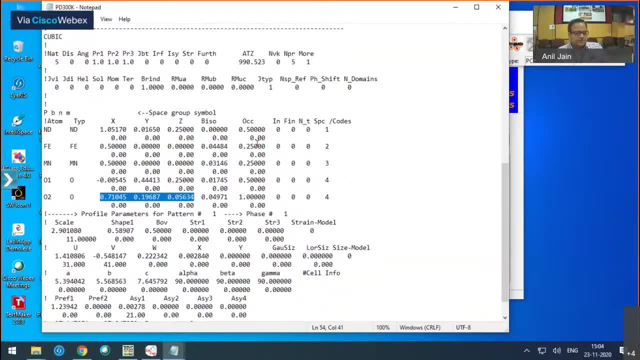 by 2, sorry. neodymium: if I multiply by 2, it becomes 1,. iron: if I multiply by 2, it becomes 0.5, and similarly manganese: if I multiply by 2, it becomes 0.5,. oxygen: 1. 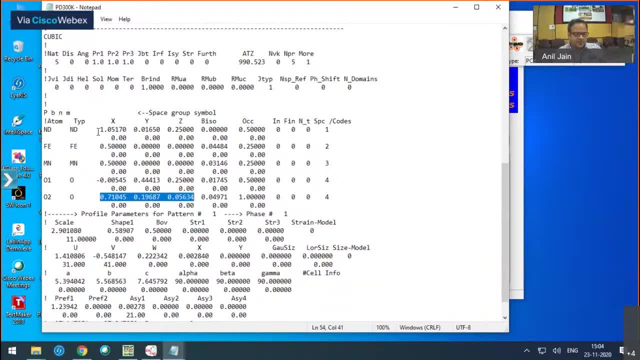 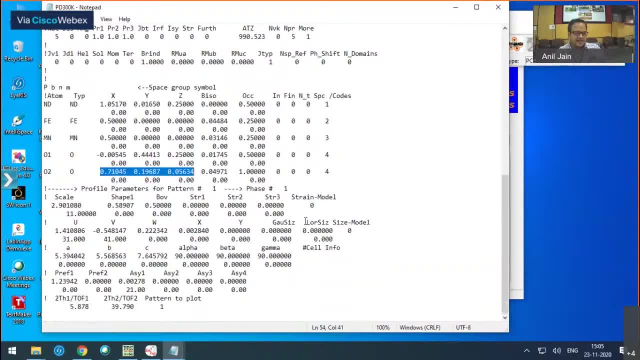 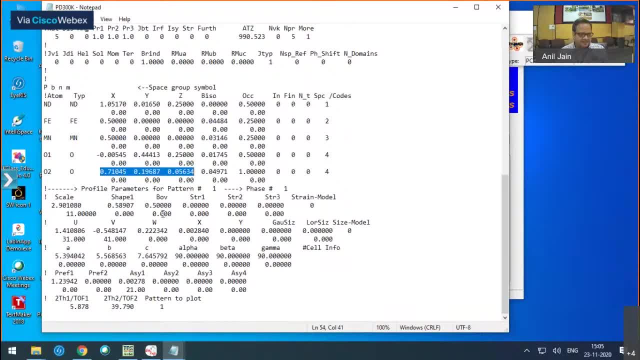 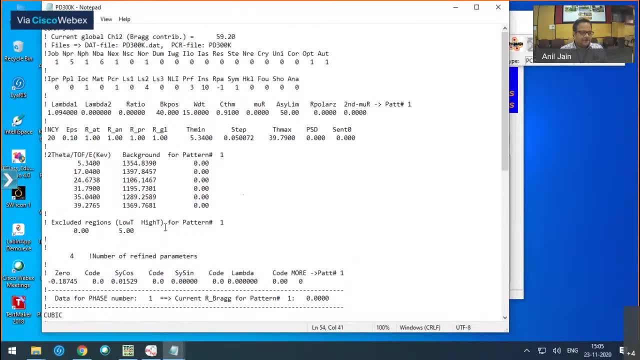 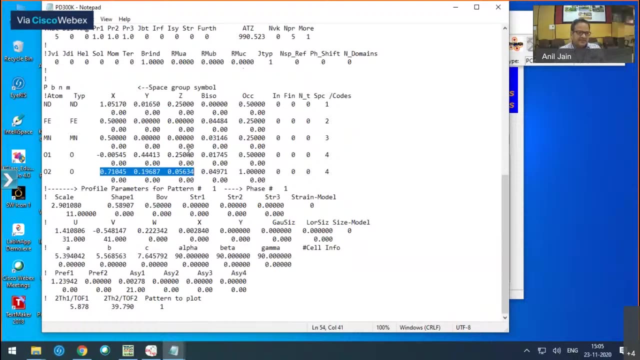 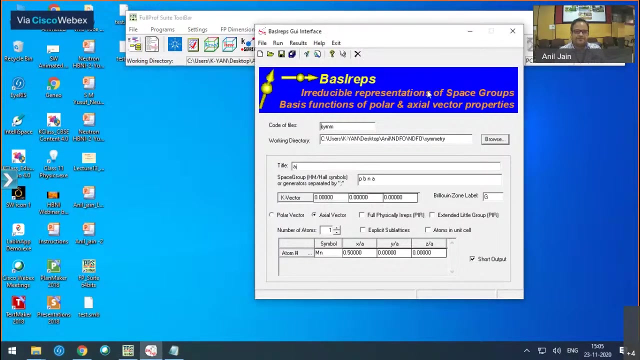 short codes, which is mentioned in this PCR file. Now, if, Now, if I have to determine the magnetic structure, then, as you know, I have to do the experiment at low temperature. So this is the data at room temperature. Now, first let us have a look at the data of this material. 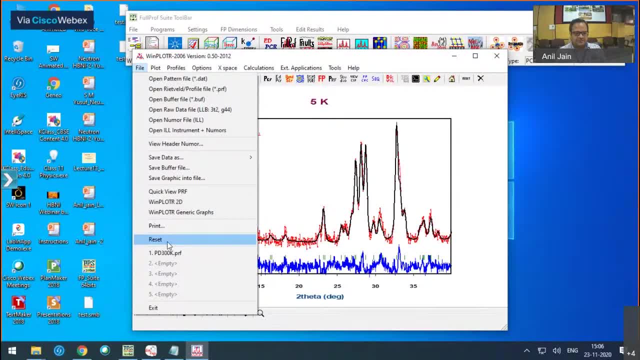 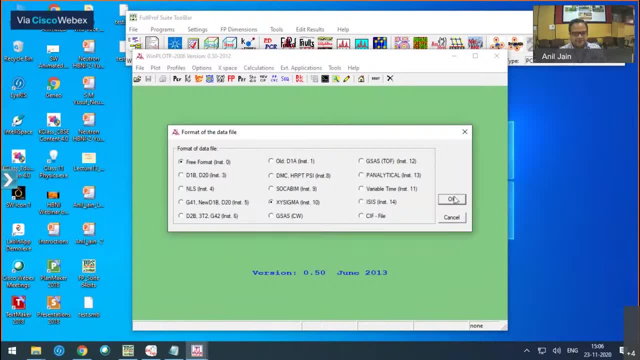 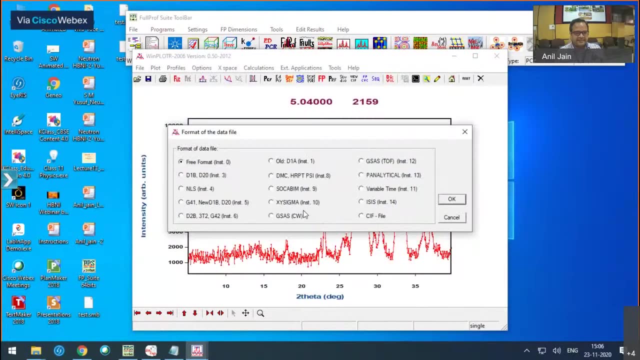 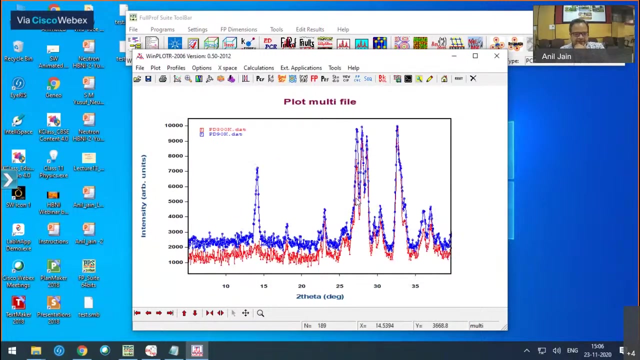 So I am showing only the data of limited range to avoid the competition, to make it easy for you to get it. get it. So this is at 90 k. So you can see clearly, at 90 k we have some peak enhancement in the intensity and last time, in the last lecture, we determined this magnetic structure. 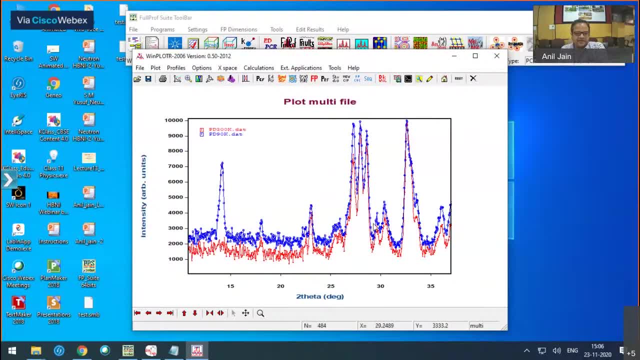 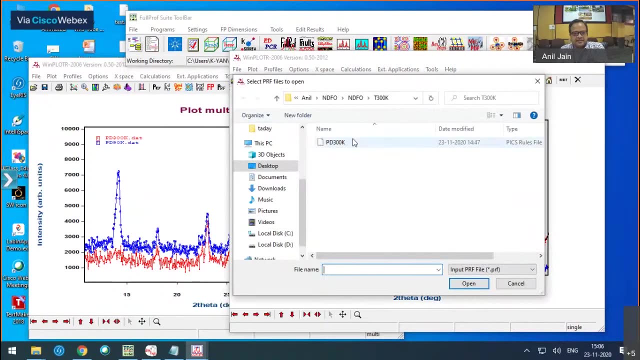 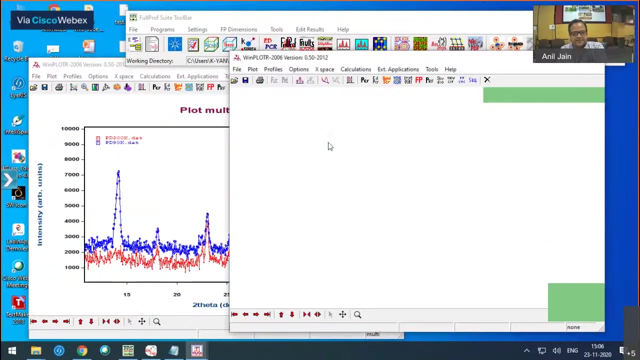 and you can see these positions are the same as like a big reflection of your nuclear peak. So I can open here another tab and try to plot here this PRF file of this 300 k. So let me reset it: PRF 300 k. So the 5 k is by mistake here. 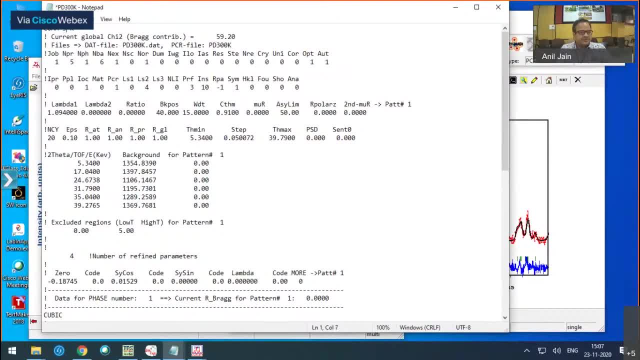 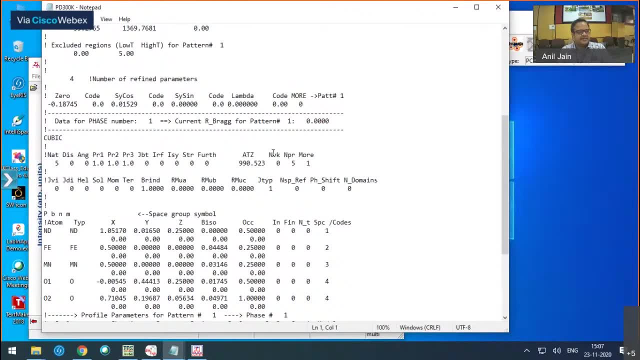 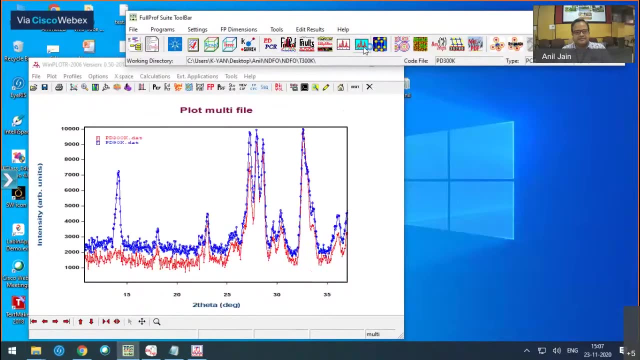 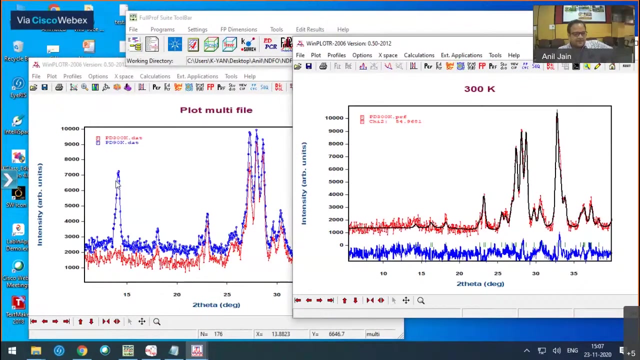 Uh, let me correct this. This is comment due to comment a. So this is the data at 300 k and let me quickly run it. Okay, So this is the refinement at 300 k. Now you see this blue lines or blue curve. here is the data at 90 k. 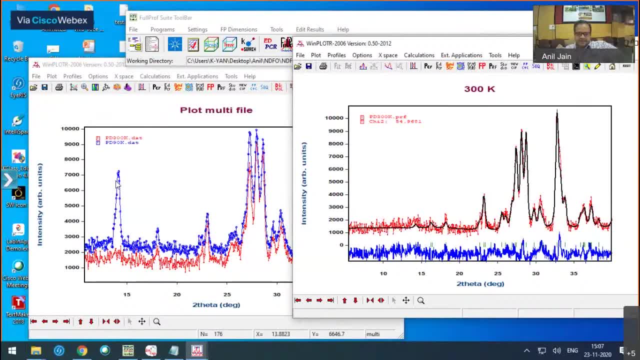 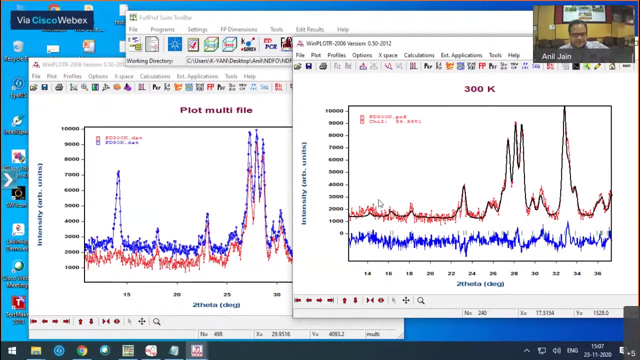 So it is clear that we have the additional magnetic scattering at 90 K and now idea is to determine the magnetic structure. So first of all, you can see this peak where we have an enhancement in the intensity, They are at the same location where we have this nuclear backpeaks. So you can see it here. the 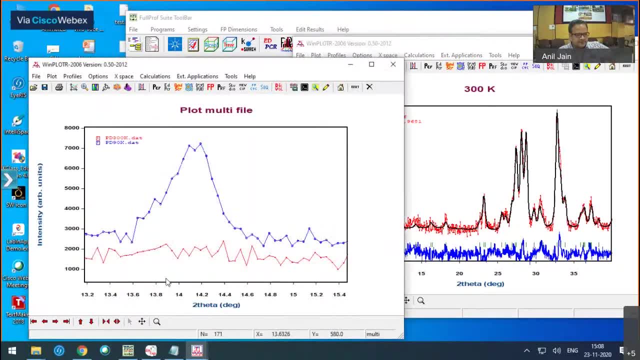 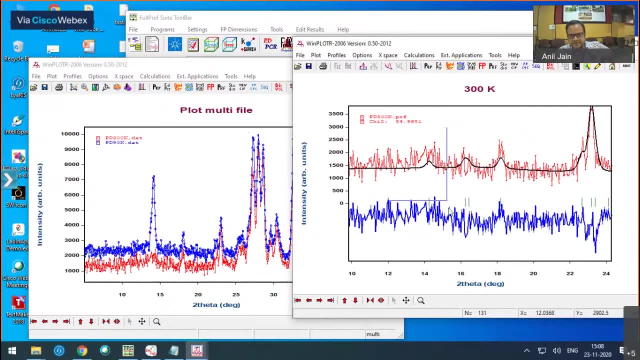 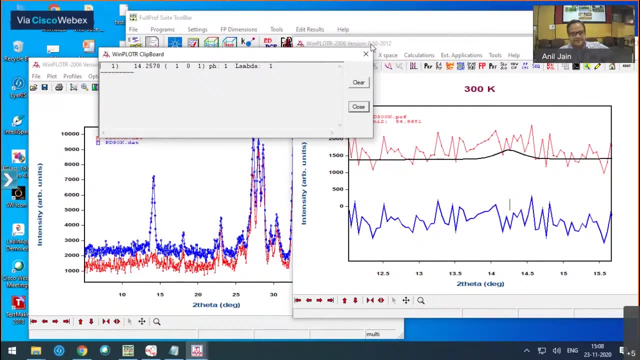 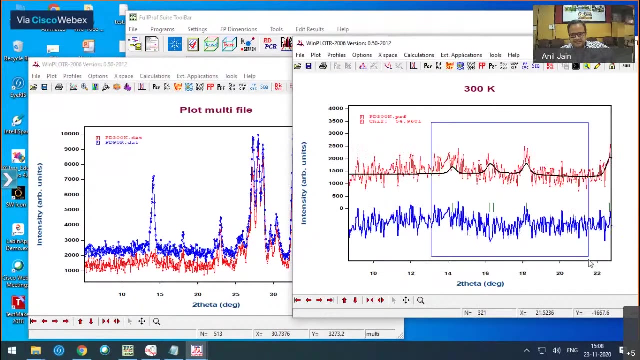 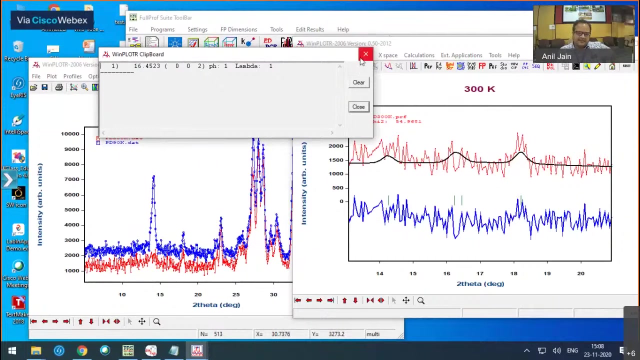 first reflection comes around something like 14.1, and you can see here if i zoom it. yes, so this is the position. this is nuclear allowed reflections, 14.2578. second, we have minor increase in the intensity here, and these are also nuclear allowed reflection. one can easily then say that the propagation vector for the ordering is zero. 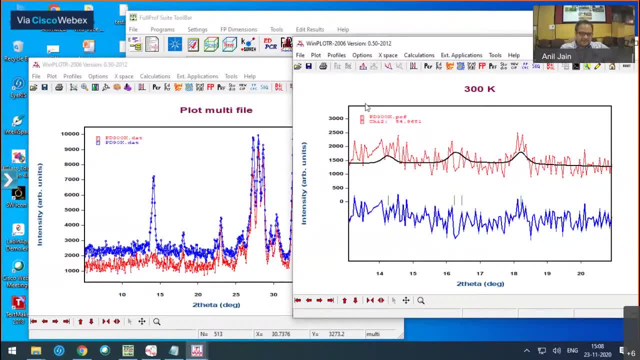 zero, zero. now our idea is: we know that two things: we know that we have some additional magnetic scattering and we know the propagation vector for the magnetic phase or for the magnetic structure which we plan to determine is zero, zero, zero. now the idea is to do this representation analysis and try to find out the 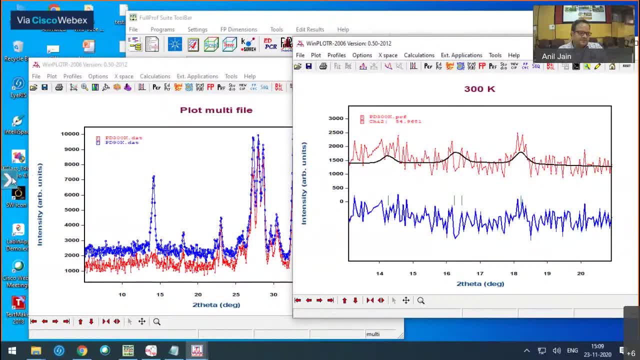 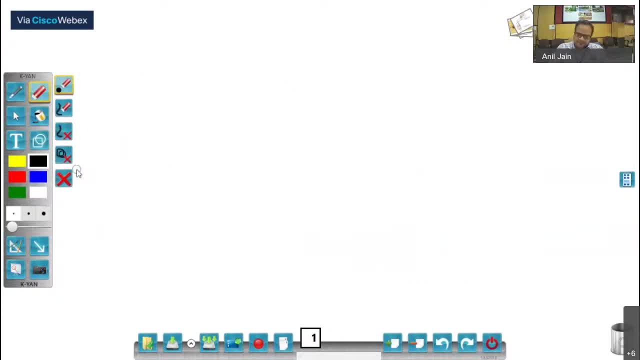 magnetic structure and you know, this magnetic moment, as i defined in the last lecture, is given by magnetic moment. m is given by sum over k and as kj exponential to iota- sorry, iota- q dot r. so this is the expression of our magnetic moment and what we have to determine is: 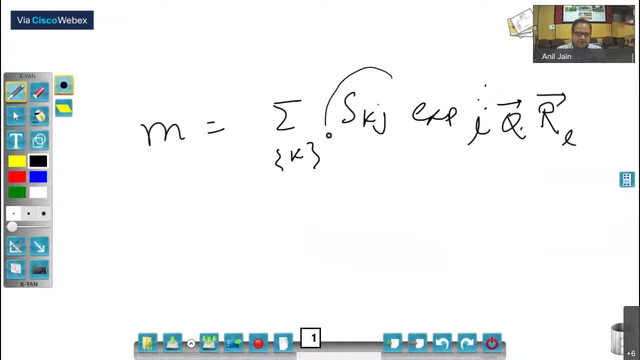 this. we have to determine the magnetic moment. and what we have to determine is this: we have to determine this Fourier coefficient, and this Fourier coefficient can be written as summation of this basis vector. so then, these are this coefficient and these are this basis vectors. so, this basis vector. 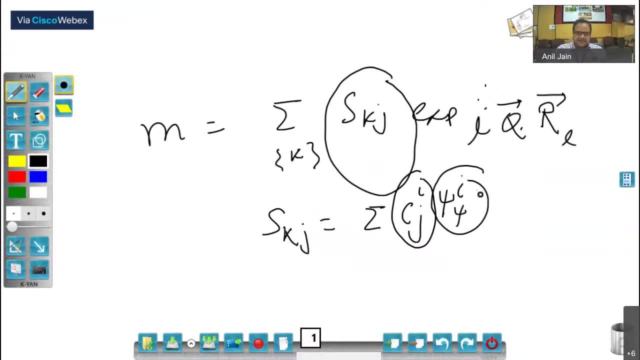 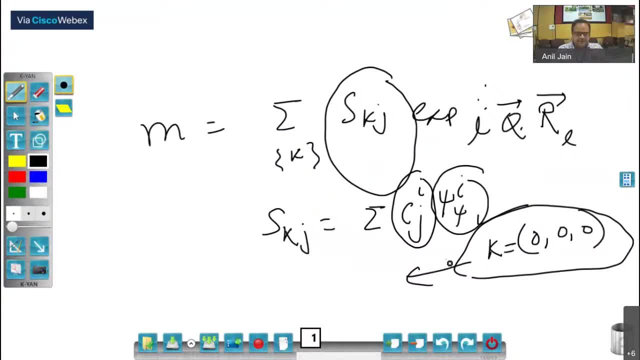 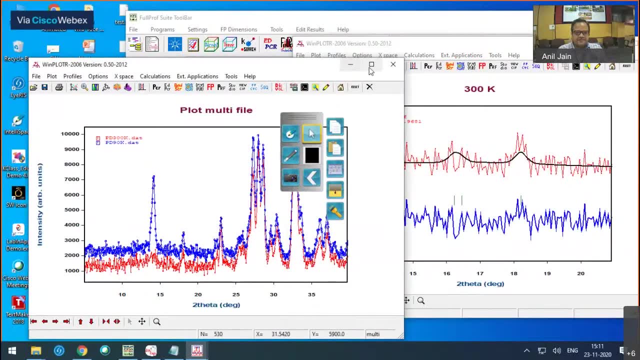 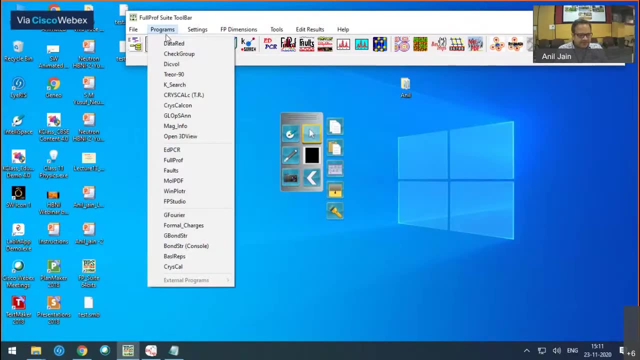 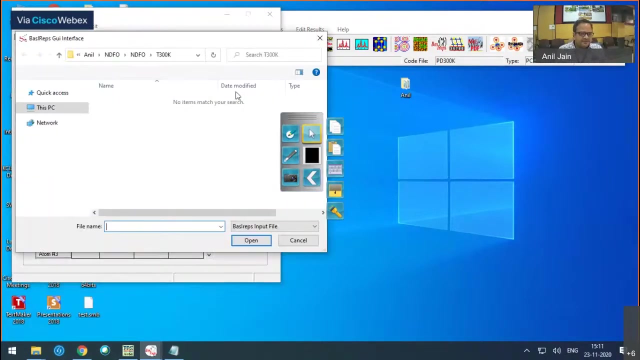 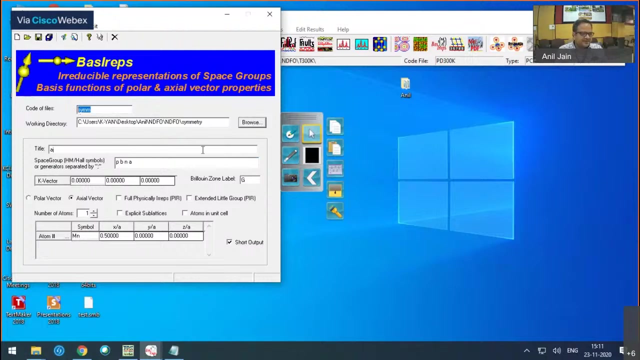 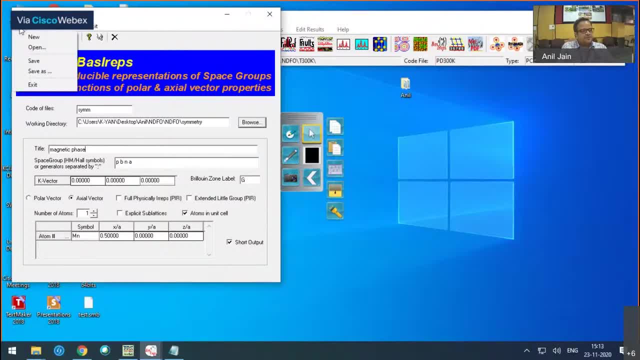 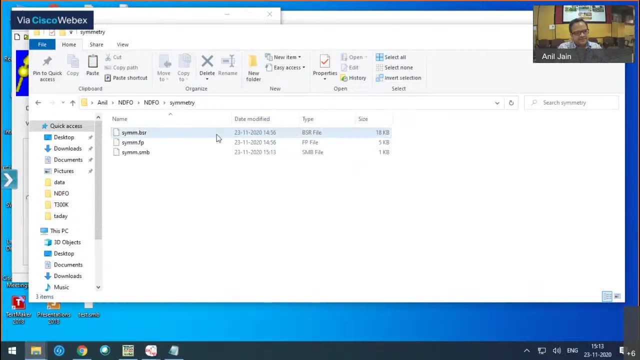 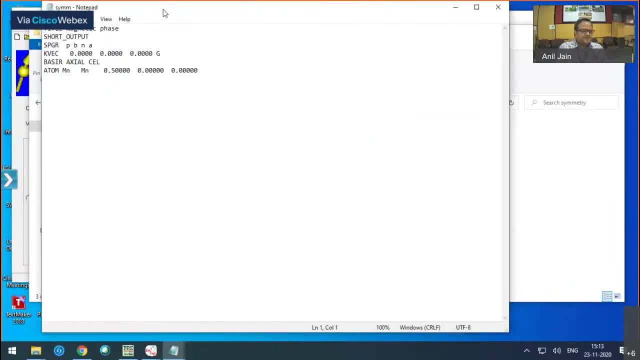 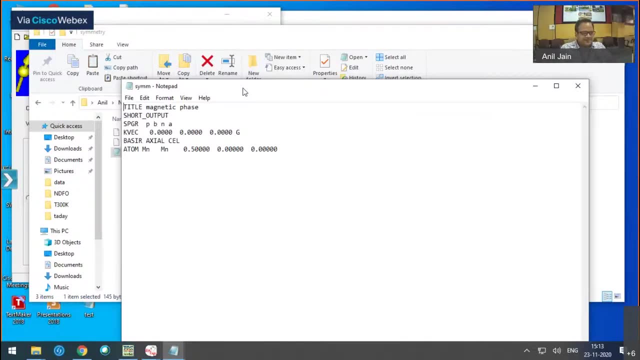 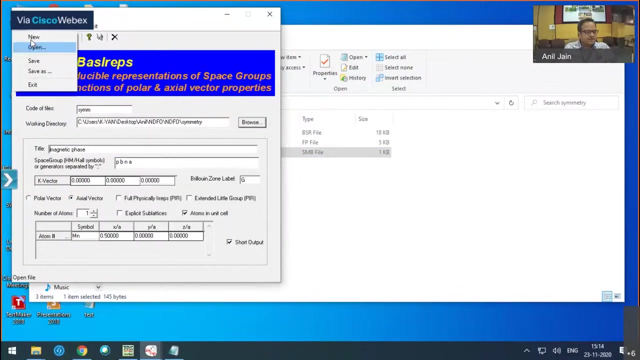 Let us see. So if you want to run this base reps by this GUI interface, you can run that also. So this file: first is title: Short output I have set. I can set this long output also: Space group is PBNA K, vector is 0, 0, 0.. And this I have, This is gamma point And this is our item. Axial is the moment And half: 0, 0.. And now let me close this And I go here. File open: Now let us ask it to run. 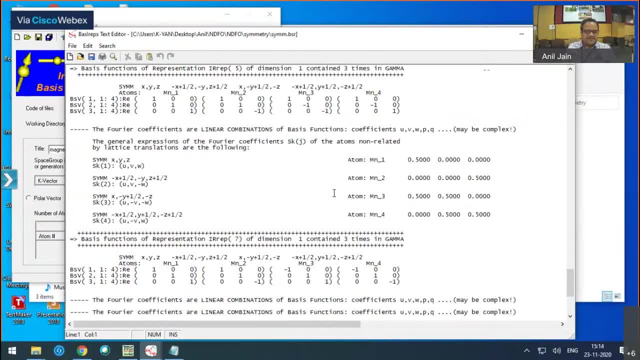 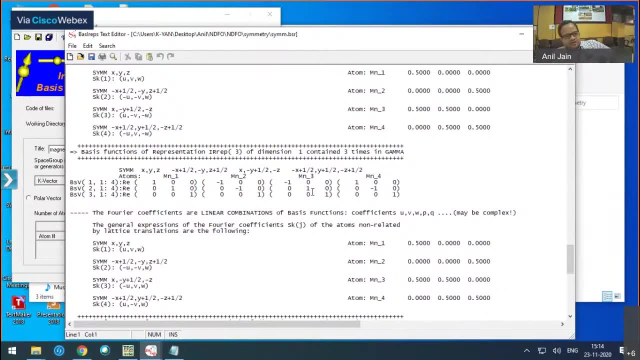 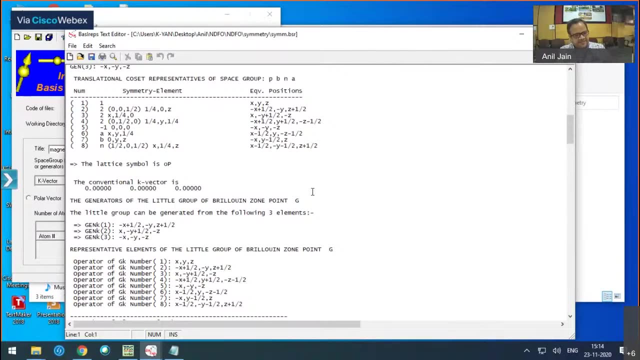 It does this Symmetry analysis And it produces a file. I will advise each of you to at least go through this file and try to understand the meaning of this, different things which are mentioned in this file. Of course it is a long file, But I think once you should go through this. 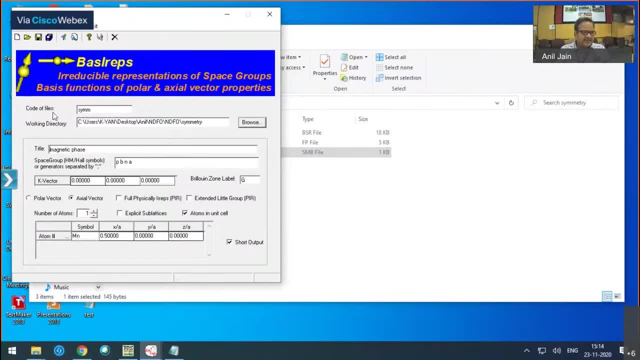 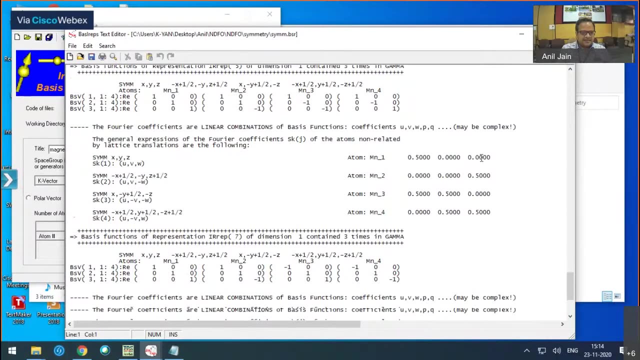 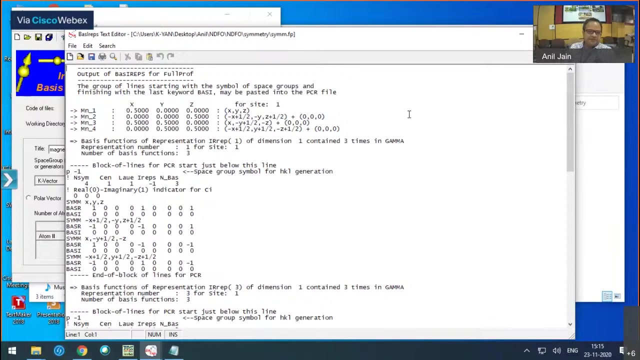 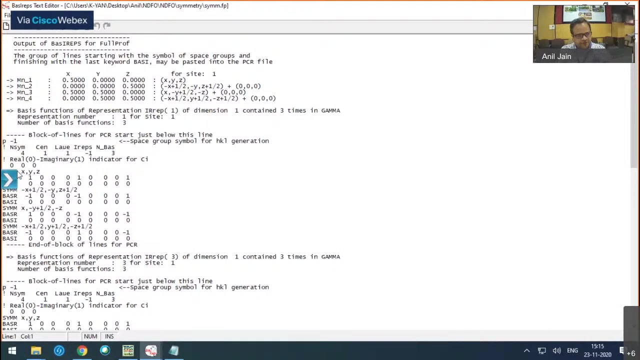 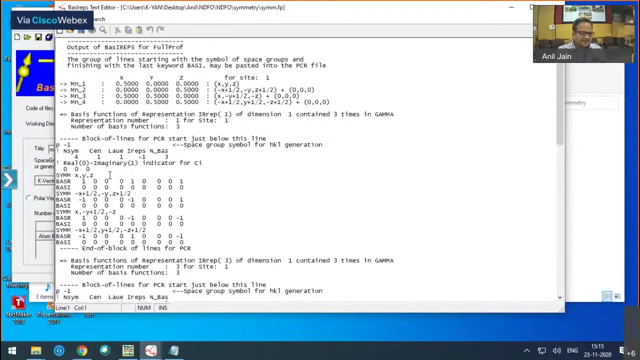 So now, once I run this file by base reps, it is going to generate two files So I can go in the result. So one is the BSR files And other is the FP file. So in the FP file this program does a lot of job for you, So it tells you if you want to put or if you want to make your PCR file with this basis vectors. So these are the basis vectors now. 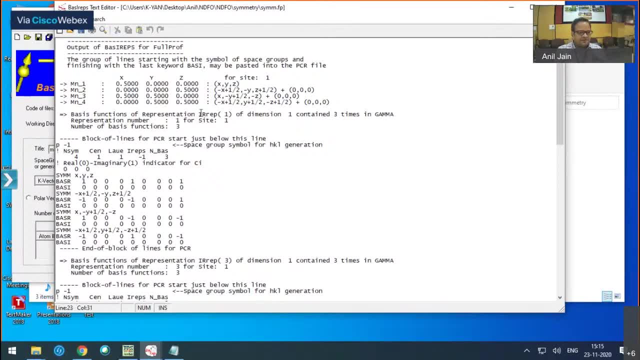 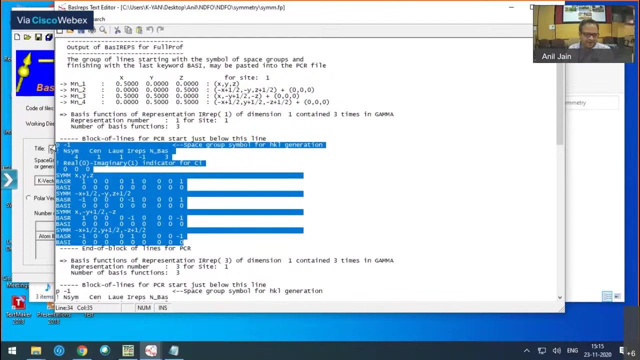 It was it does. So it write. So it write. the basis function of representation, number one, of dimension one contain three times in gamma, So it write. So these are three basis vectors. This program has given this basis vectors for you. Only what you have to do is you have to copy and paste in a PCR file which is compatible with taking with this moment value. 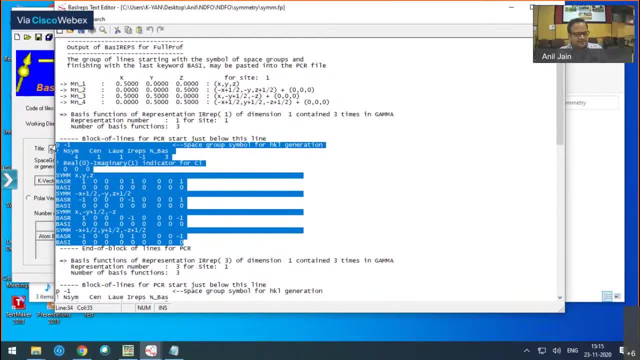 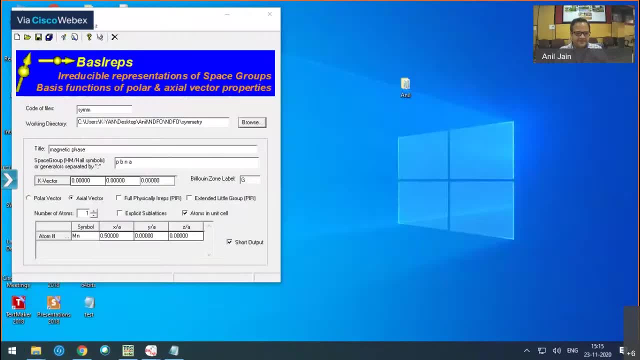 Taking with this notation in the terms of basic parameters, Using net Notation Notation, Notation in the terms of basic parameters. So what we do is now. I show you. so what generally we do in this case is we go to the 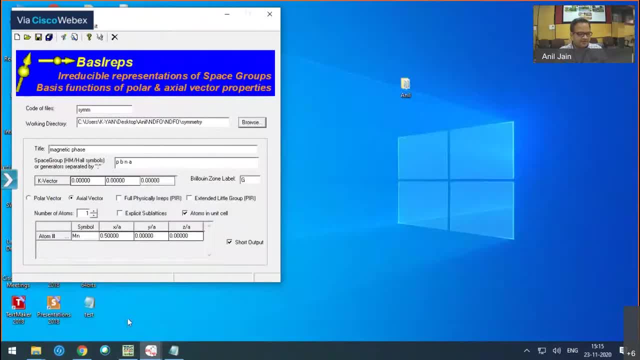 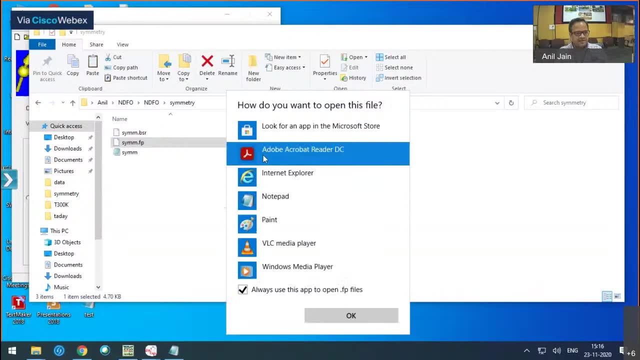 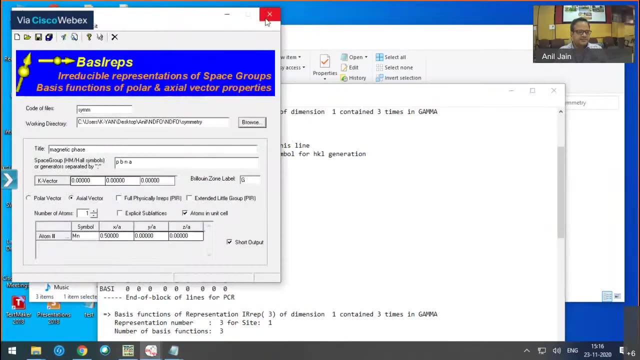 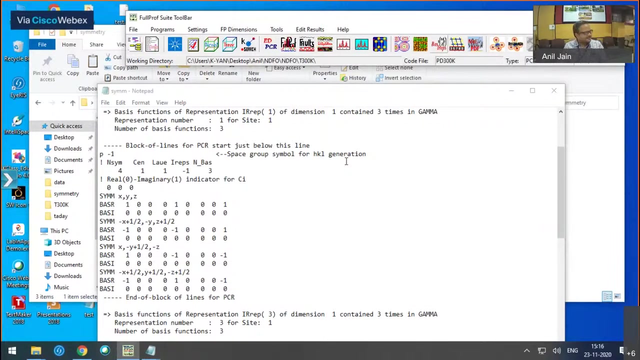 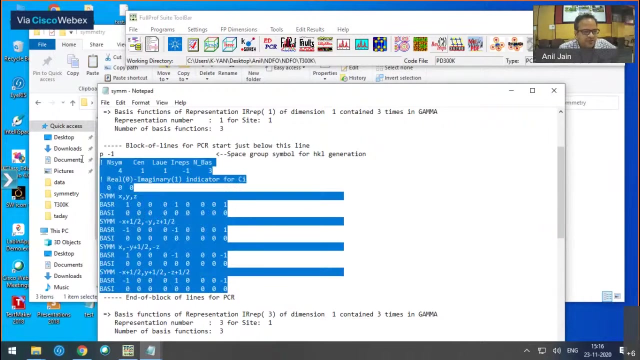 so we close this and I keep this file open, which is generated as a fp file in the notepad. Now I can close this file. Now, what we do after this is: let me close this. So we have done this representation analysis. now we would like to see this magnetic structure. 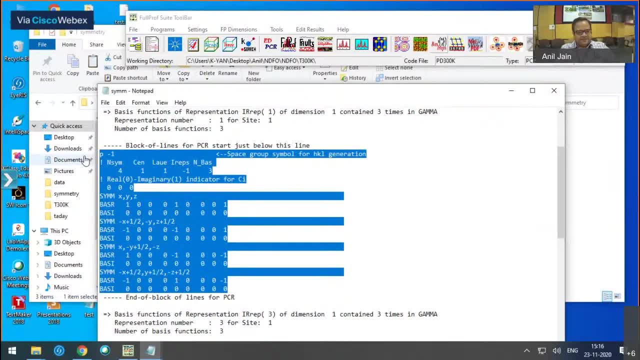 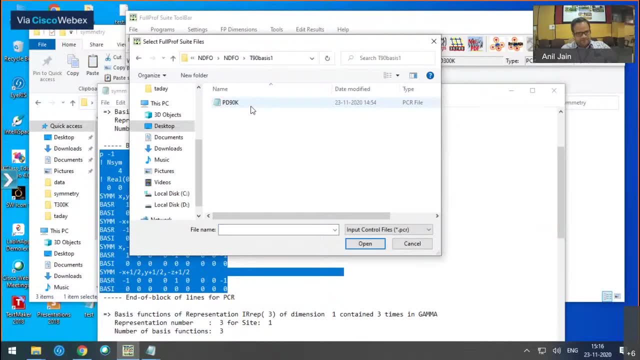 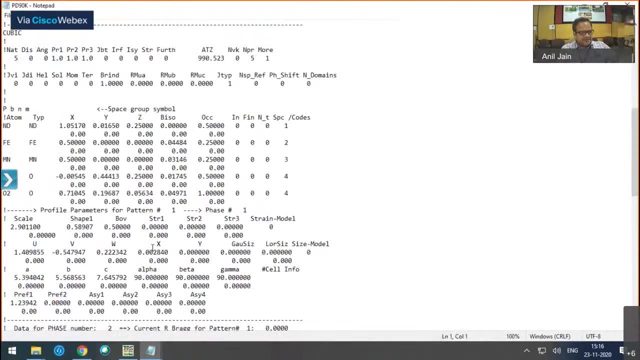 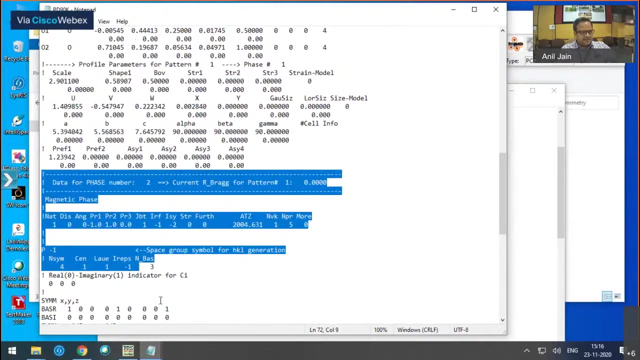 corresponding to this symmetry operation. So what we do in the PCR is then. so let me show you. I go to this PCR here I have already added a magnetic paste, But how it is done is that So if you see our nuclear phase file, so nuclear phase file generally have content. 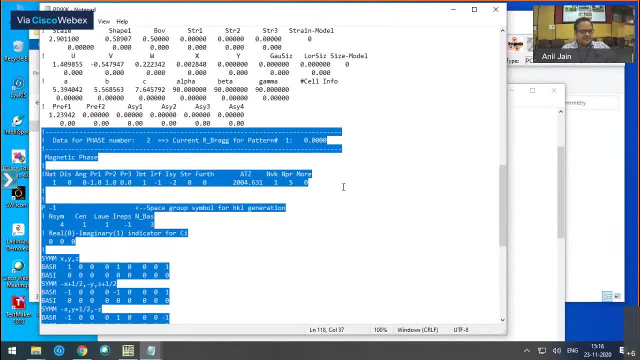 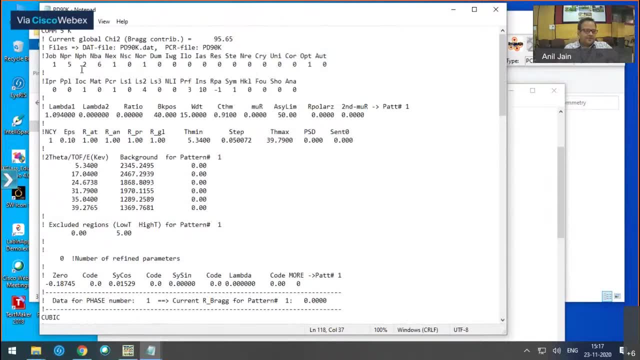 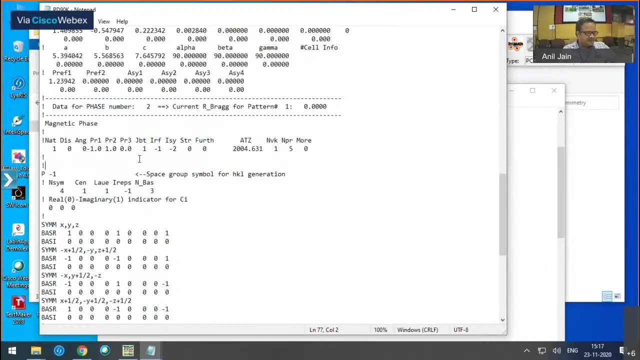 all content other than this highlighted one. So in the last line where it comes here, I have inserted this phase, and I have to put here number of phases too. Then what are the different symbols here telling me is that this irf equal to minus 1, and? 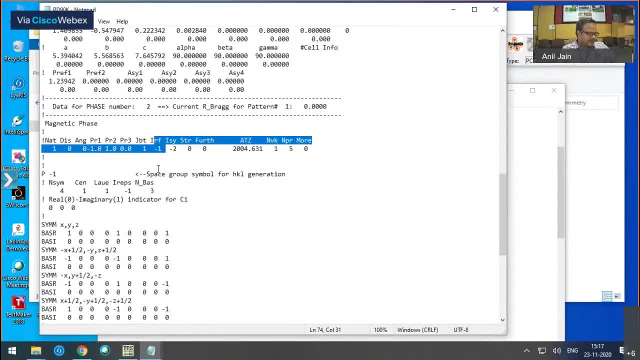 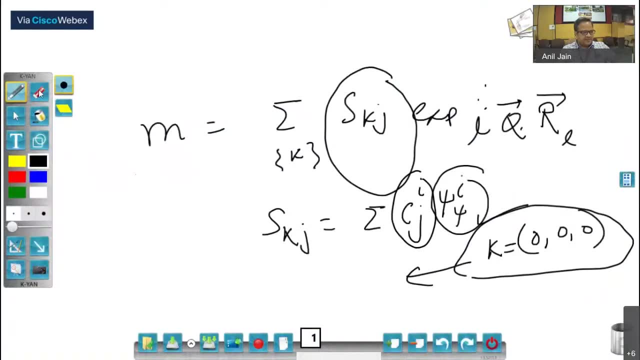 rito, Everyday is telling me, is that only satellite reflections for the magnetic contribution? let me not it down. So what is the meaning of this different symbol in the magnetic face? So we have magnetic phase, So irf equal to zero. 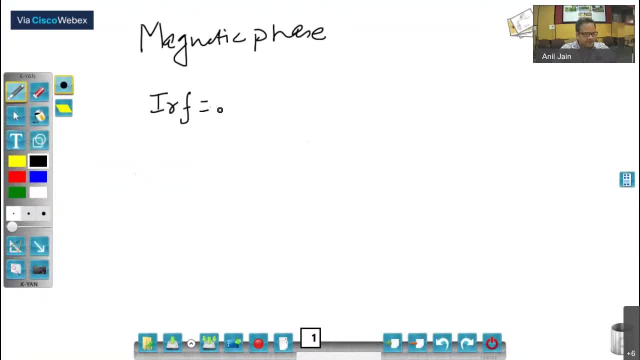 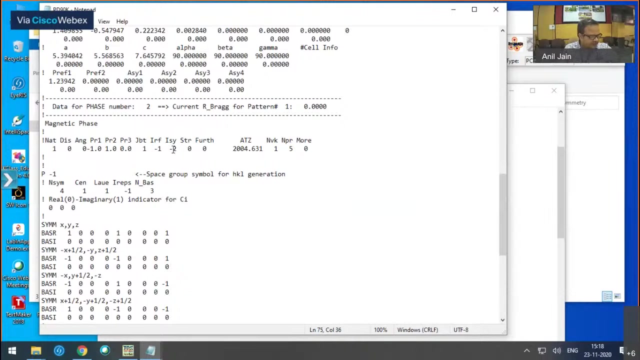 Okay, So the yeah, magnetic phase Rf equal to minus 1 means only satellite reflection for the magnetic contribution For magnetic And there are couple of more important things here. I Sy equal to minus 2 tells me that in this PCR file. 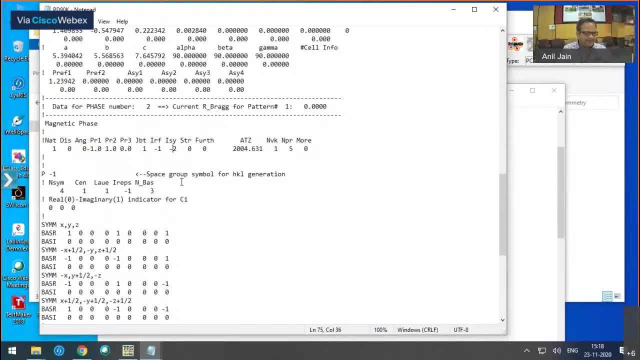 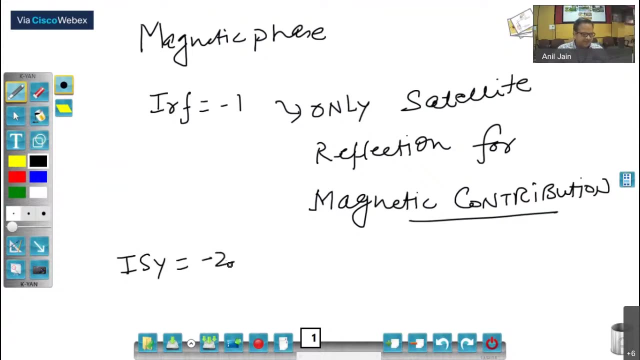 I will be giving the information about the moments in terms of the basis vector. So I Sy equal to minus 2, it means component of magnetic moment in terms of basis vectors. So this is what I am telling. if I am putting I Sy equal to. 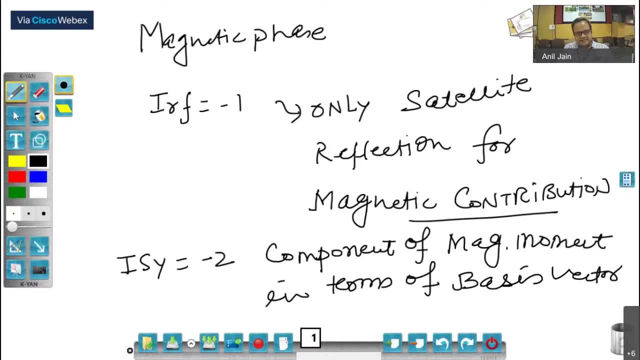 minus 2.. Instead of this, like what we did in the last example, we used I Sy equal to minus 1.. So if I use, I Sy equal to minus 1.. So if I use, I Sy equal to minus 1.. 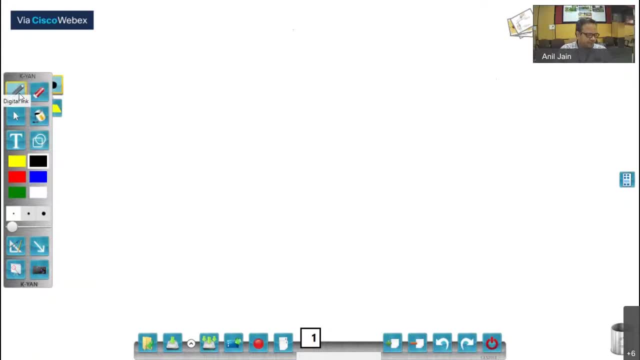 So if I use I, Sy equal to minus 1.. So if I Keyboard I- I, it means I will give this information about this moment in terms of this symmetry operation, that I will write something like magnetic symmetry Sy equal to minus 2, and something I will about it. So I will not give this basis vector. 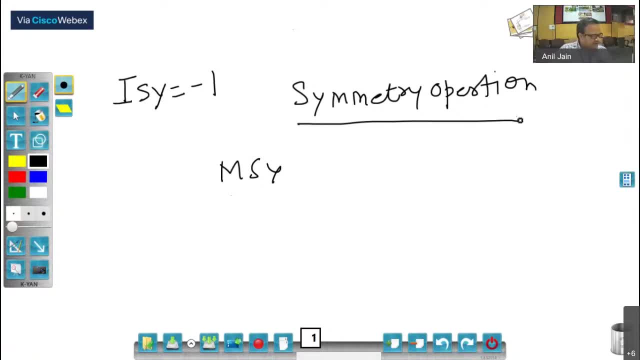 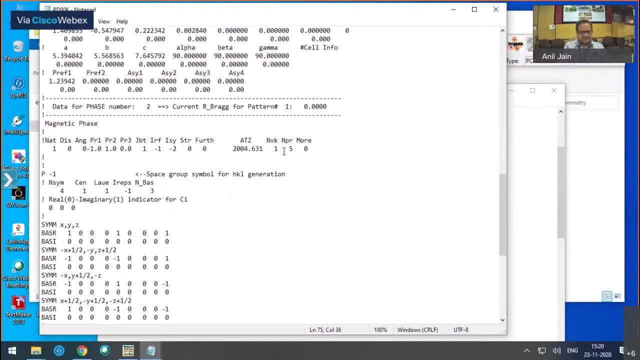 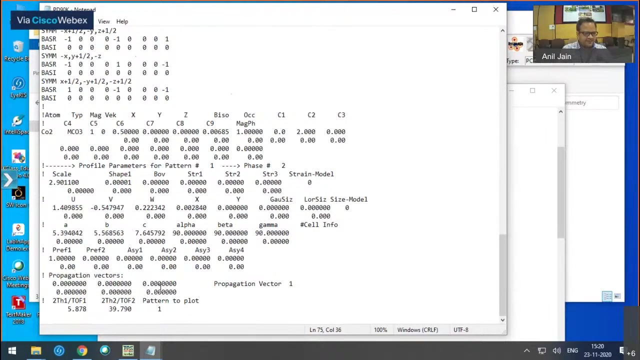 But I will give this symmetric instructions in the pcr file. and there is one more piece of important thing here in this pcr file is nvk. so this nvk is telling us this number of propagation vector here, and what we have is only one propagation vector, which is 000. 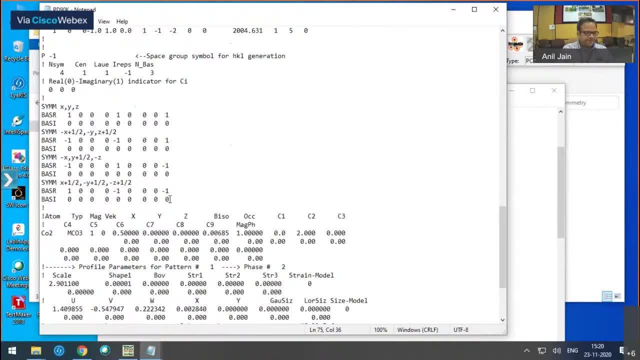 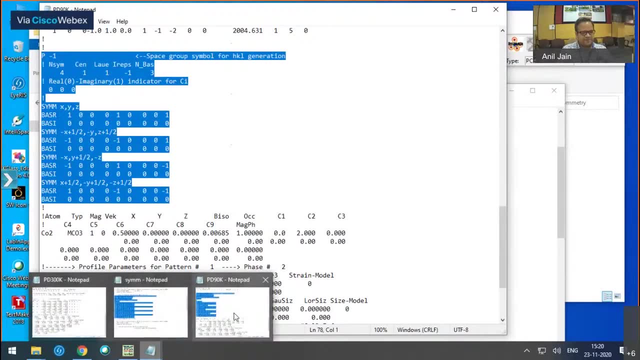 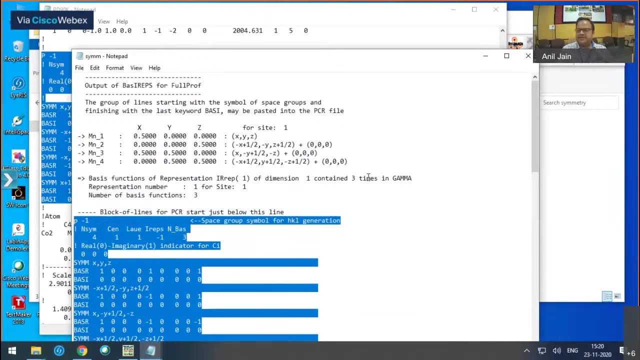 and then this information, this: when you run this basereps code, it comes from this basereps program. so let me show you. so this is the output of our symmetry operation. so iron and manganese goes to the same site and we have a four position in our space group of this. 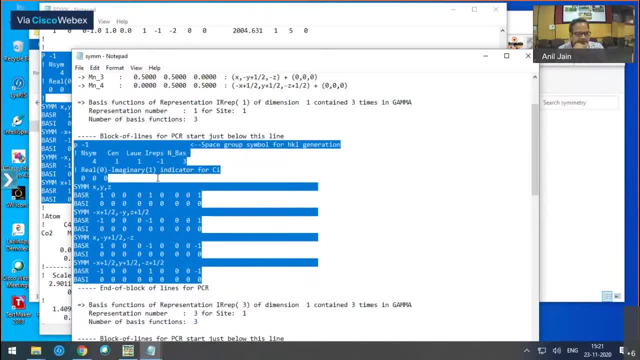 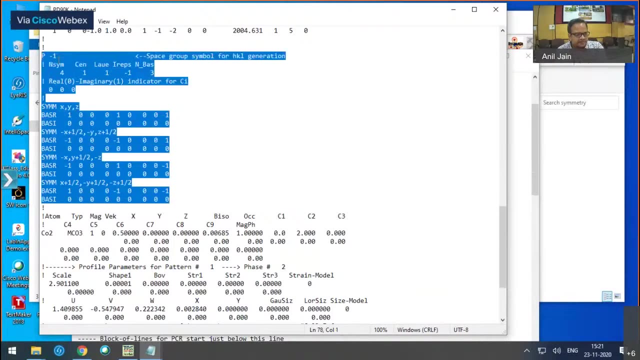 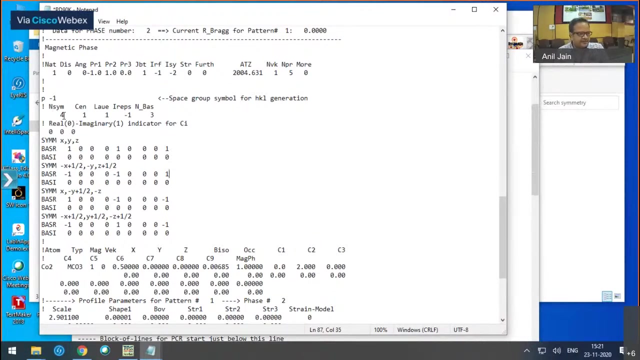 site. Now this is the block of the pcr file which directly I can copy it and I can directly paste it here Now what it is telling is that we have four symmetry operation: one, two, three, four. this is the information about the lovin. 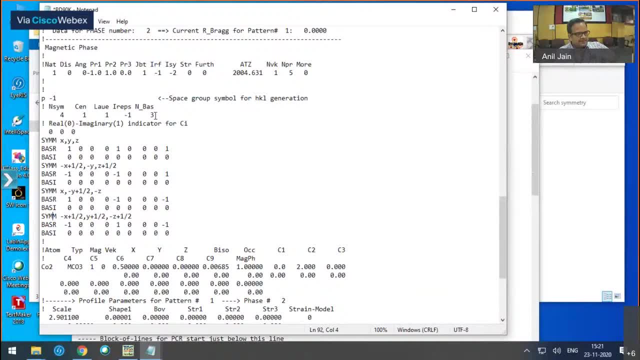 So we have three class and n base. 3 is telling me that I have three basis vector. so it means I will need here at least three coefficient for this magnetic structure and magnetic moment will be given by this. so, like for this site xyz, magnetic moment will be. let me write down: 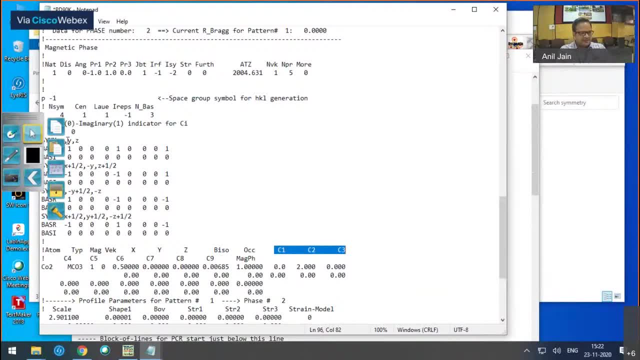 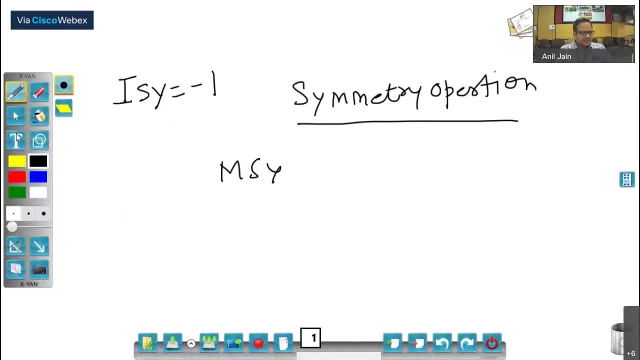 explicitly So, the, So the. So the basis vector is 100, 010 and 001, so magnetic moment in general condition can be written as the Fourier coefficient of the magnetic moment and they are directly moment in this case, because k equal to 000.. 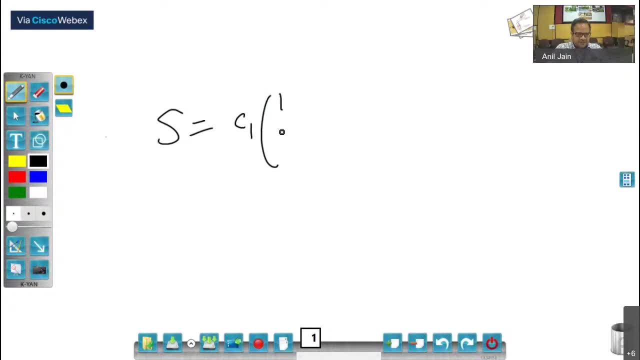 So this will be like c1 1 0.. So this is the basis vector. So we have c1 1 0 0, c2 0 1 0 plus c3 0 0, 1.. So this will be our moment. 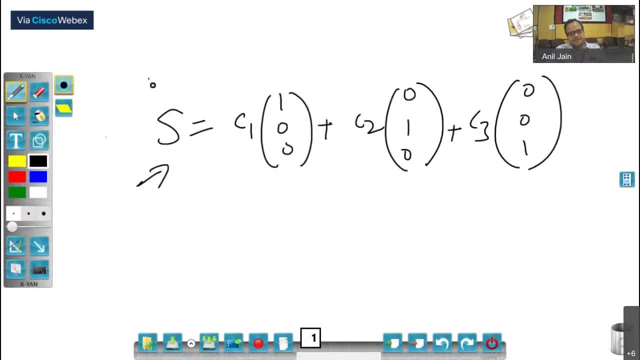 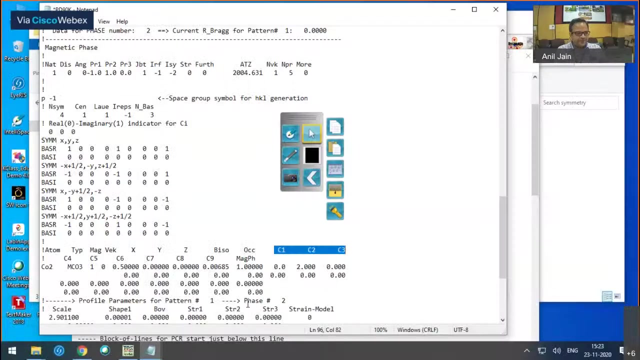 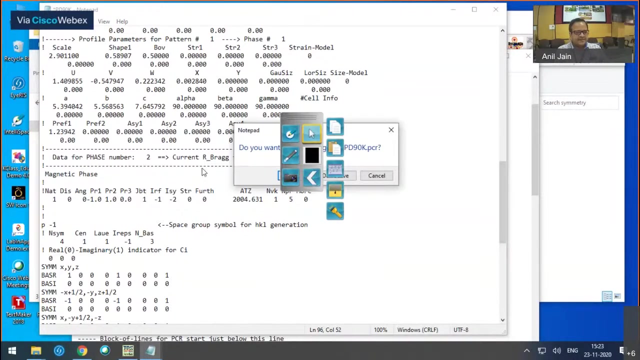 So our idea is to determine this c1, c2 and c3.. So we want to get this information about this three coefficient, So to determine the magnetic structure of this compound. so let's go to the full crop now and let me close it and let me show you how it looks like in the editor. i say save. 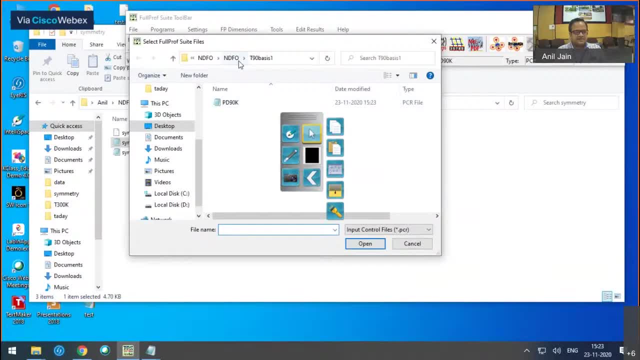 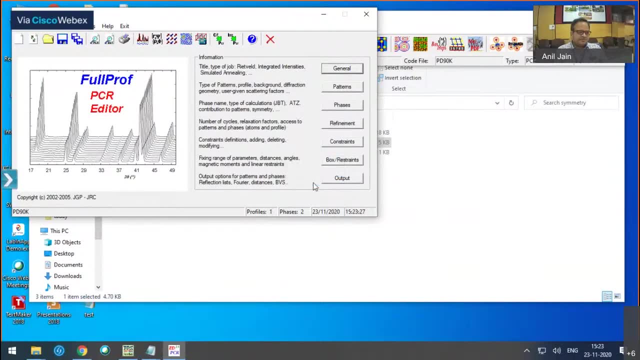 and i say to this that this was the file. i was working at 90k and i go to edit pcr so those who are using it first time, they can use this edit pcr. and if you can open this file in this edit pcr, it means your file is more or less correct. otherwise, 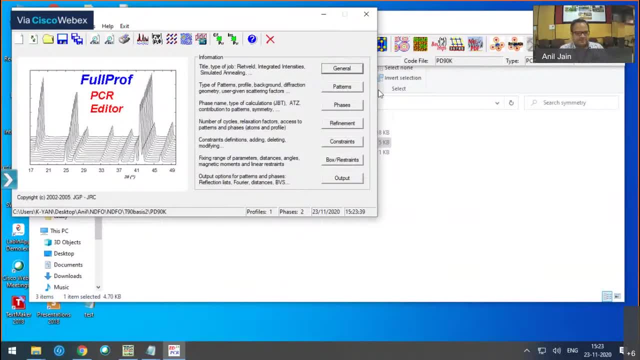 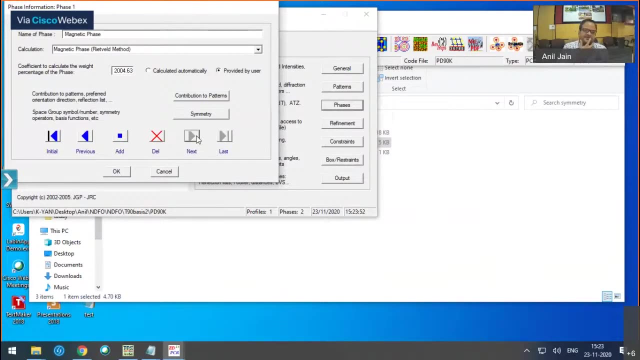 this edit pcr will give you some error. now i will directly like to go to this pattern. we have only one pattern and what we have is two phases. one is this structural model and other is the magnetic phase, and you can enter here in the magnetic phase. 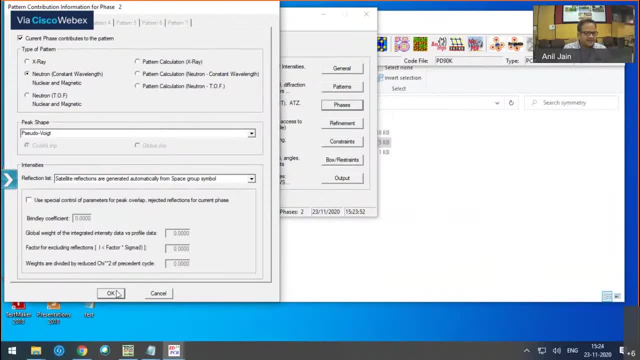 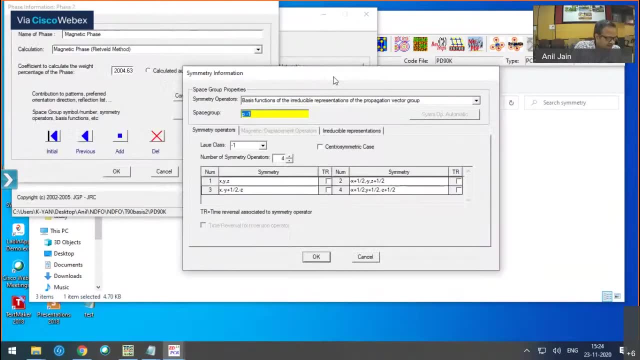 that this is the with the constant wavelength, and we have to go, importantly, in the symmetry. so you can see here that i have put i as y equal to minus 2, means due to which it is coming. that basis function of the irreducible representation of the 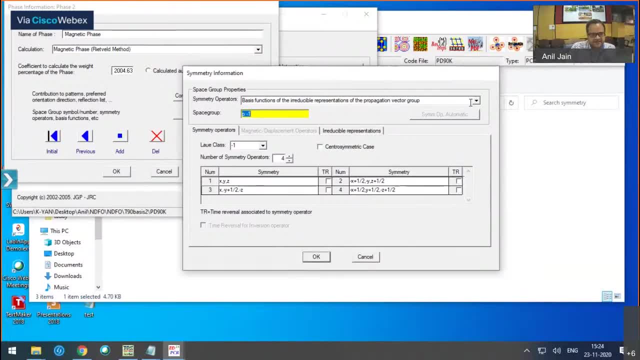 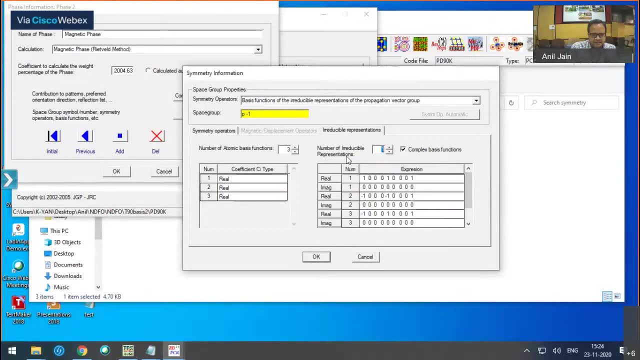 propagation vector group. so what i will be giving here is the. i will be giving the information about the basis vectors and these are the basis vectors. so this is imaginary part, real part, and this basis vector is three component and these three components are along the direction of your 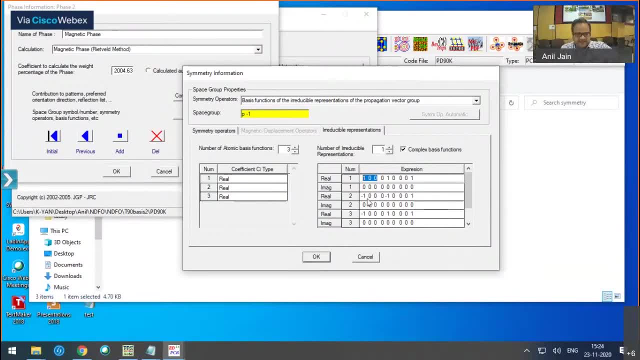 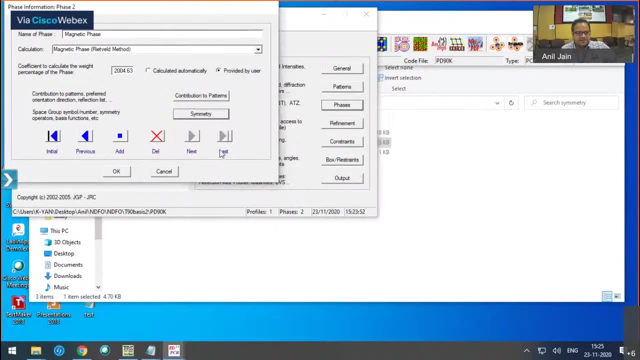 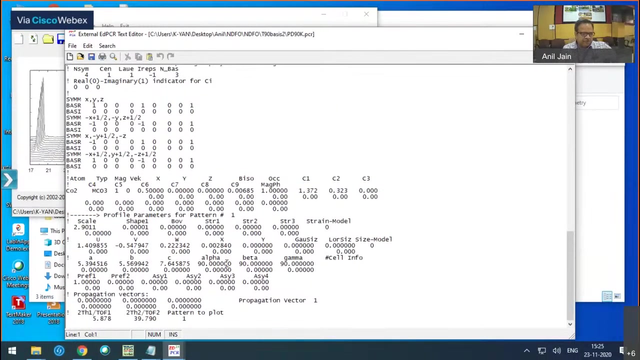 crystallographic unit cell in the real space. so these, so c1 of this plus c2 of this, plus c3 of this we plan to determine, and these are the coefficient which is written here. okay, let me save it and see it whether now a very quick way to do it. 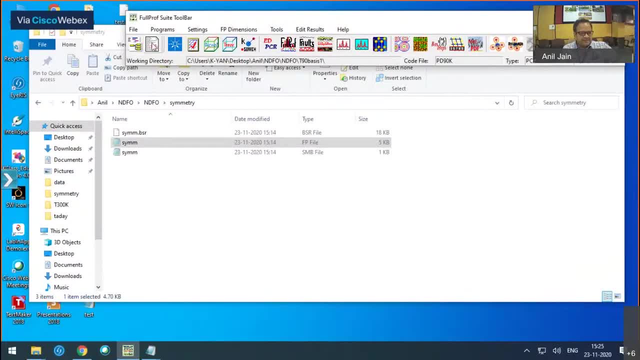 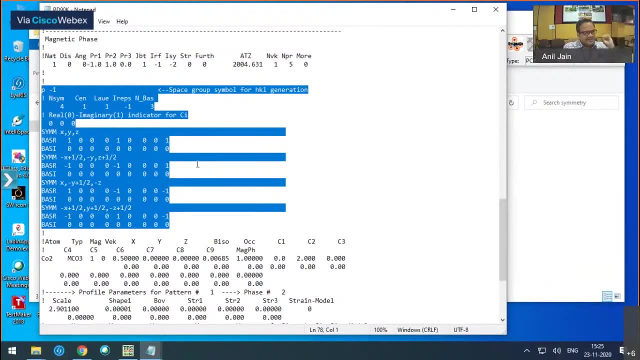 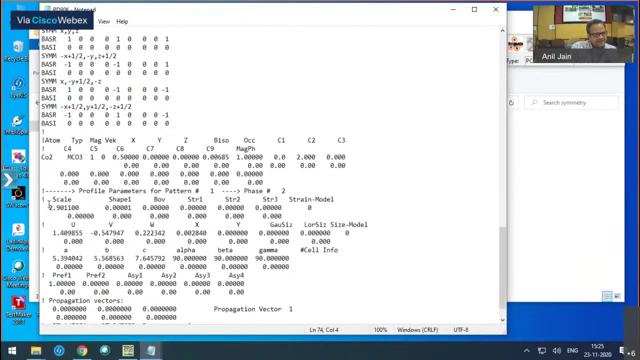 is like this: you have added this additional phase, basically. so now you are going to forbidden not very interesting work, because i mean so as itإs very difficult, so as it is Resistance an onnant, to make difference would be like of using for series variable. so you can definitely. use. uh, you can see here that you can now use the. we have a curly line. give it a to vthe i, which you can do that if you want, so that you have added the die questo, which is a non protrusive. again, again, one of the hidden. 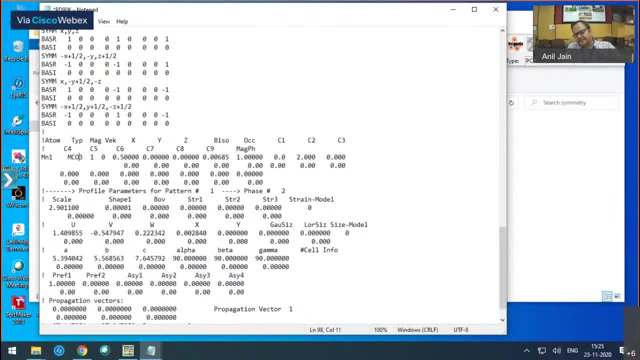 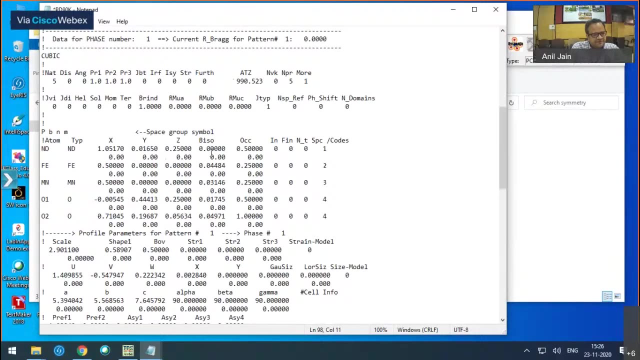 minimums of the on, going to the non protrusive random string that we are. the atom is magnetic. I write mn- n3 means mn3 plus and this half zero. zero is the position which is given here and this side. when we write in the magnetic phase, it is fully occupied. 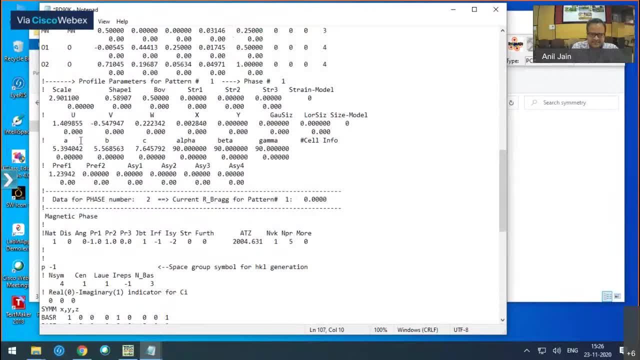 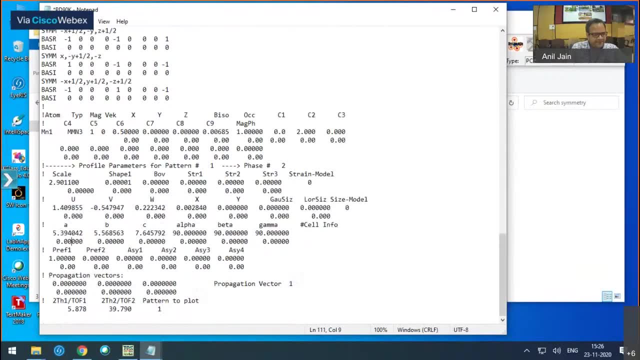 Now this parameters UVW in the starting. you can keep it as same as is there in the nuclear phase abc also you can keep it same preferred orientation, preferred to, and this all four asymmetry parameter. you can keep it one, zero, zero, zero, zero, zero if you are dealing it. 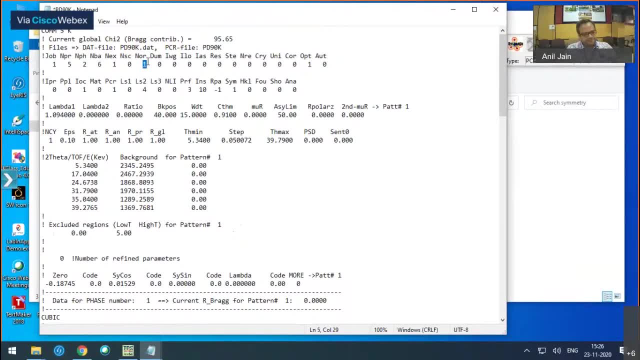 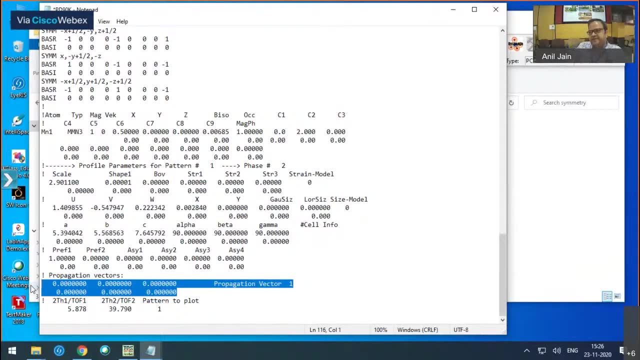 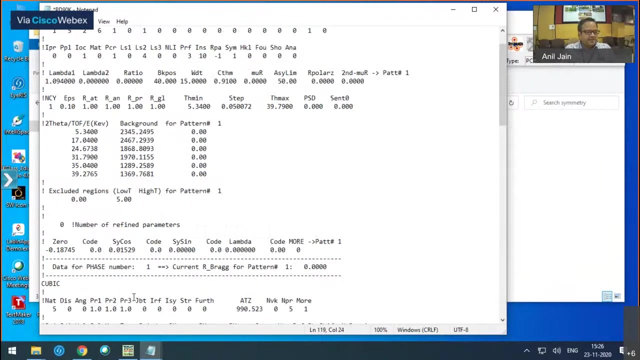 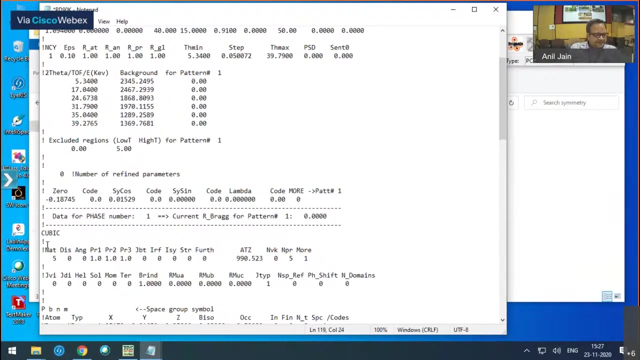 here with n or equal to one. This is the information about your propagation vector, and we have only one propagation vector And this you know. This is the range by which you will see the refinement while running this PCR file. Now what generally looks better way to me is that I make it this number of refined parameter. 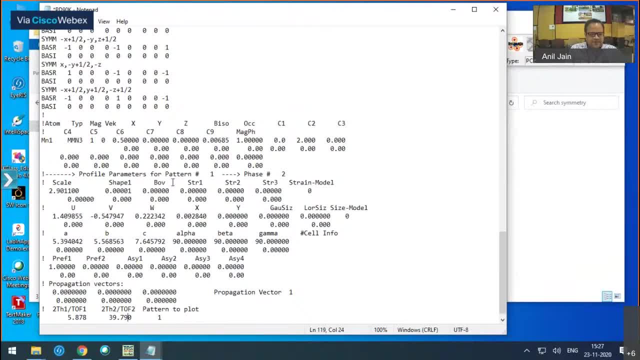 zero and I just try to see it what kind of magnetic intensity I get it by playing with this parameter. So let me put, let me put some parameter like One which looks like reasonable value of the moment for the C1 and let me just try to. 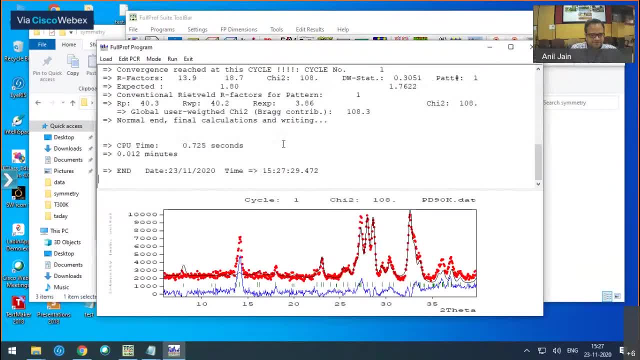 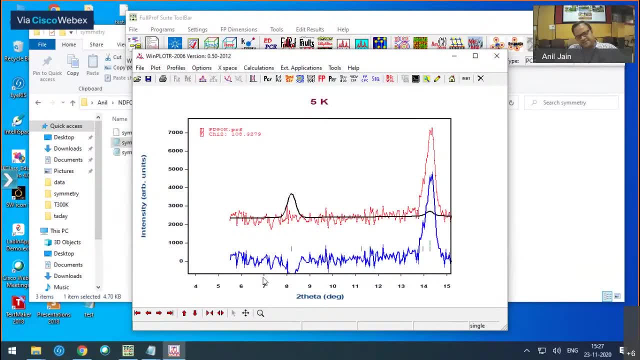 run it. You see it, if I, I can see it from here that if I put a, even a small moment of one, it tries to generate the intensity at this location where we have no magnetic intensity. So I can see it from here that if I put even a small moment of one, it tries to generate. 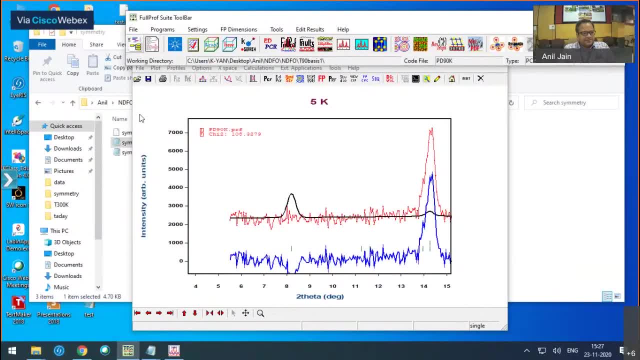 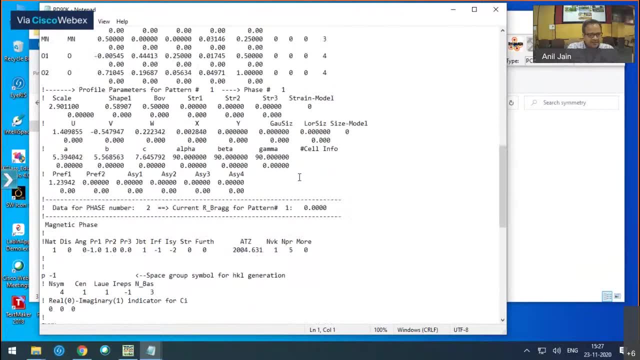 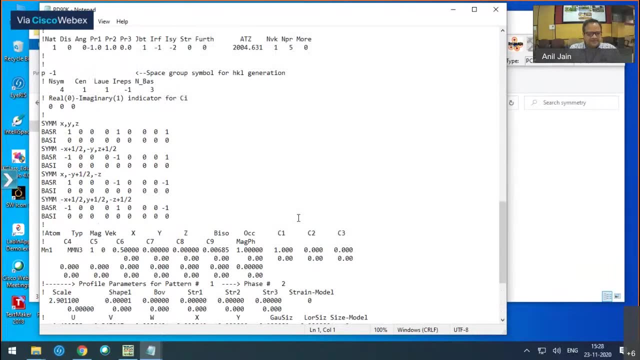 the intensity at this location Where we have no magnetic intensity. So it means This configuration is not good for the magnetic structure. So it means this configuration is not good for the magnetic structure. And now, if you have only C1 coefficient, it means what it is telling it that if I am writing, 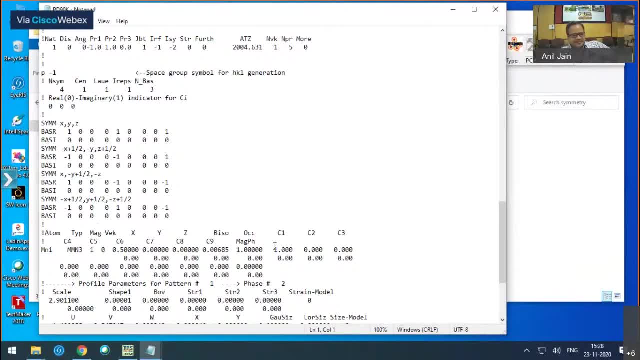 only C1 equal to one and C2 and C3 zero. it is telling me, by looking at this basis vectors, that my moment is aligned along only one. So that means, if I am writing only C1 equal to one and C2 and C3 zero, it is telling me 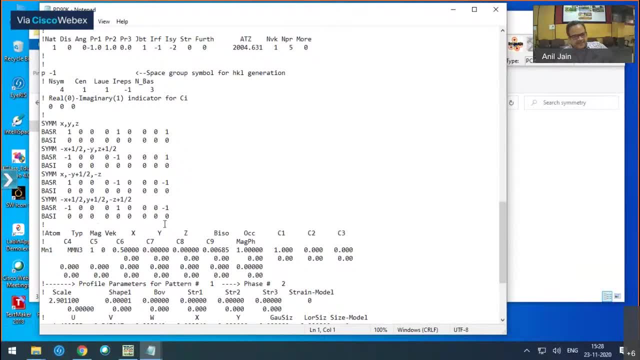 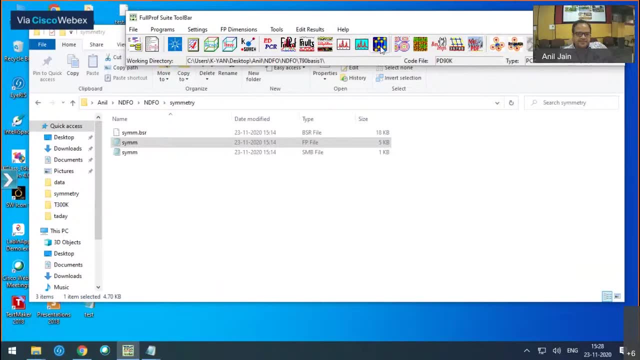 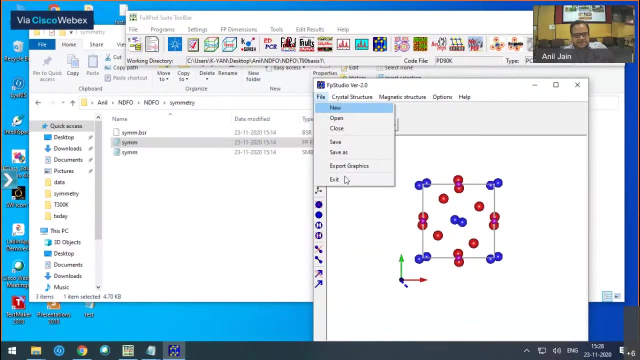 by looking at this basis vectors Along only crystallographic A axis. If you want to see the detail corresponding to this, then what one can do is one can close this, go in this studio and where we are- we are here in the T90 basis one. 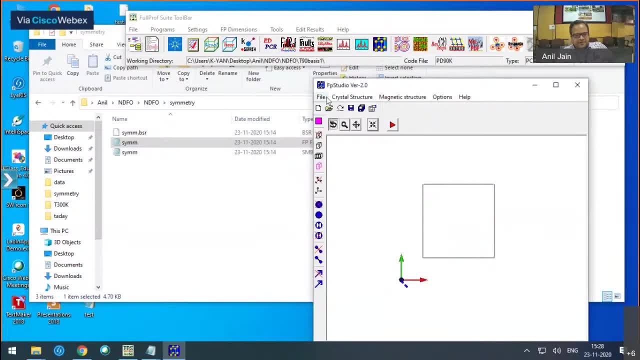 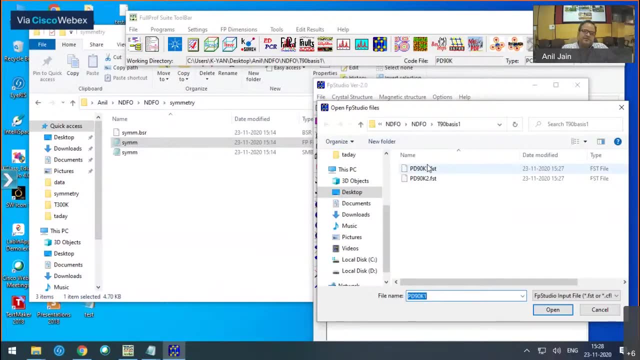 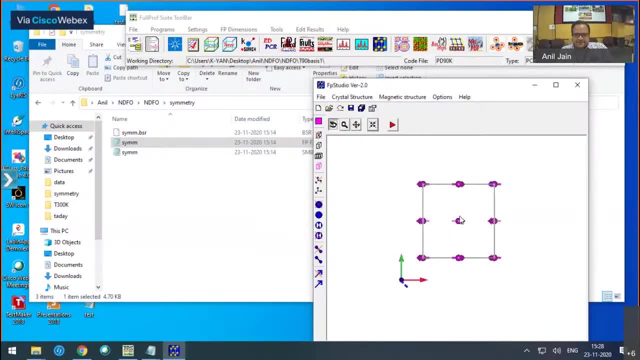 One is corresponding to the phase 90.. One is corresponding to the phase 90. One is corresponding to the phase 90. And the other is the corresponding to the magnetic phase. So let me see So with this representation, if my material ordered, then, as you can see, this is telling. 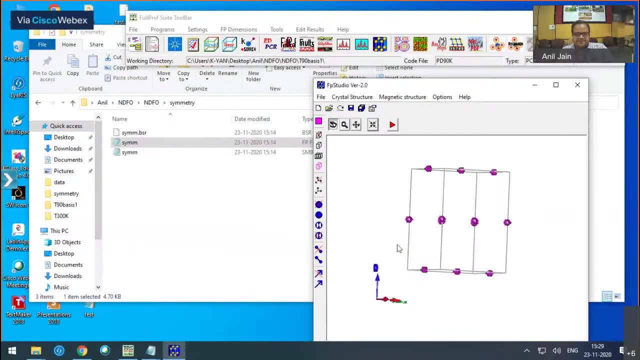 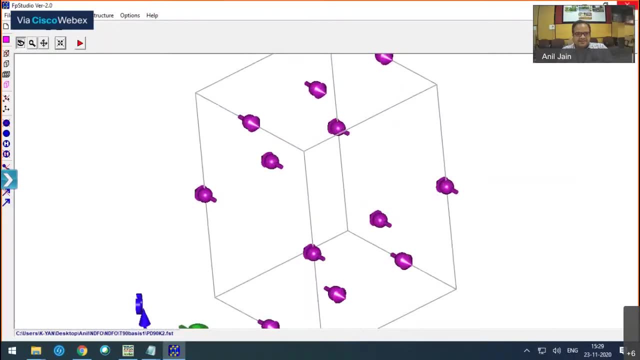 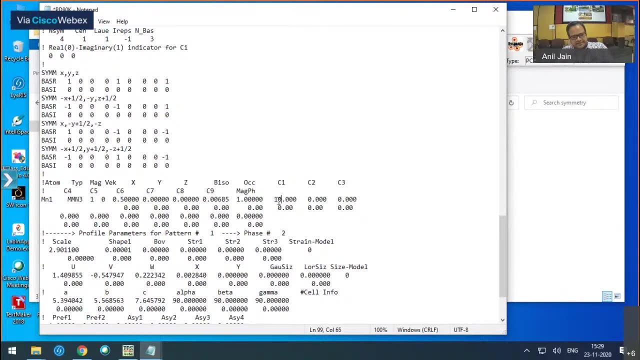 me that the direction of the moment is along the axis Right. Let me just try to play it with more. What I can do is simply to show it to you Now. this is the position of the magnet. Let me you that i make my c1 coefficient zero and i can make c2, now one. then let me see. 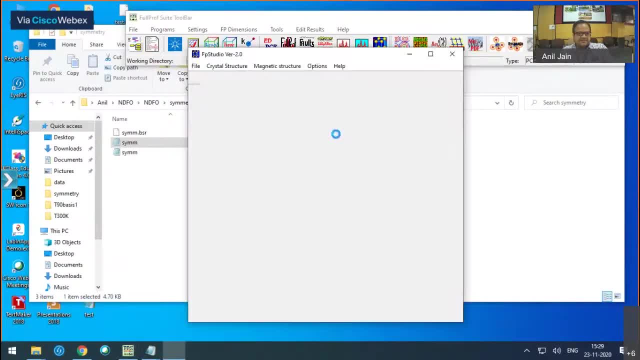 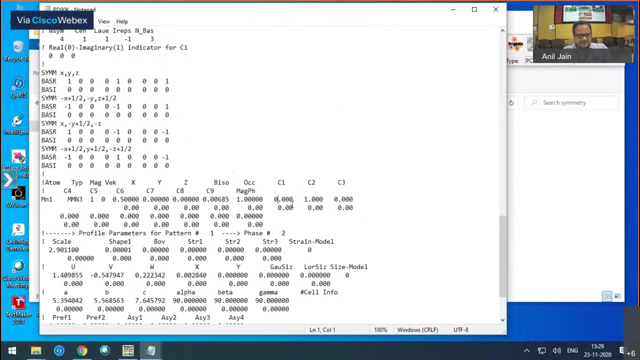 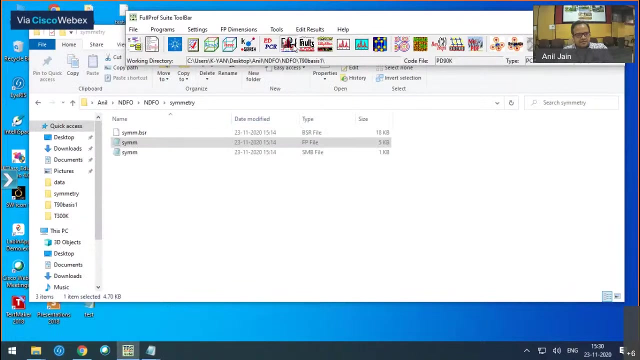 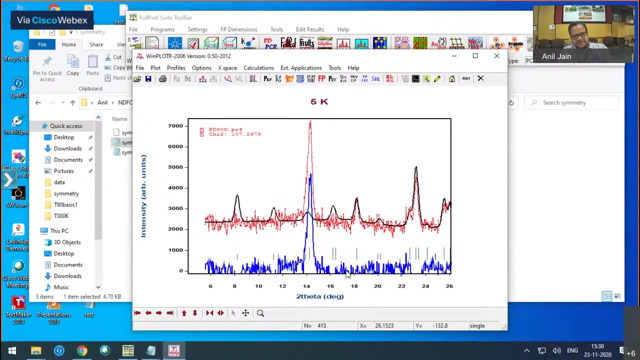 i can now let us try to see the magnetic structure. so now you can see the moment is along the b direction. you can see it here. i can also put all this coefficient and try to see whether it helps me somehow. you can see it here that still i do not get this. 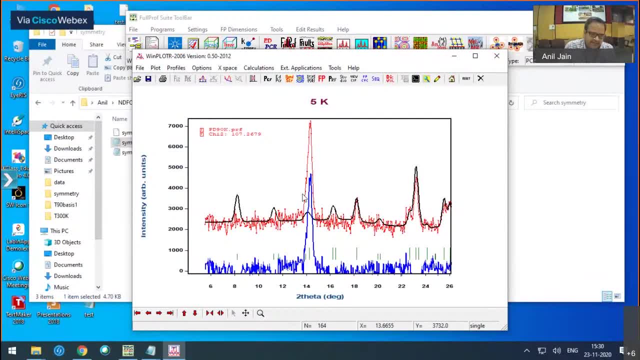 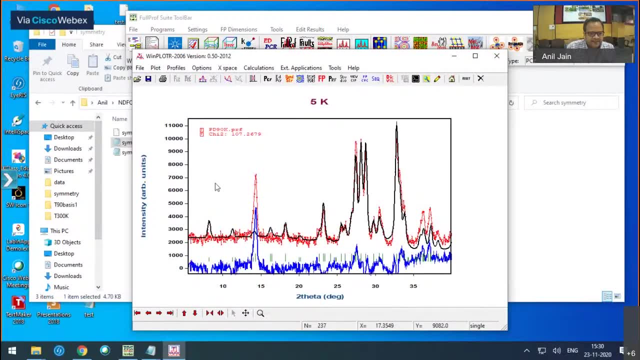 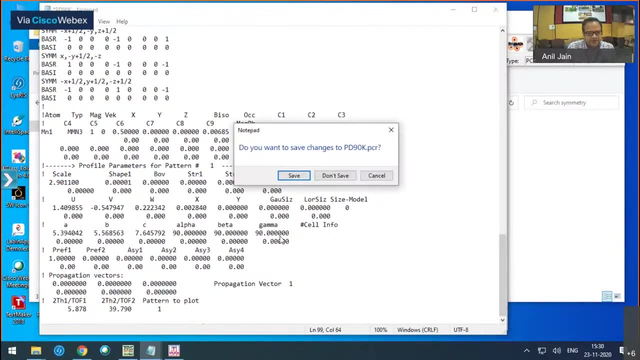 good increment with the experimental data. in addition, it gives me this peak where i do not have any intensity. so this peak, if i try to play with this coefficient, if i make this c 1, 0, let me see how it looks now. so c 1, 0, i have made it. 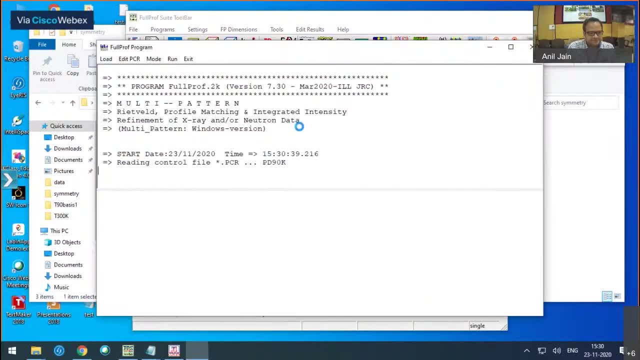 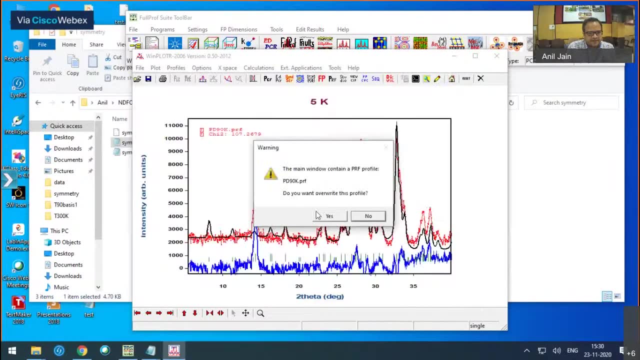 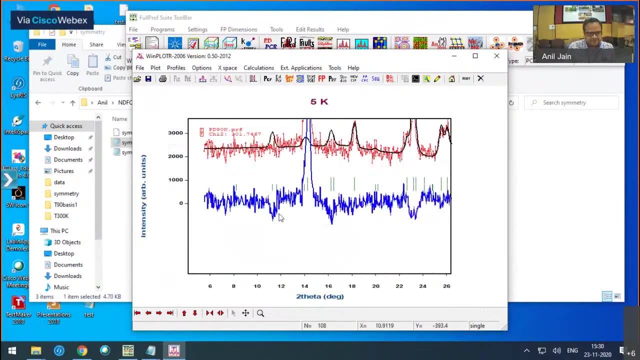 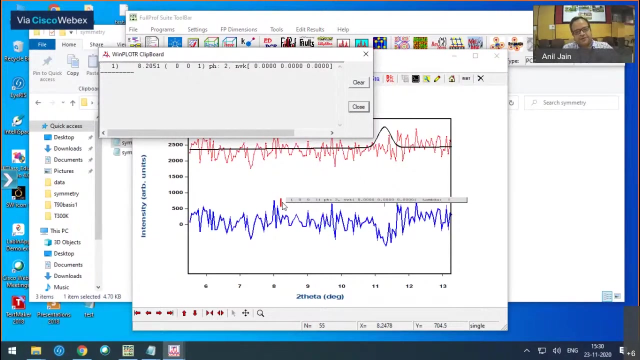 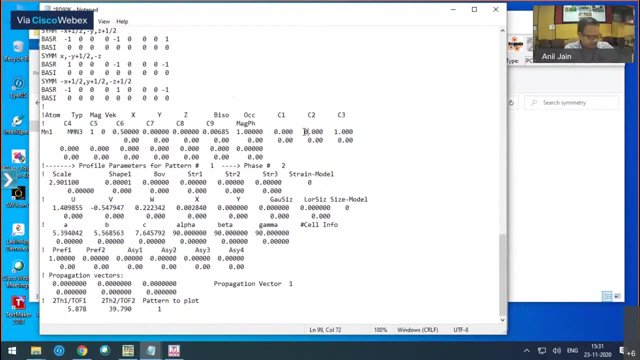 now and i ask it to run. so it means making this coefficient c 1, 0 is trying to make this intensity here small. so we have the intensity when we have the c1 component at the 0, 0, 1 location. now suppose if i make c 2, 0, how it happens- h looks like voice name- if i make c 2, 0 now. 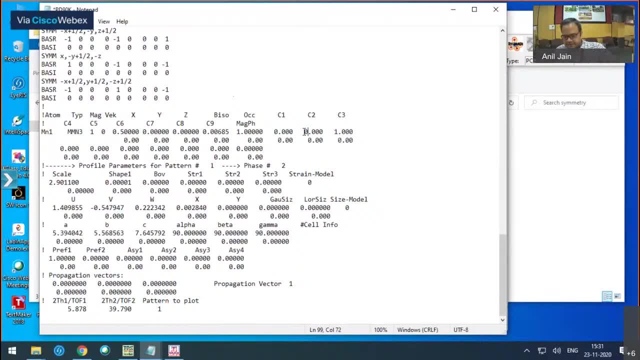 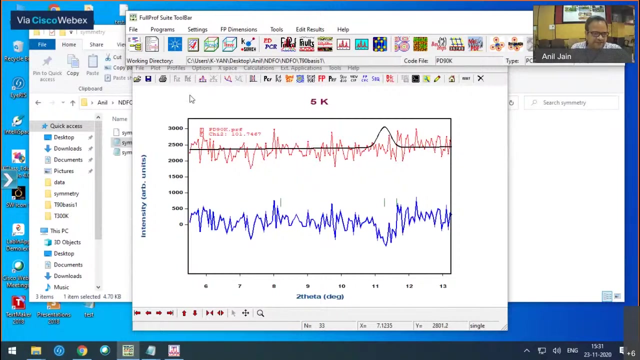 you can use vishnu voice. so if i make it the coefficient c 2: 0, let me see how it looks like. c 2, c 1, c 2: 0 means i have the only one coefficient, which is c 3. so, as per this basis vectors, 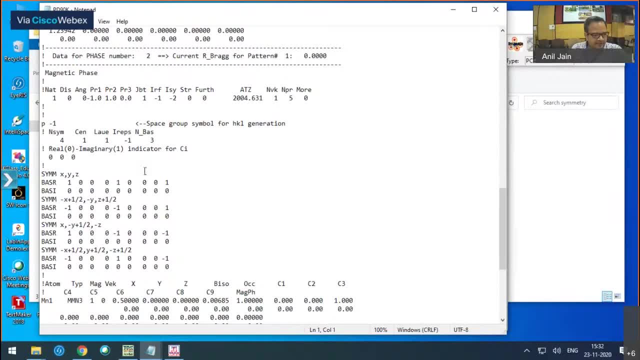 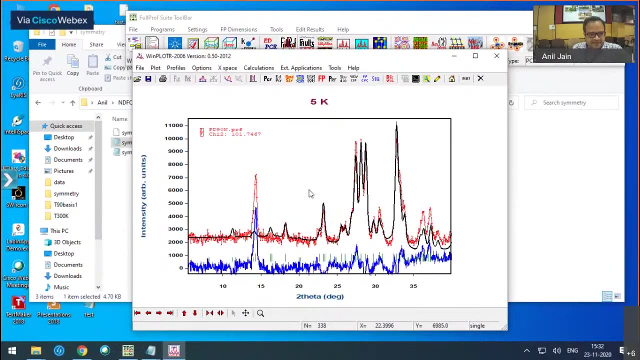 now i have only the coefficient associated with this, so my moment is along the c direction, and if i try to run this program then you see it. this also do not help you in creating this proper intensity. so this is the cycle one has to go through always once you have this kind of 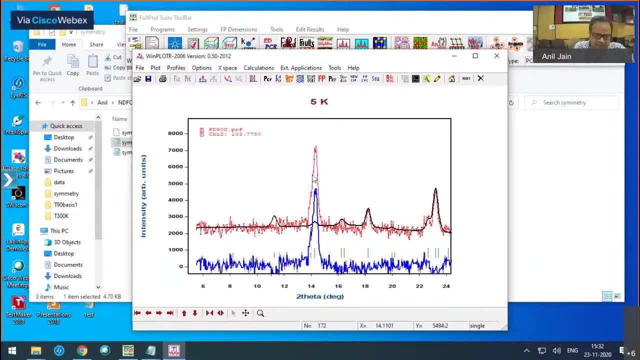 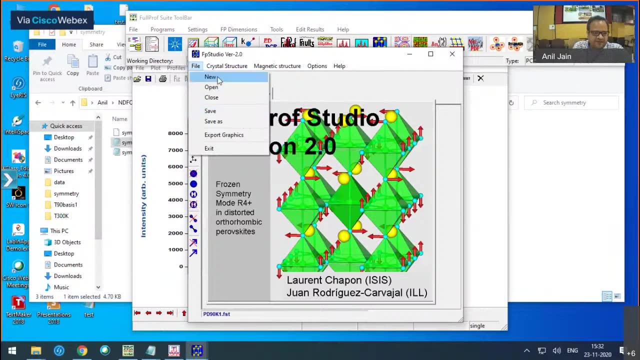 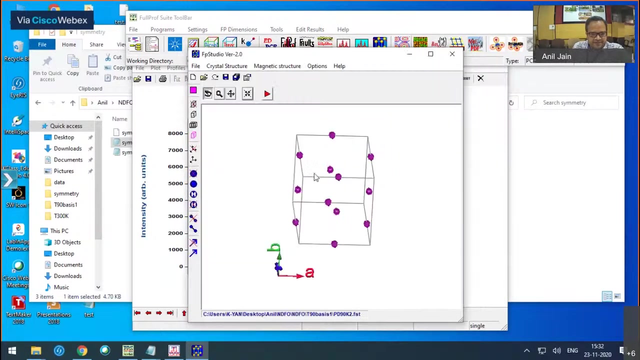 representation analysis and the idea is to see whether you can get this accurate magnetic intensity, what you have been seeing in the experiment and now, quickly, you can see that what kind of magnetic structure it corresponds, because you might have some idea of this moment direction from some other experiments. so let me put it here, so, as i told you that, if i put only 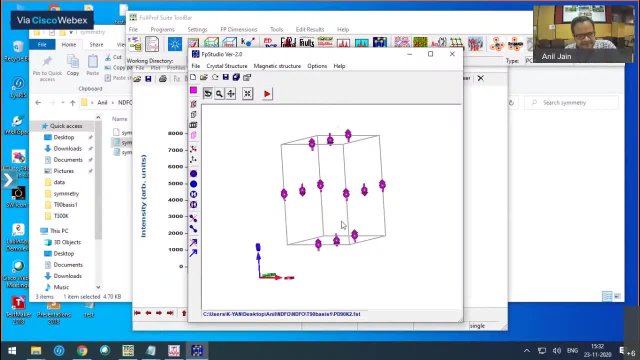 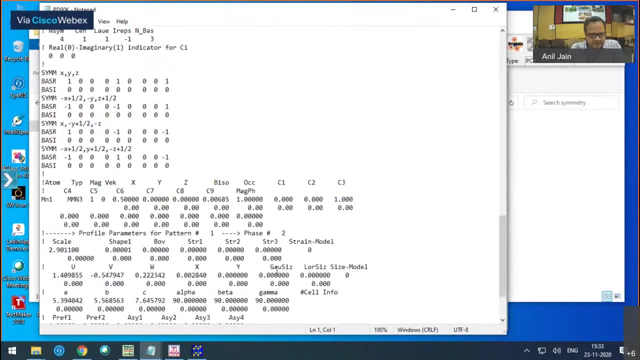 the coefficient c 3 component, non-zero. c 1, c 2, 0. with those basis vectors, my magnetic structure will have component where the moment will be along the crystallographic c direction. so this is how we proceed about this magnetic structure. now you can see it here. you want to? 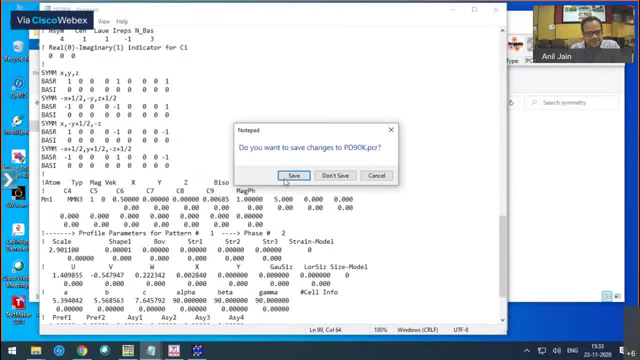 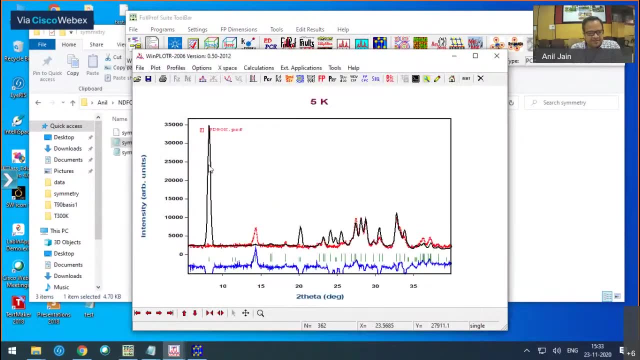 generally quickly see it. generally. i put a huge moment and try to see it whether i am having some intensity at the location where this program is generating. so this do not looks to be very favorable condition for the magnetic ordering for this compound. so then what we do is we 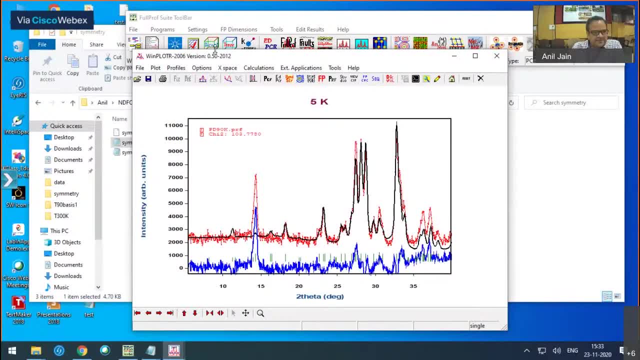 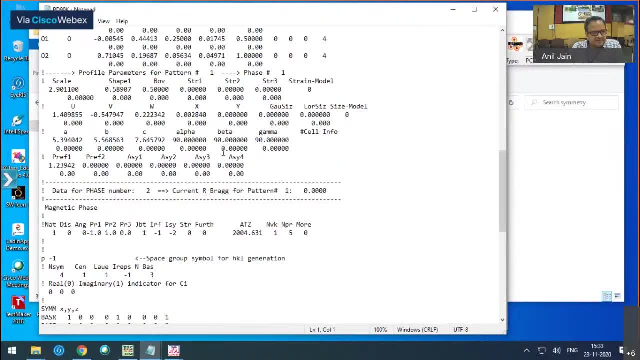 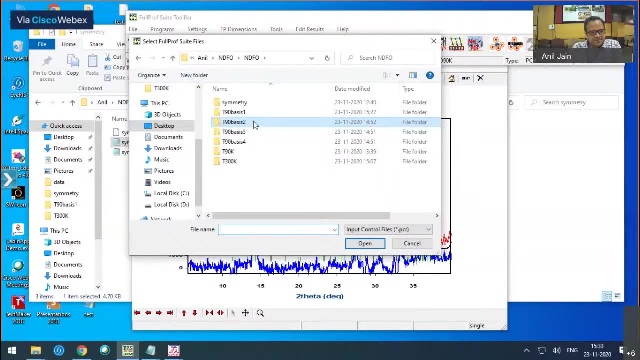 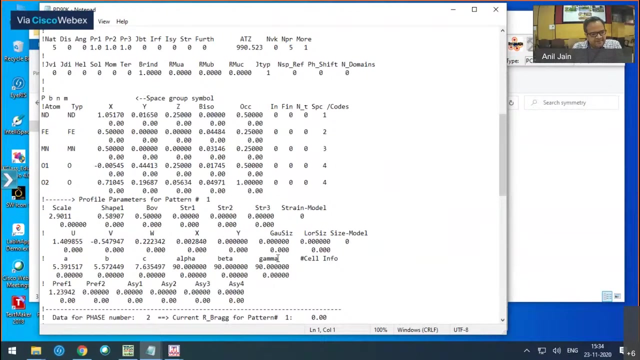 go to the another representation. so what i do now is so for going to another representation, i will try to go in the another directory where i have marked it with the basis 2.. let me just open it. so here. this nuclear phase is same what we have. 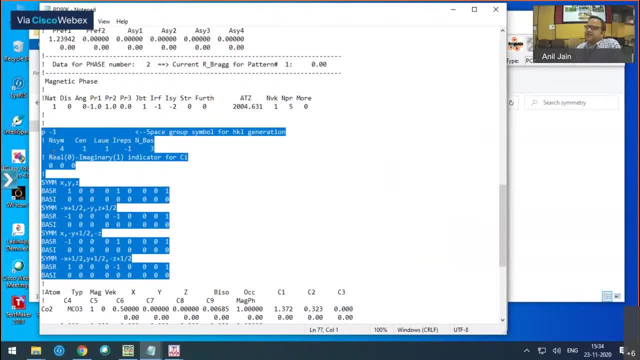 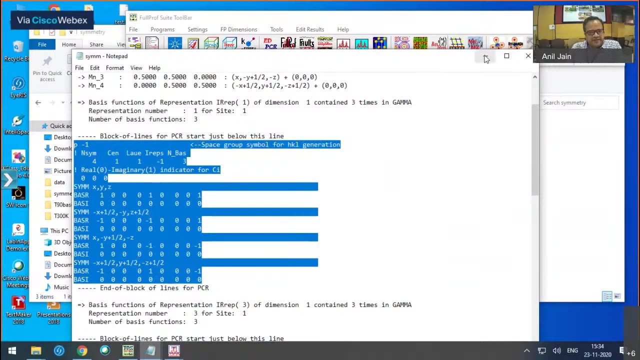 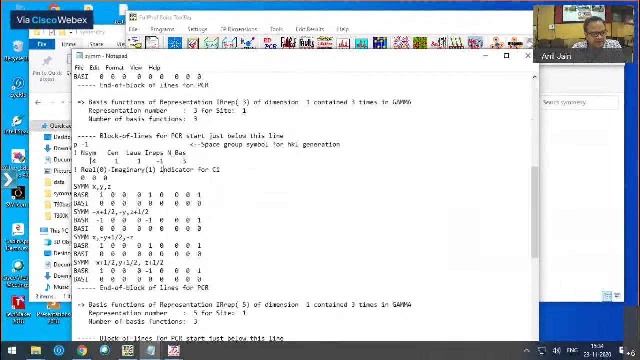 to change it now. we have to change this part of this magnetic phase. now, how to do it? again, as i told you, what we have to go do is we have to go to this fp file, which was generated by this best reps program. so now i go to this number. 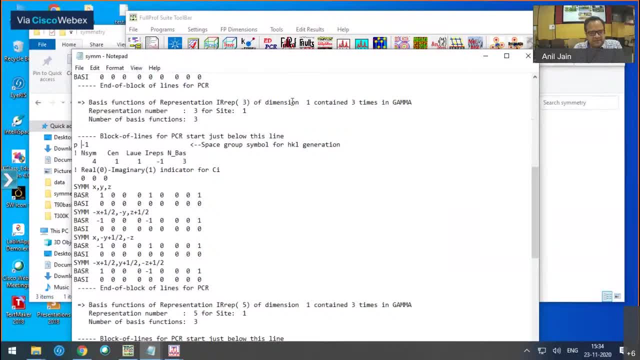 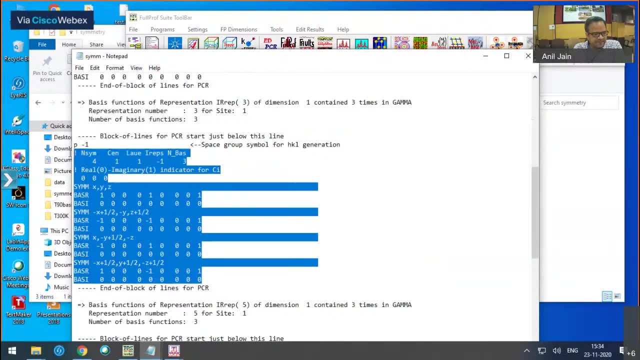 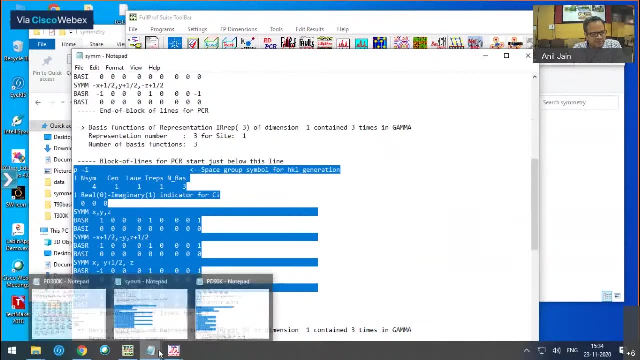 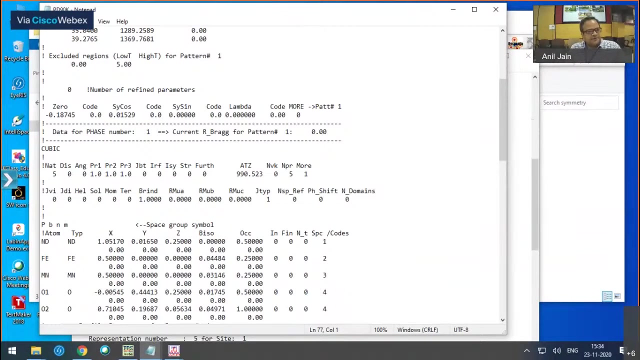 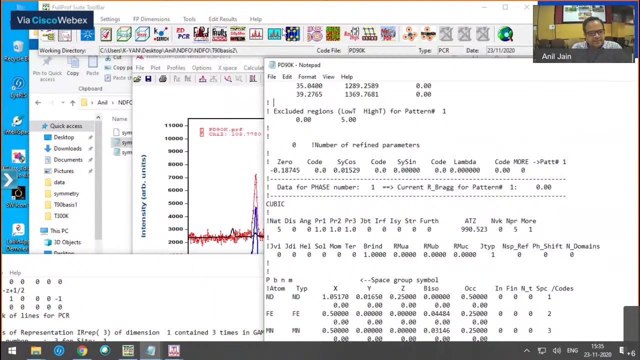 basis function of the representation. i rep 3 of dimension 1 contain 3 times in gamma, and i go with this representation now. so what i do is i copy it here, and so this is the symmetry. so this is the file we are working now. so what i have to do is: now i have to replace. 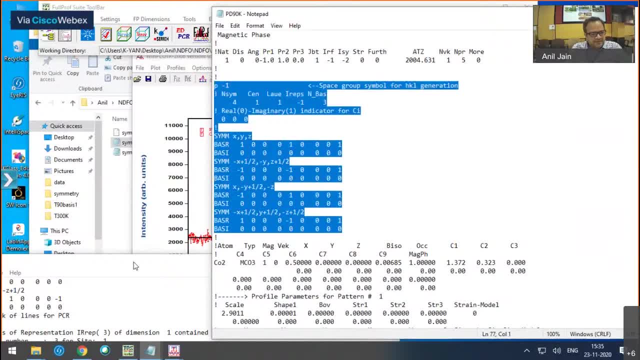 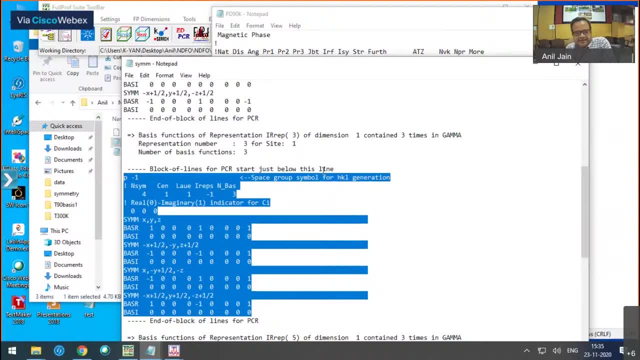 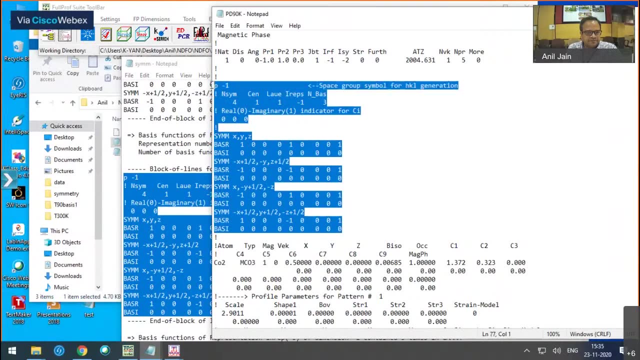 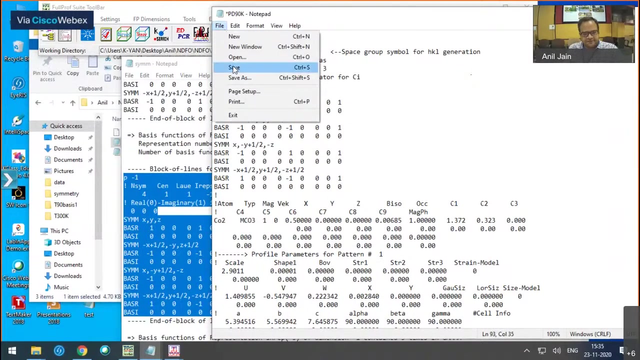 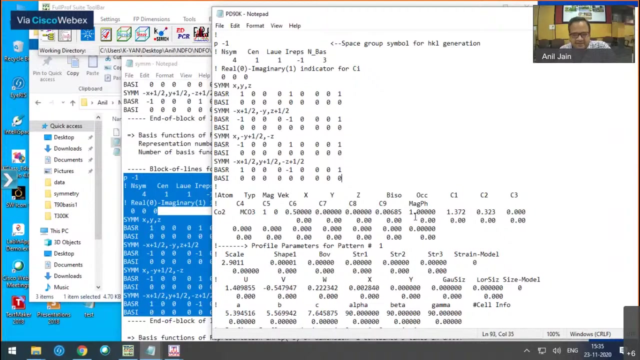 this part in the pcr file, by this part of block of the lines which was given to me after running base reps. so copy it. I have pasted it here and file save and now rest. other things are the same which was there in the previous pcr file. 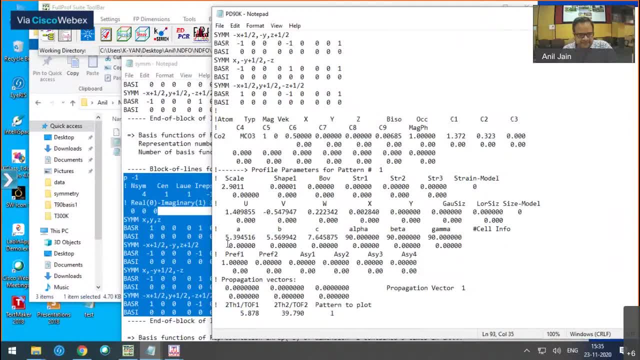 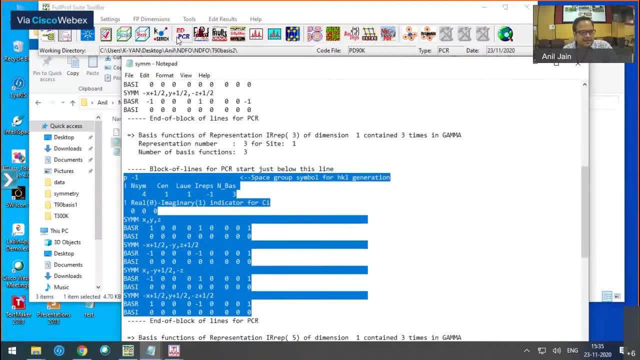 you can see it here. these lattice constraints are the same. now, once you do it, it is always better to close this file and try to see in the edit pcr whether you can open this file. this gives you confidence that what you have to do is you have to run this. 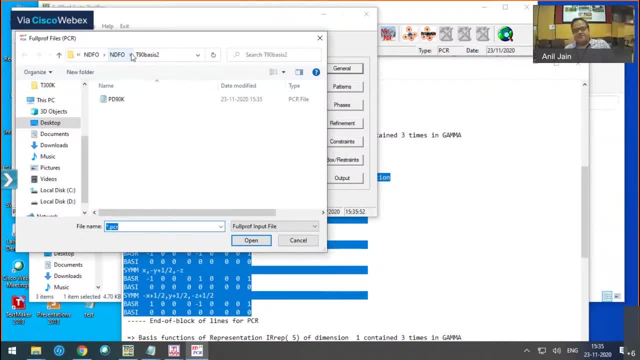 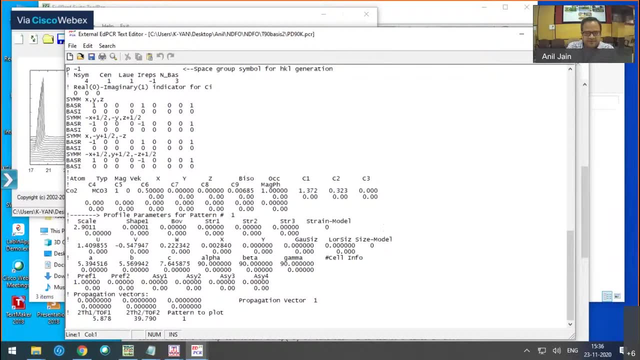 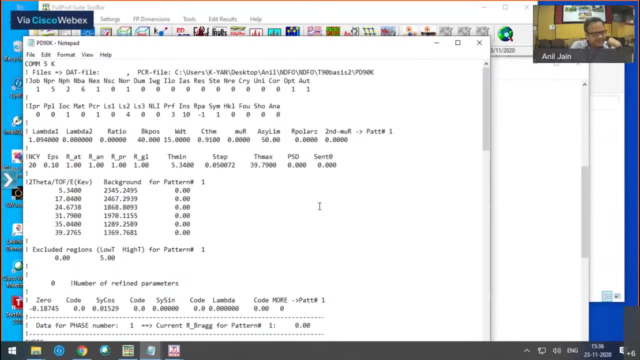 What you have done is alright as per the language of this code. So I see it here. everything is alright. now I close it here and then see it from here. So here again, I would like to make the number of cycle. let's say only one, and I would make 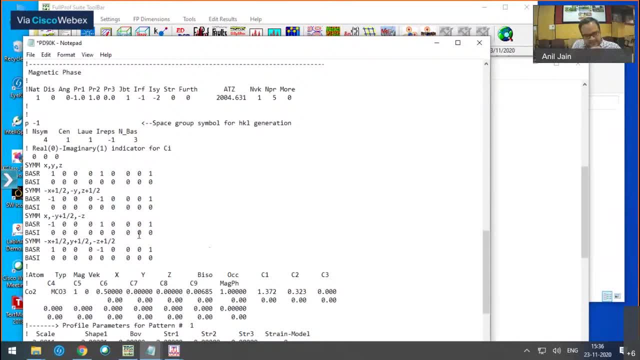 the number of refined parameter zero, and then try to see it that if I can get this magnetic intensity at the location where I need the magnetic intensity, So again in this representation also you have the three basis vector which is given by n underscore, base 1,, 2, 3, and when you go from this position of your magnetic atom to this, 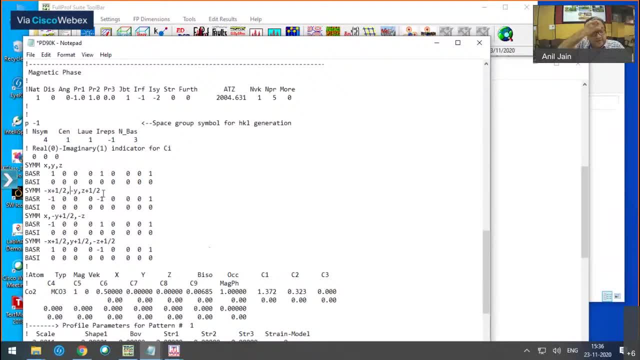 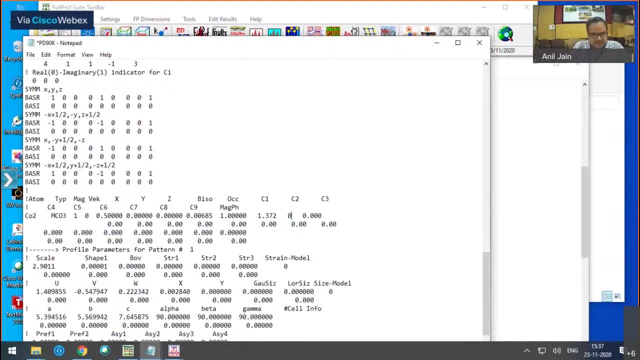 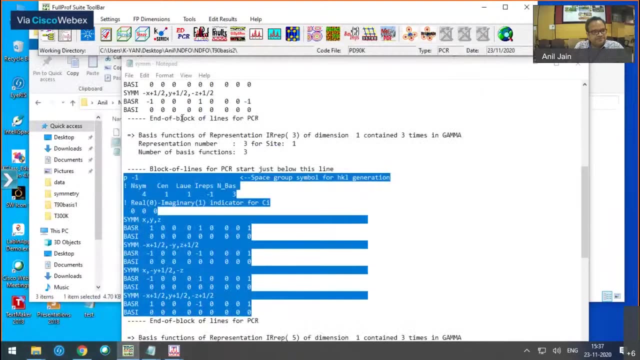 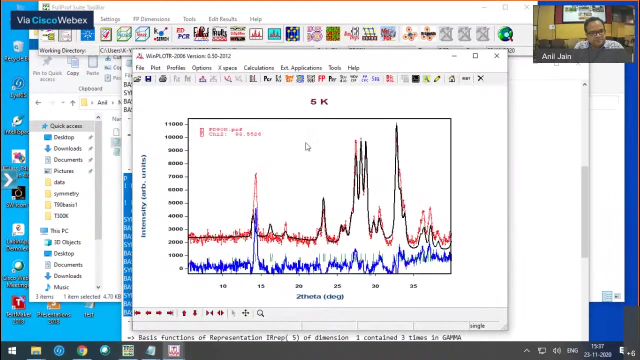 position. This is how this moment should relate from the previous position. So now let's try to make this thing zero and then try to see it how it looks like. The good part here now is I see this magnetic intensity Almost at the location where I need it. 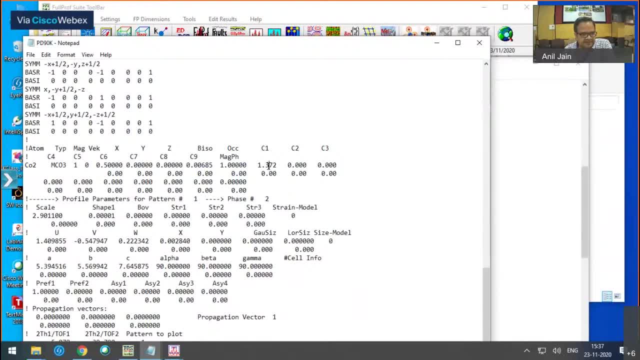 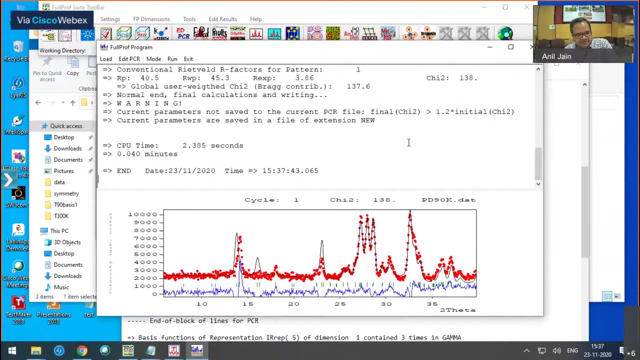 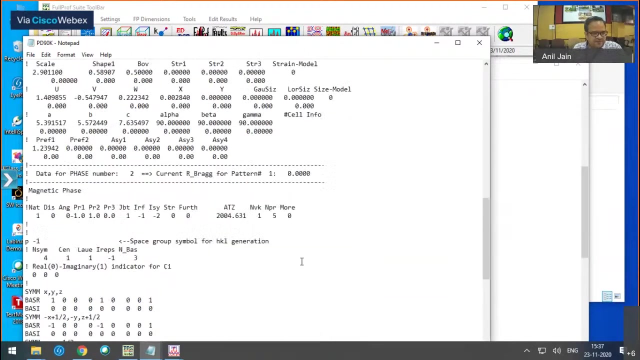 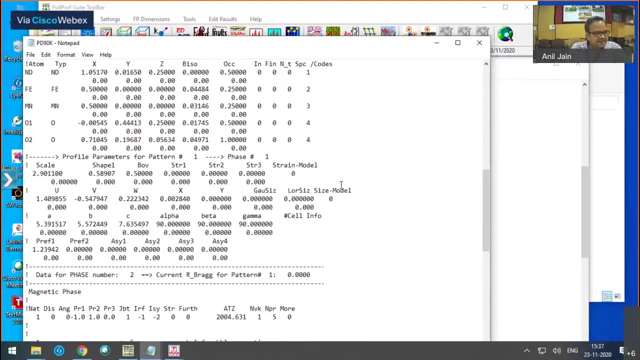 Only what I can do is I can little bit try to increase it and see it whether still ok. So it is generating the intensity, but it is giving me some symbol. So now I have some hope that This, This representation, might work, and what I do, that in that case, is this lattice constant. 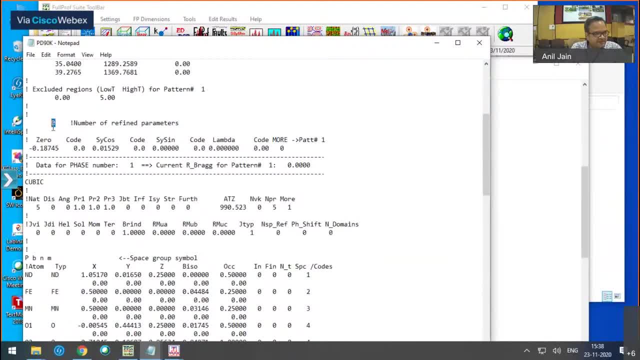 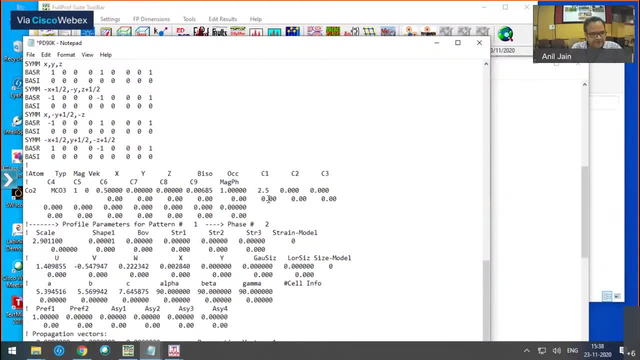 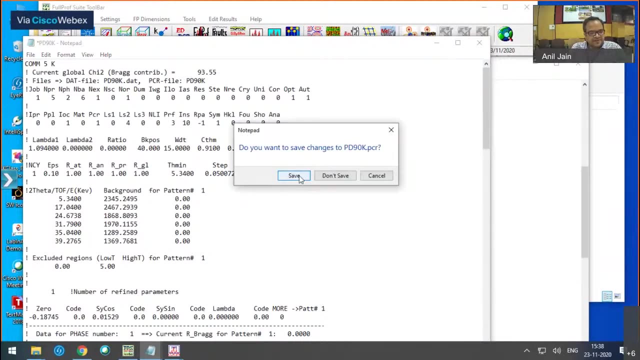 as you know, were refined at room temperature, Then I will quickly like to do the refinement for this file and then try to see it whether there is some hope to get this magnetic structure corresponding to this representation. So I have done now, So I have entered in the refinement mode now. 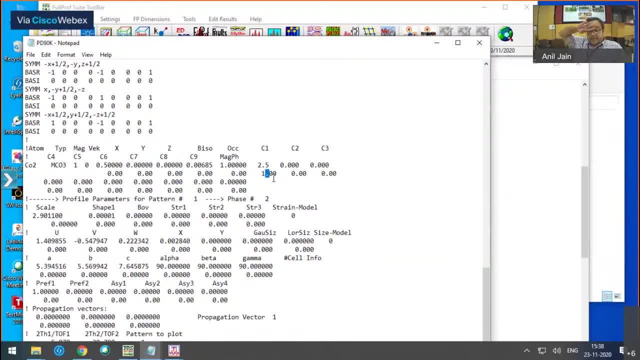 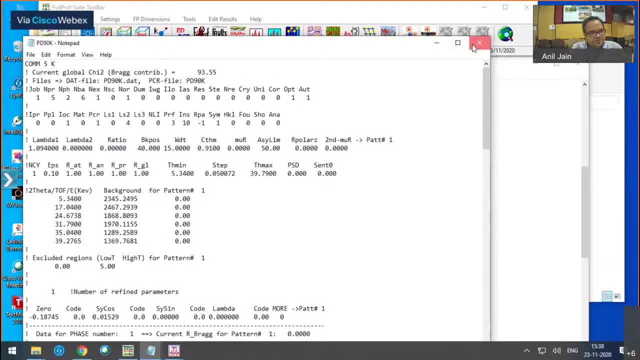 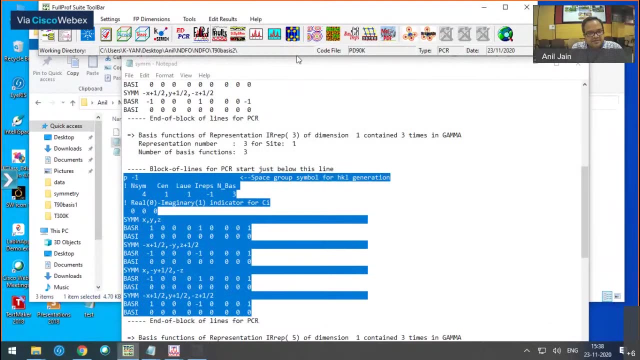 By putting this code 1 here. 1 means it will try to refine this parameter c1, because I am working in this automation mode. So now you can see it is trying to generate some intensity. of course it is little bit shifted, So we have to see it. 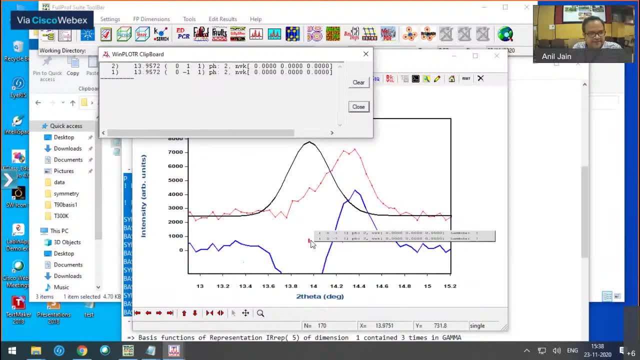 So it means it is generating the intensity for the peak 010.. But actually it is not 010. It is 010. 010.. So your peak looks like to slightly different location. Ok, Ok, now what we can do is: 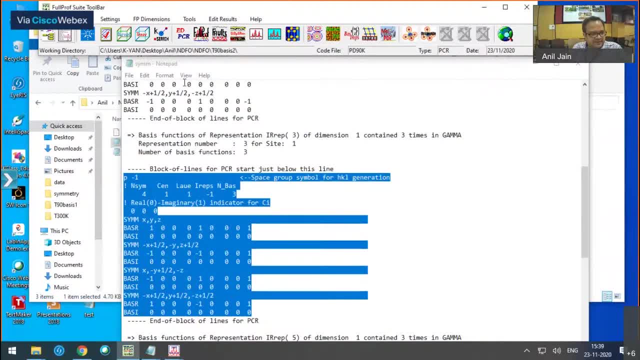 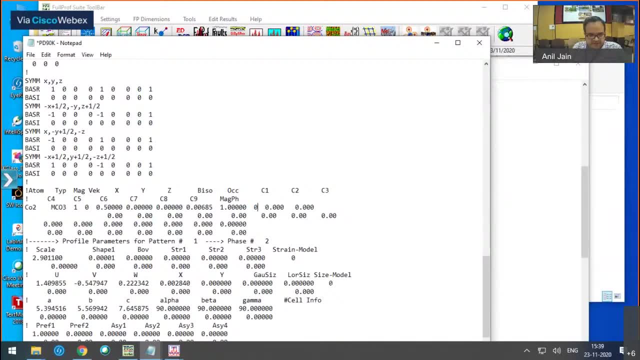 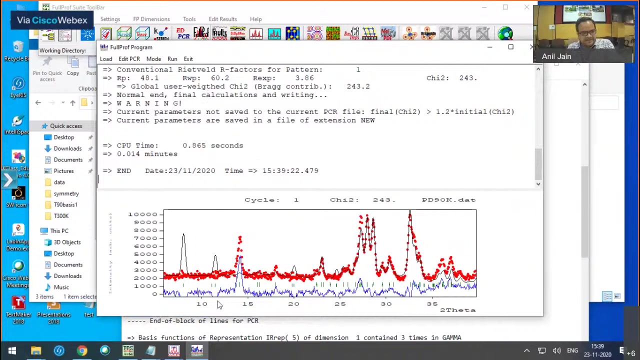 We can play it with more And instead of this coefficient, 1 coefficient. I can see it. what happens if I put this coefficient Here? Oh, Let me save it. Ok. So this is not good. as you can see, it is generating the intensity at different location. 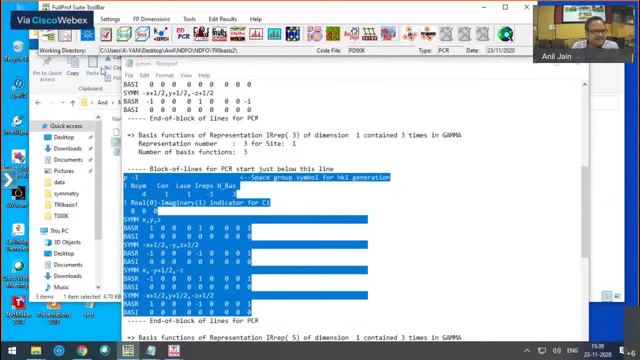 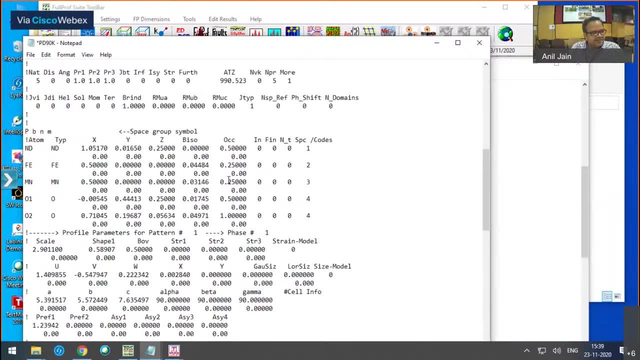 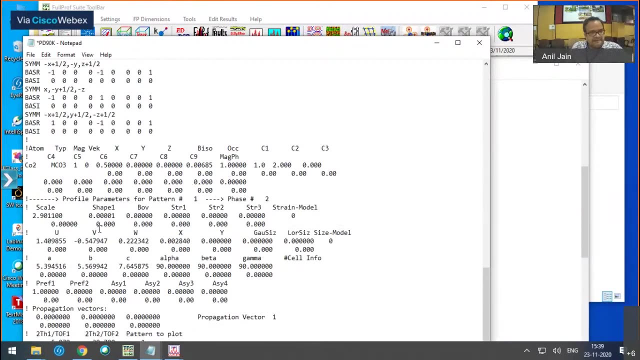 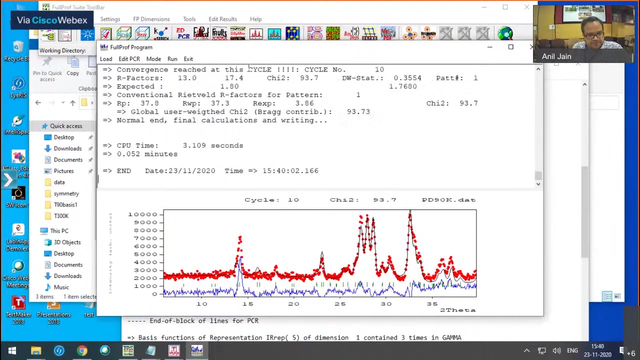 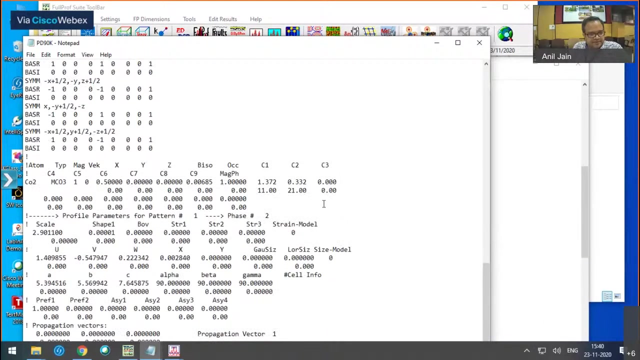 So this is how you make a progress in the refinement. So then I can put some value here. I can increase the number of cycles, lets say around 30, then I can enter in refining this two parameters: C1 and C2.. Let us see how it looks like. 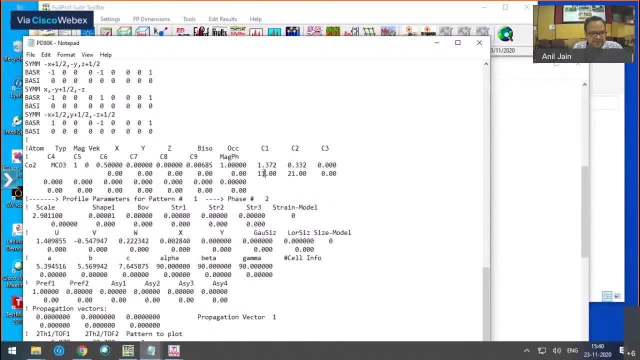 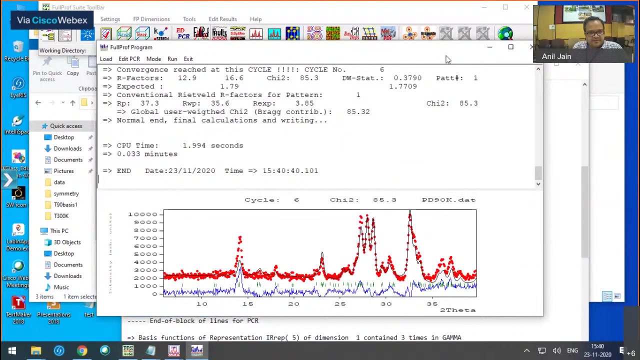 So it is increasing C1. try to decrease the C2, you can play it little bit more. and now what we can do is We can try to refine once this ABC, because they were refined at room temperature. so what I will do is I will try to refine first for the magnetic phase and then, ok, so you can. 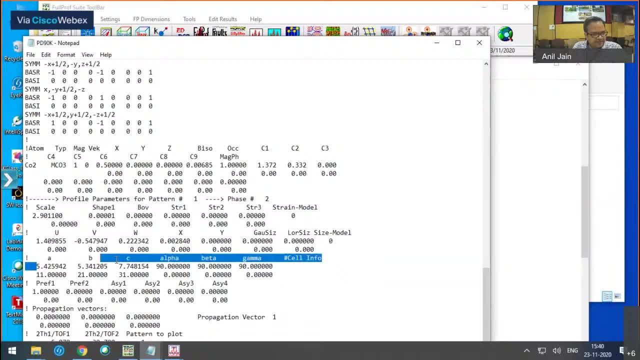 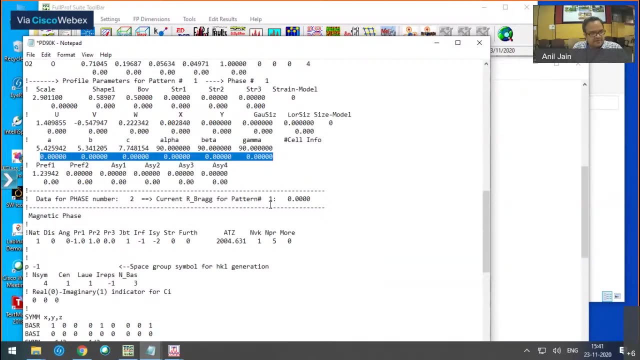 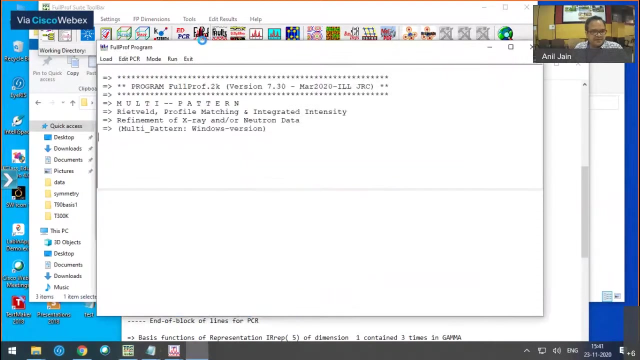 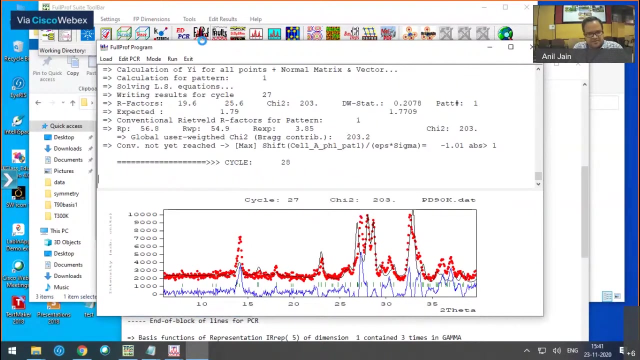 see this: our lattice constant has been changed a bit. I can put For the nuclear phase and then I would like to refine them with the same code. Let me see how it looks like now. so you can little bit play with this, not much, and then 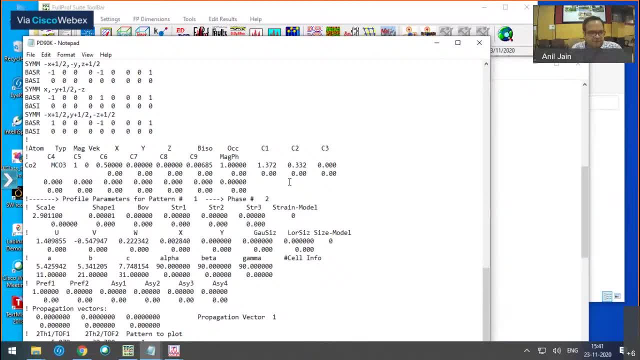 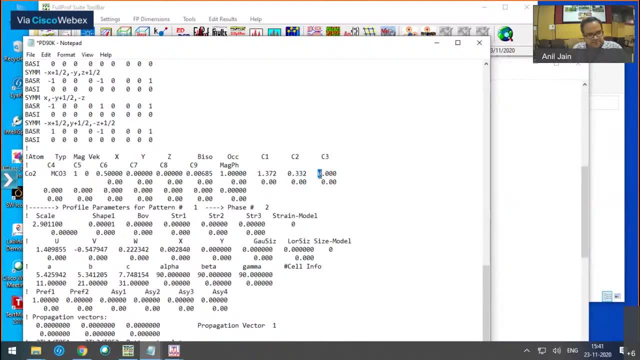 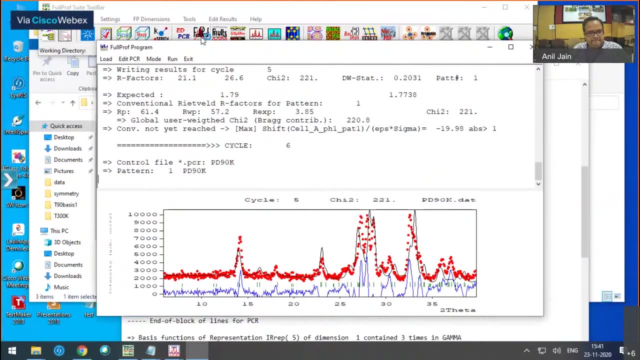 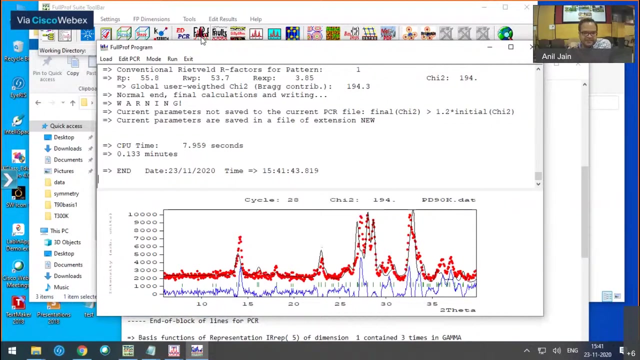 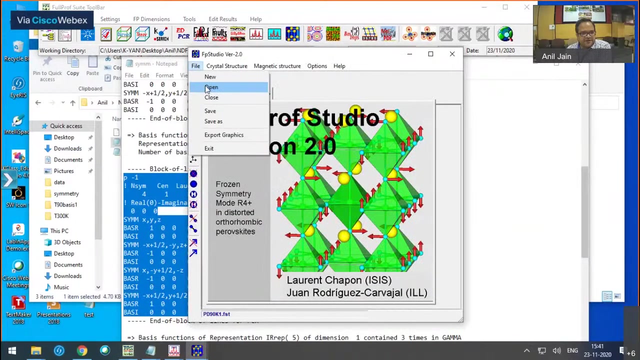 you can play with this coefficient C1 and C2 and if you want to introduce, you can introduce this coefficient C3 here. sorry, Now, when you introduce this coefficient, either you can calculate or you can see from the studio then what kind of magnetic structure it corresponds. by giving this coefficient, 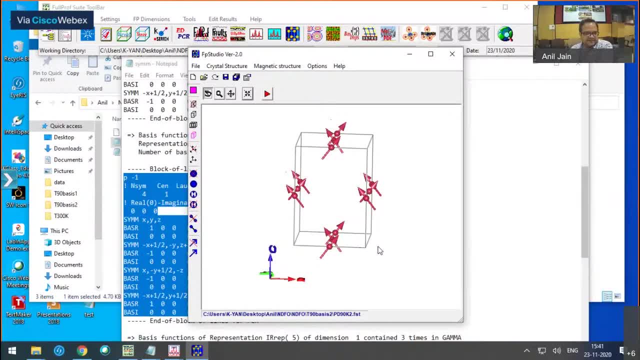 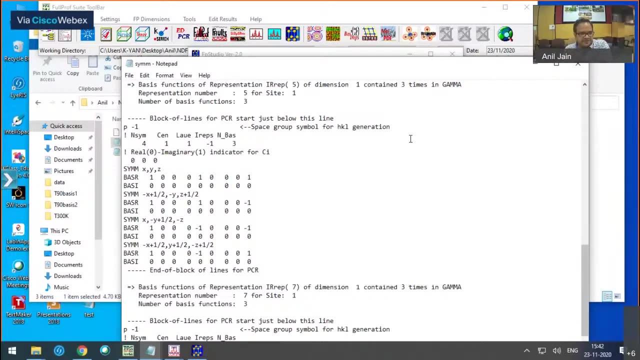 So you can see, so this is the formalism- how we keep this moment in terms of this basis vectors. similarly, I have done this for the two and you can try to do this for the rest of the two. Let me quickly do it for the number three also. 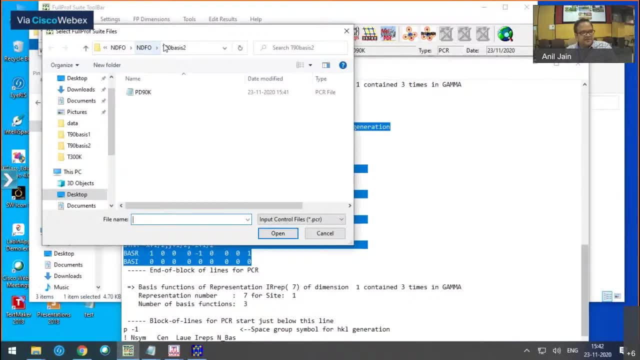 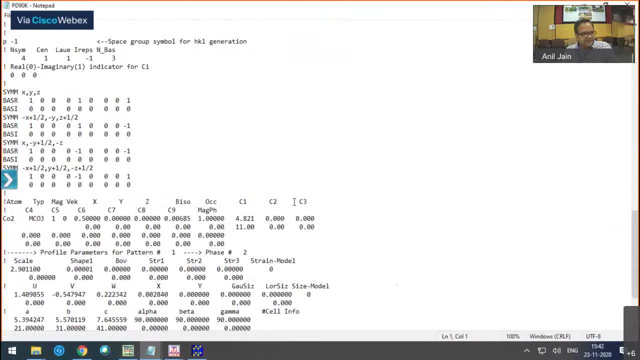 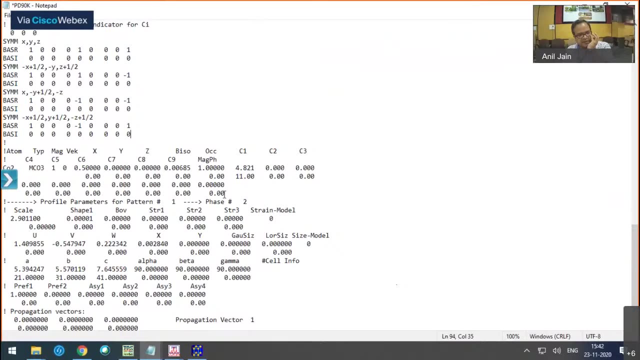 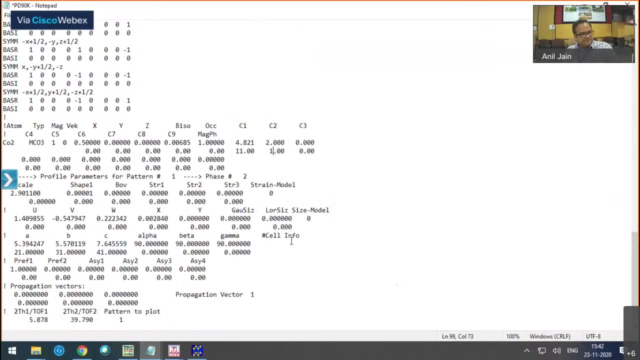 What I can do is I can copy this. I have kept here this replica in this number three. I go here and again. what I have to do is I have to change this part of the PCR file. Now, again, let me try to refine this codes and see how it looks like now. 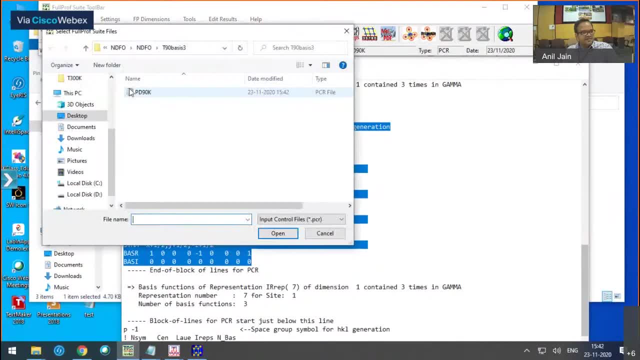 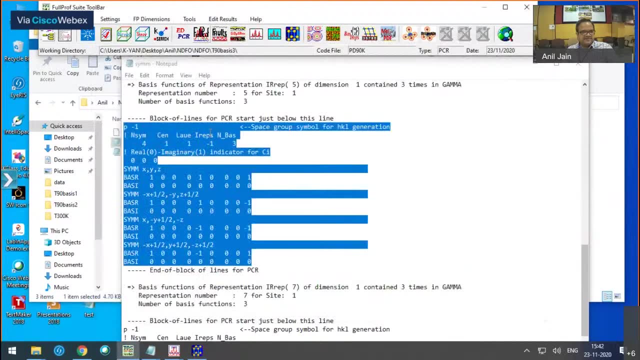 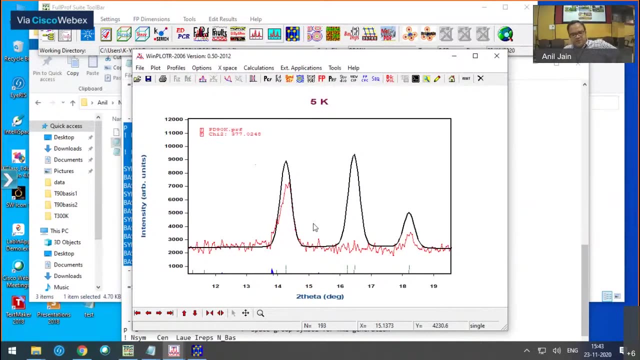 Let me again check, Ok, Ok, Again, run it. So this is not good because it is generating this intensity at this location. So this is the way one should try for all this representation, and when your magnetic intensity matches, you can stop that point and you can see what is the magnetic structure. 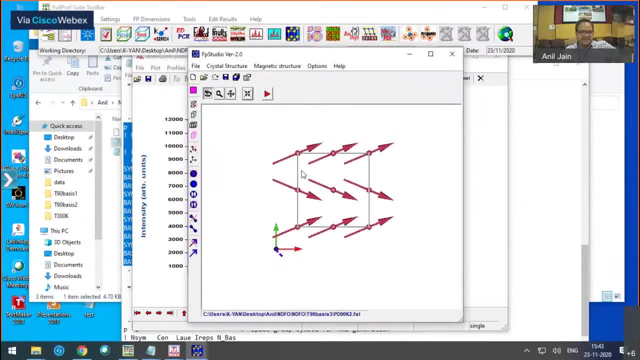 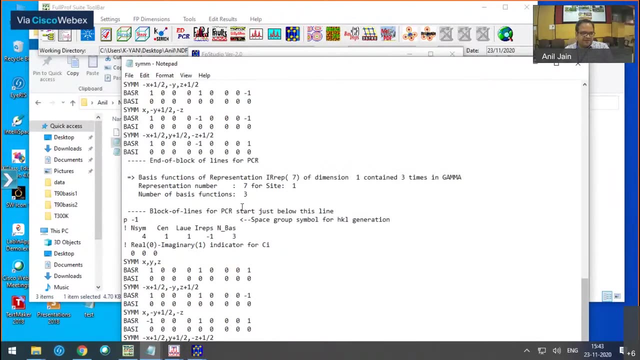 and what are the values of moment at the side? Ok rates by given, by your refinement. So this is the way how you put the moment by this basis vectors. So in this case, this case is simple- we have only four kind of representations. 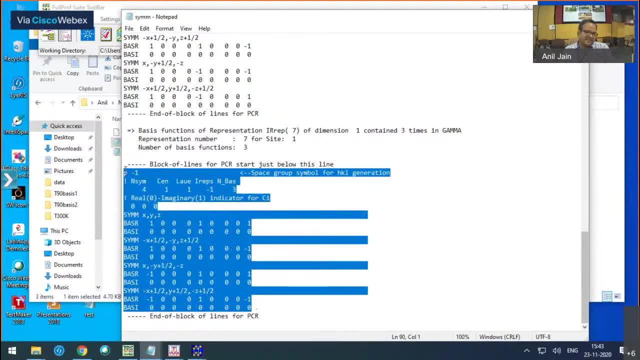 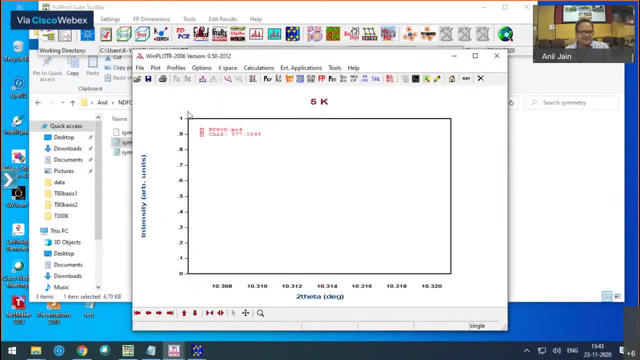 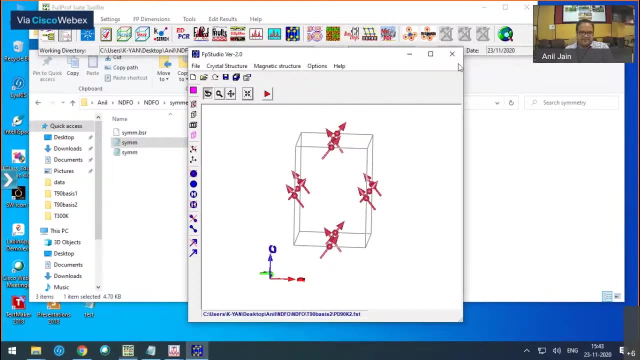 are coming, So you can easily repeat this for one more and see what kind of result you get. Another way to write is this PCR file, the magnetic phases by this symmetry operations. So this also comes when you try to run this base refs file. So let me show you how it. 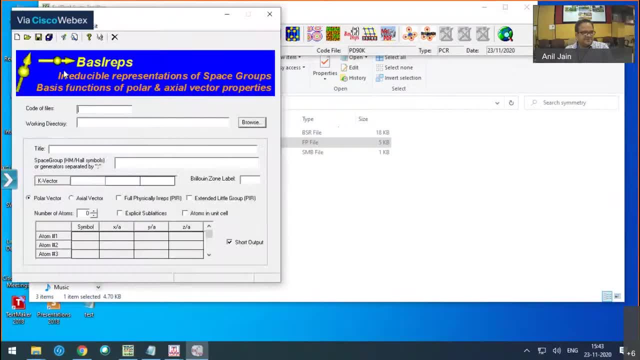 comes. So this is programmed base refs. Let me open the file which we did last time. This is the same file which I have run last time and let me run it again. So in the results there are two parts. One is the BSR file. 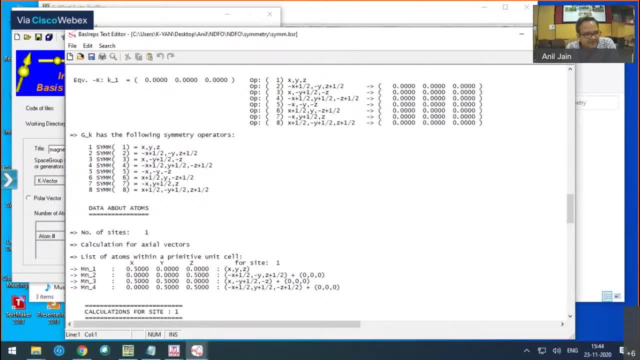 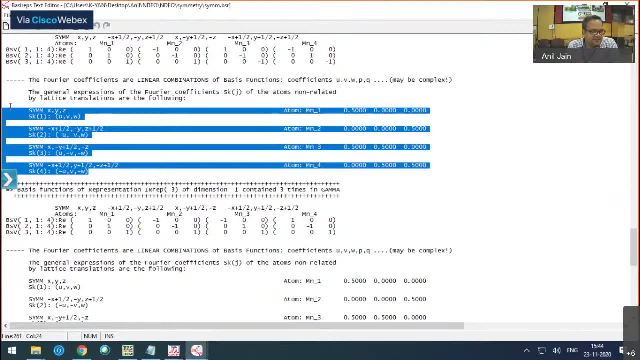 Let us see the BSR file. So this file gives you the information. if you want to put the moment in another format, So these are the information here. So this gives the general expression of the Fourier coefficient Skj of atoms known. related: 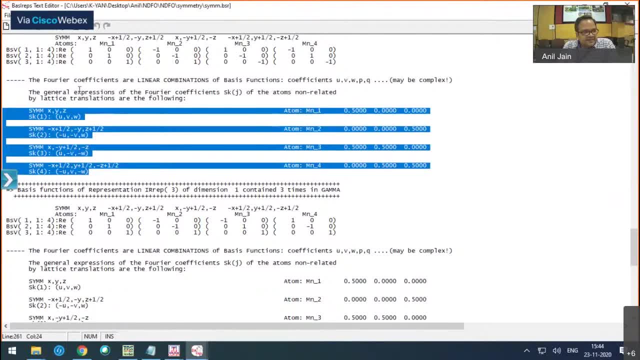 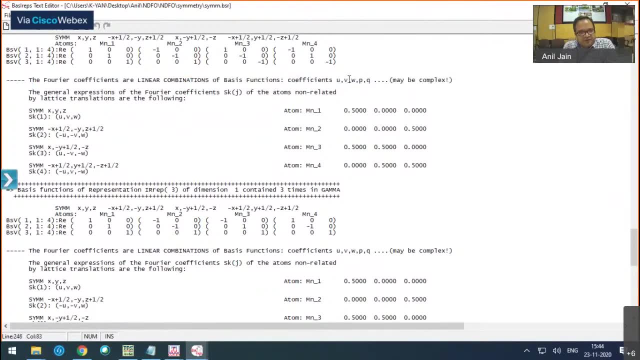 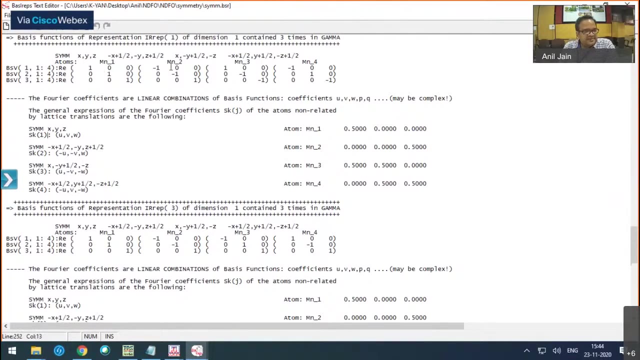 by the letter translation. and the Fourier coefficients are the linear combination of basis functions and coefficient of this basis functions are u, v and w. This u v and w and this is how it has come. So it is u times this, v times this w times. this for this side. 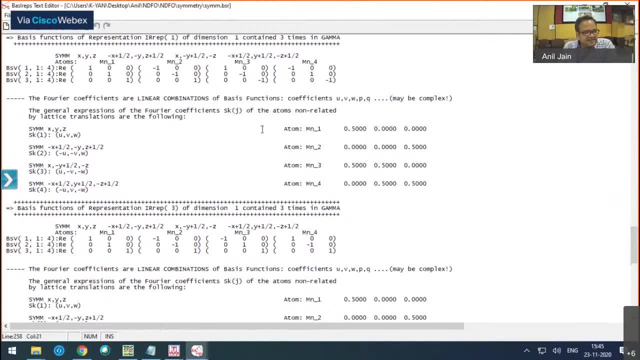 Similarly, you can write it for this side, this side, this side. So this is u v w. this is minus u minus v w for this position, For this position, this: this is u minus v minus w. u minus v minus w. 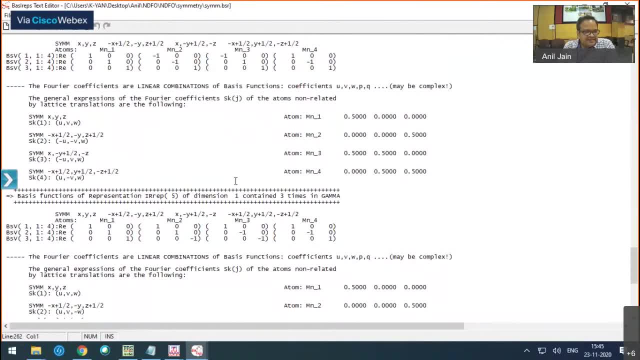 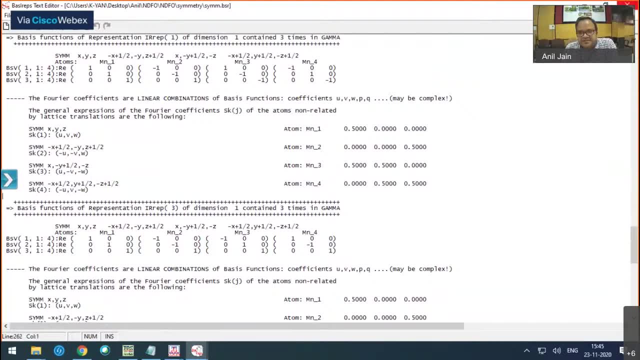 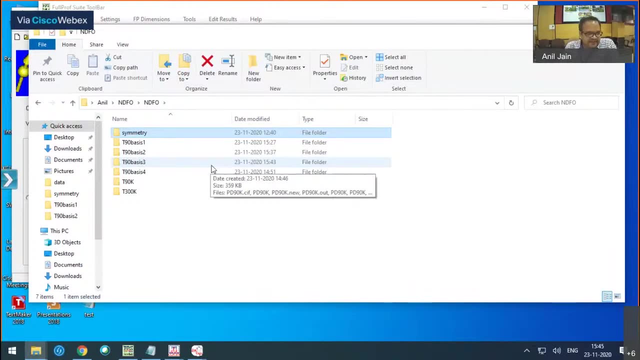 Similarly, you can write for this side and this is represented for all this representation. Now let us see how we go ahead with this formalism. Now, what I do is I go to this another way by which you can add this magnetic phase. So this information now is in the terms of: 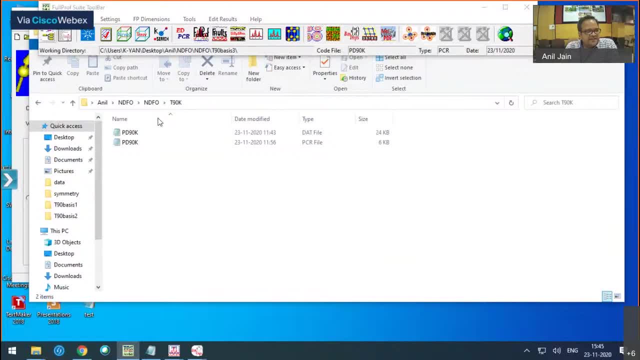 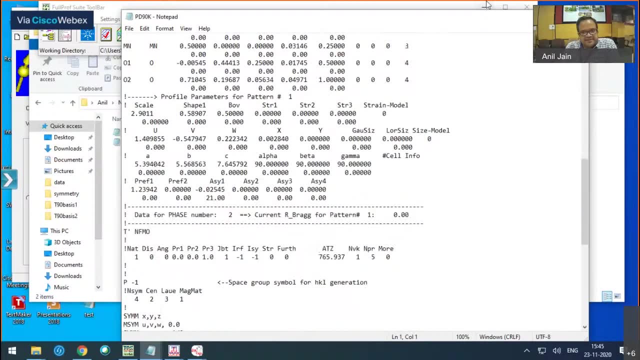 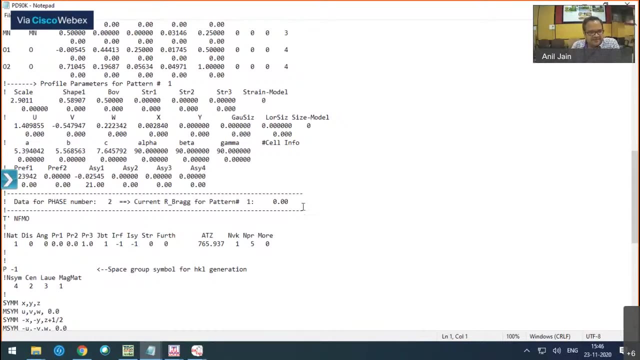 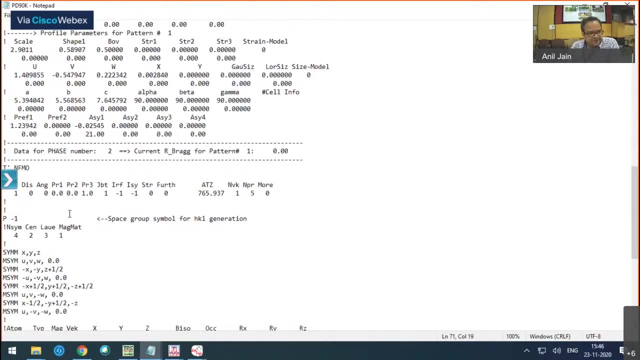 Symmetry operators and how this PCR file looks. now try to make it here and let us see So. first part here is still the same as previous. We have two phases, and now for this phase number two. you can see it what we are having. 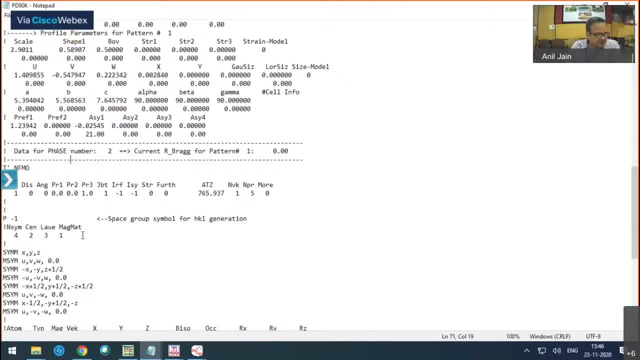 here isy equal to minus 1.. So what we will give is this: we will give this symbols Magnetic symmetry. we will put in this PCR file like this: So when I writing isy equal to minus 1, it means I will be putting magnetic symmetry. 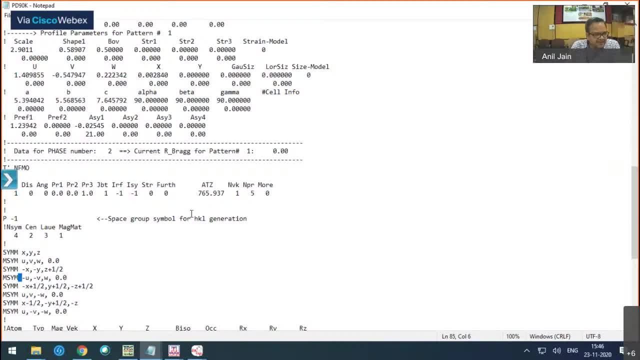 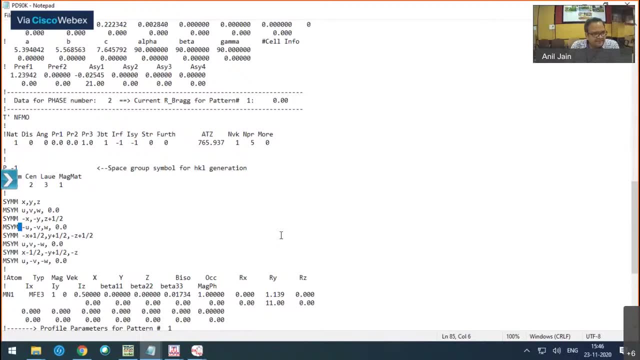 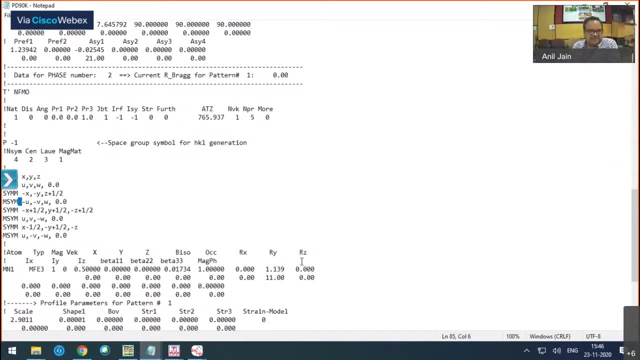 instruction in the PCR file. Rest other thing I believe is the same Now here. in this case, what we are giving is the information about the moment in terms of the direct projection along this x, y and z axis, Rx, Ry and Rz. 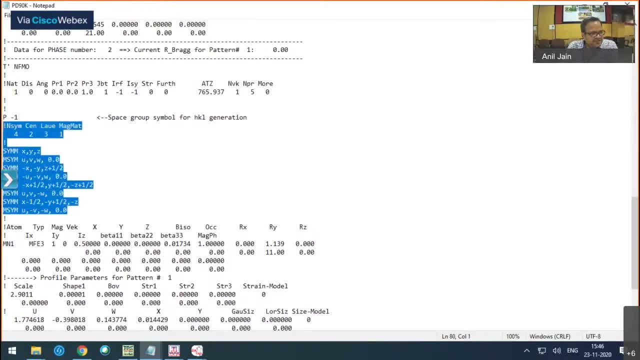 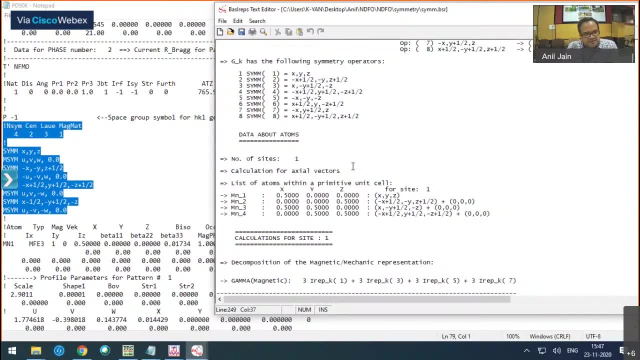 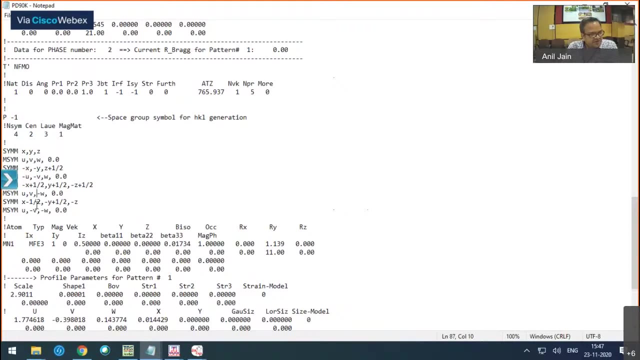 Ok, And this piece of this information, I am getting it again from this. You can see it here. So what it is telling is n sim is I have four symmetries: 1, 2, 3, 4, and these are Lave. 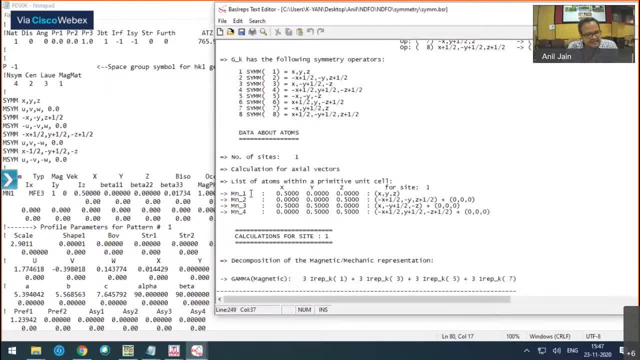 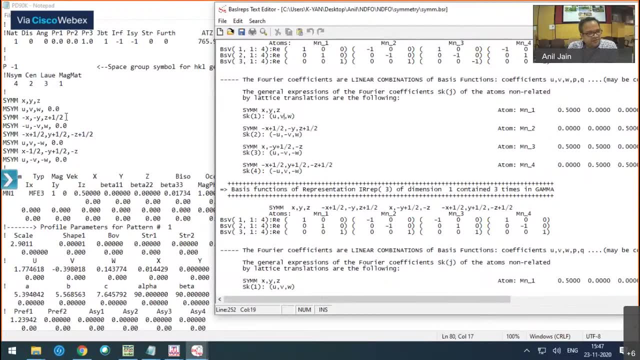 clasp And this value, how you write it, it is directly given in this PCR file here. Ok, Ok, Ok, So you can see that this x, y, z, u, v, w minus x for this line, this is the corresponding. 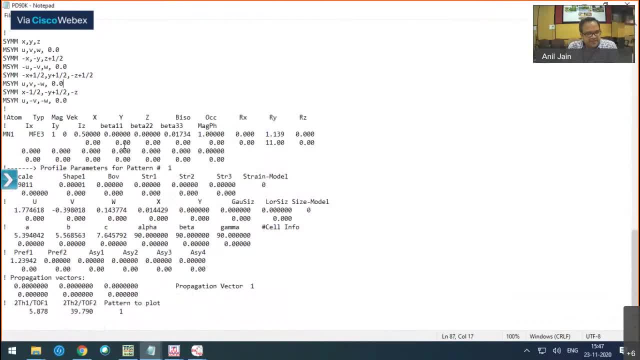 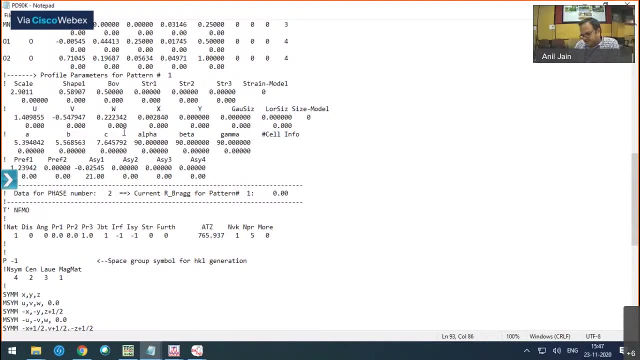 line and similarly for line number 3 and 4.. Now here the advantage is that you can directly put this value of moment with respect to your cryptographic axis, And please note that when you are trying to refine this magnetic structure, you can keep your scale factor fixed. 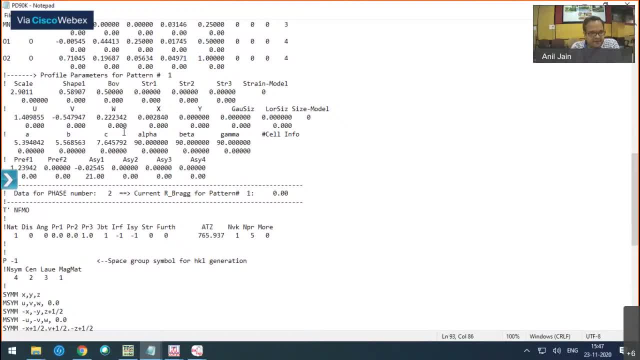 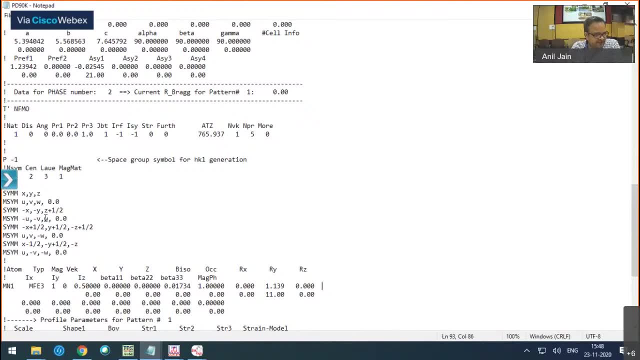 Once you have this scale factor fixed, you can keep the magnetic structure Once you have defined your data in the paramagnetic phase. Now let us try to run this file after putting the symmetry operation like this, which has been given in this BASELAPSE file: 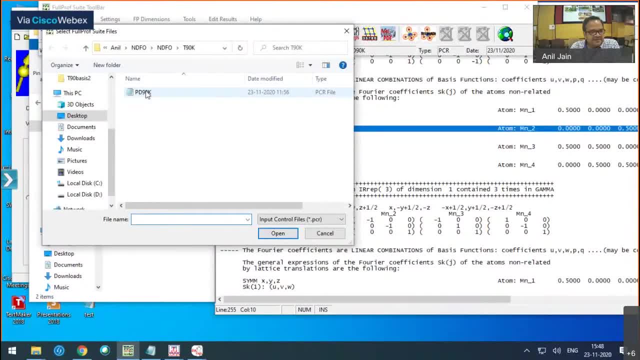 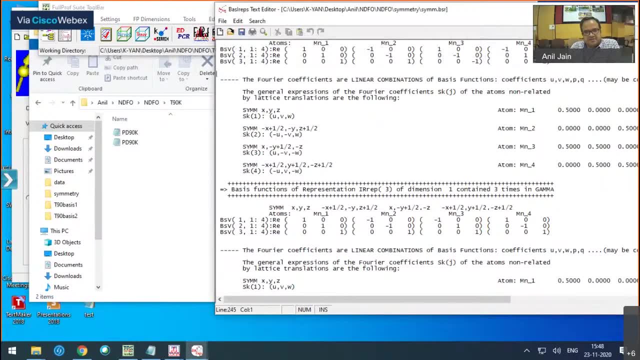 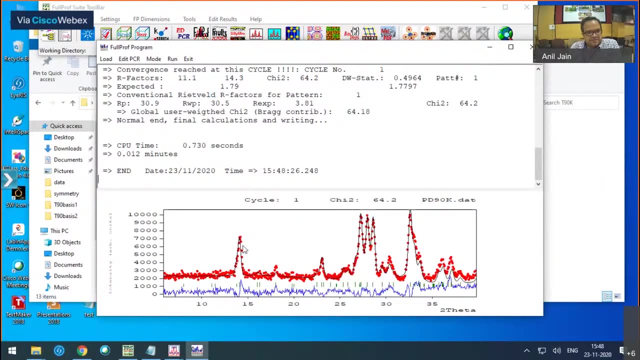 Let me again see it. if I am in this alright file, Ok. Now what I do is I try to close this. Let me run it Ok, Ok. Let me run it Ok, Ok, Ok, Ok. So looks like excellent. 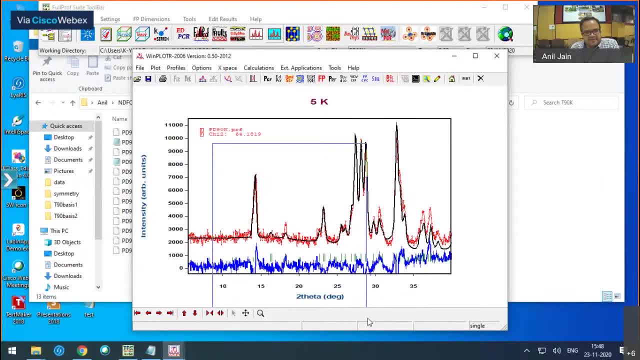 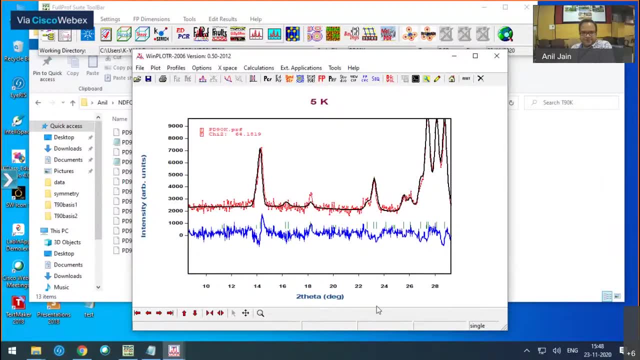 So we are getting very good agreement with this observed data. So this kind of fitting, if you tried in this basis vector information also, you can get it. So this is your choice how you want to work for this magnetic phase. Now again, if you want to play, you can play it. 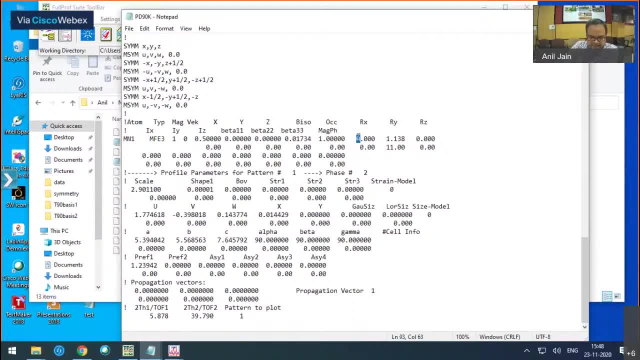 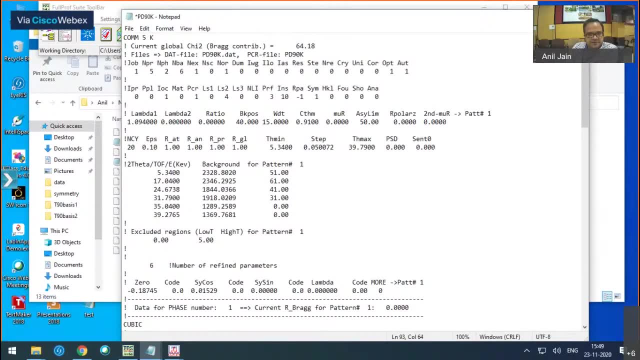 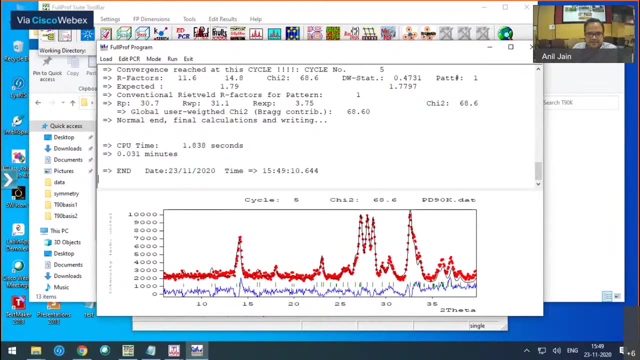 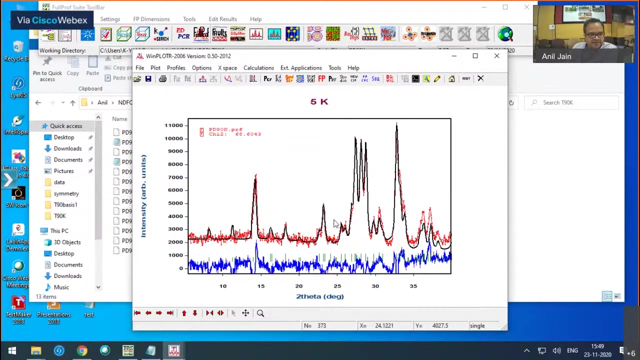 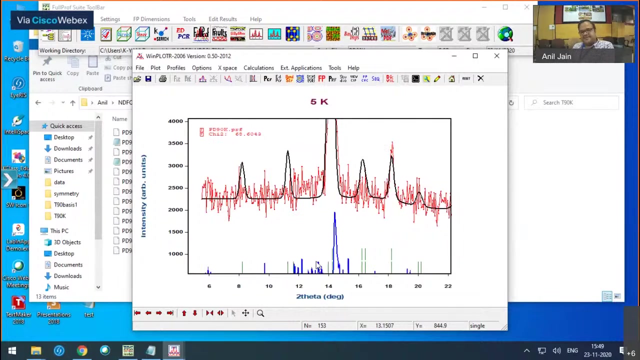 what I would like to do is I can put a small moment and try to see it what it does. So let me see, if I put the small moment, what it does. So now, what you can see clearly is that if I put this moment along this A axis, it is trying to generate some intensity at some location. 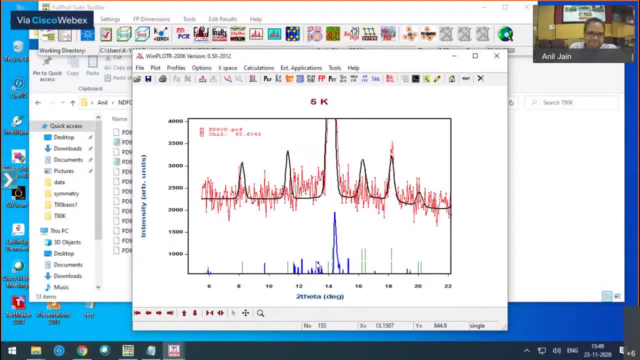 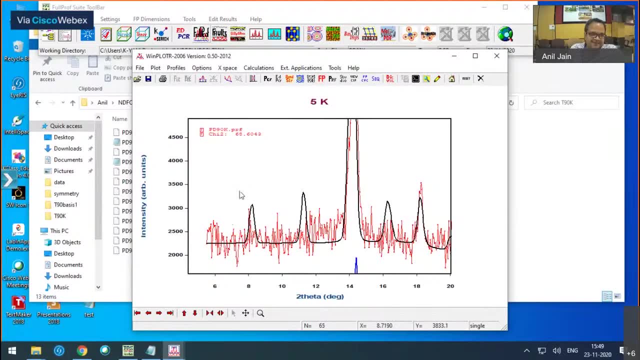 where I do not have any magnetic intensity. So it means I should have no component of the moment along this A axis for this refinement. This value of this temperature is wrong and this is wrong. issue is related with this comment line in the PCR file. this is 90k I can save. 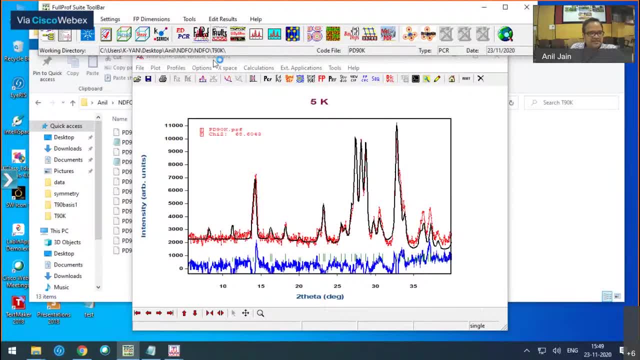 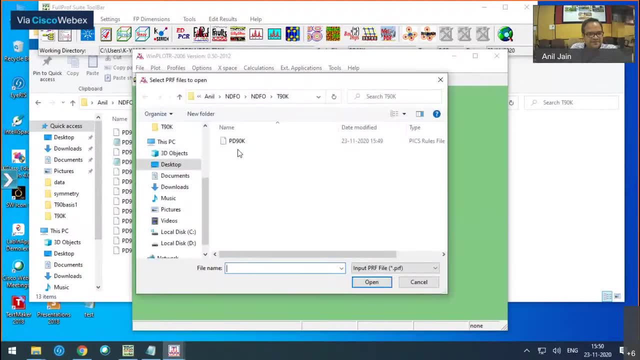 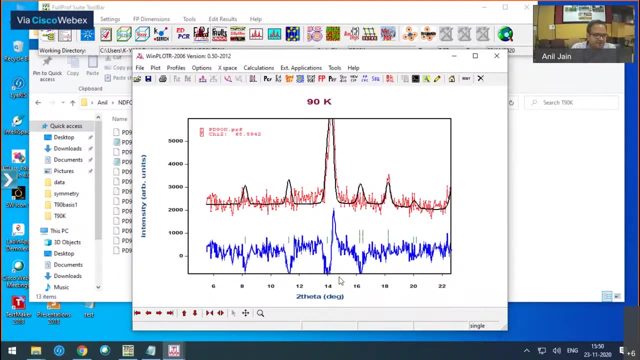 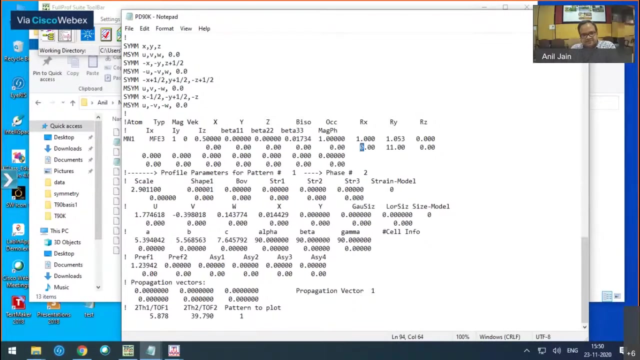 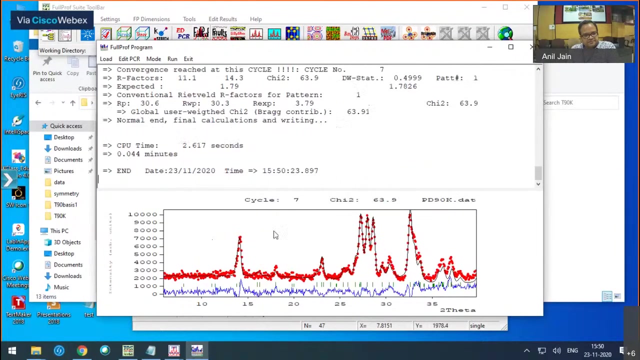 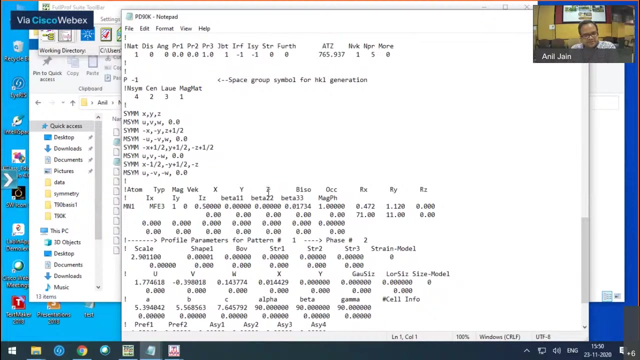 it and I can run it again. so, while reset here, yes, so you see that keeping this moment along this axis do not give us good fitting. I can try to see it by putting a refinement on this. you can see it becomes a small earth and in principle there is no intensity. 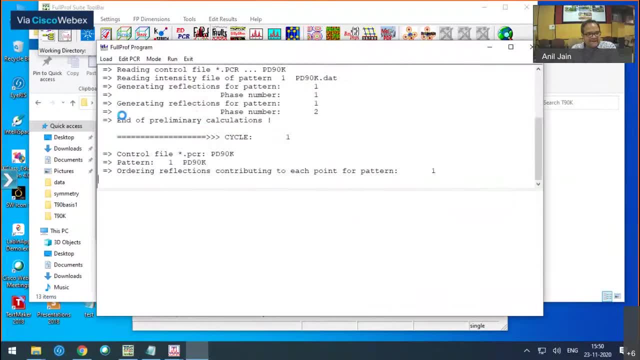 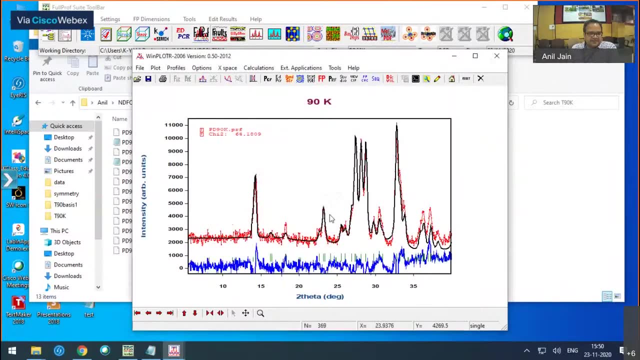 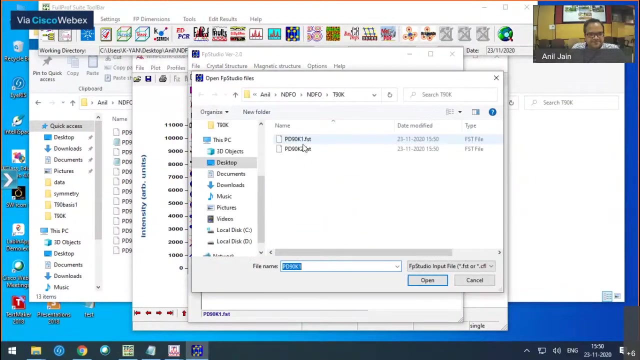 you can see it becomes a small earth and in principle, there is no intensity. So I believe what it is telling you is that your moments are along this B direction and again what you can do it here is you can again go to this studio, open it and you can see. 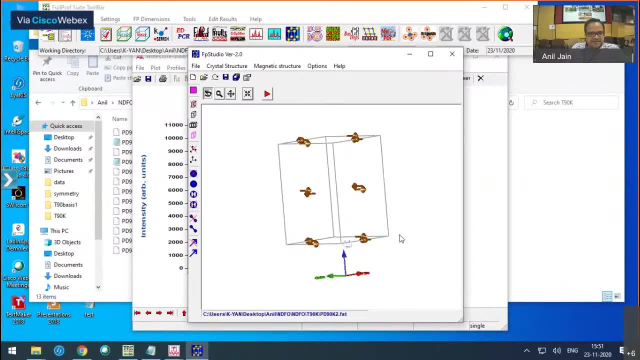 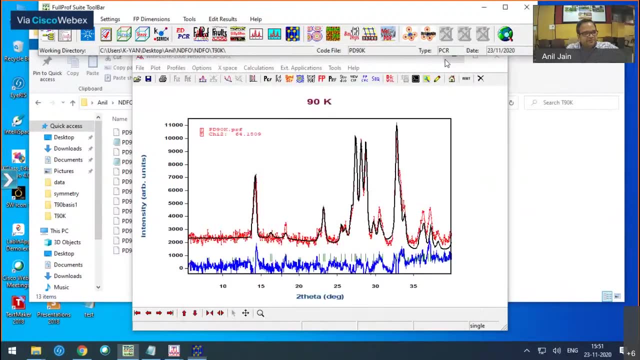 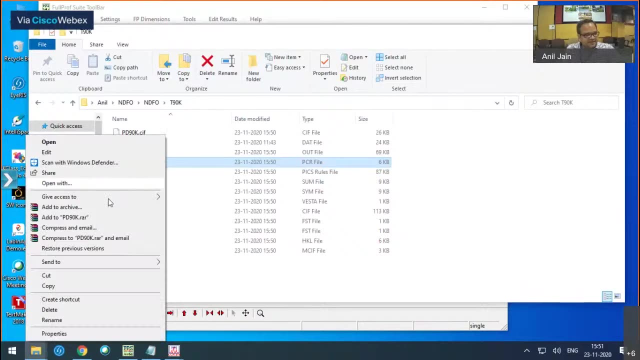 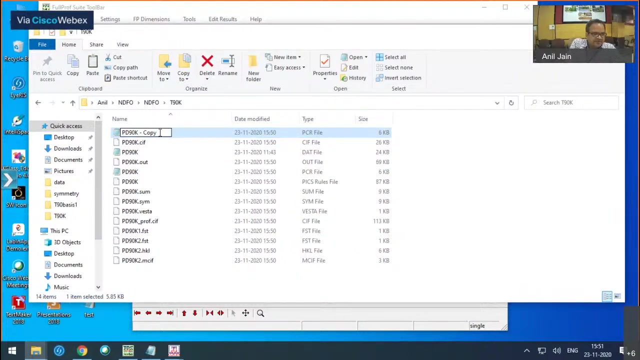 this magnetic structure or magnetic moment. So this is how we work for the magnetic structure determination. If you want to go for this other symmetry, then what I can do is I can copy this file, copy paste and let me put SIM 2.. 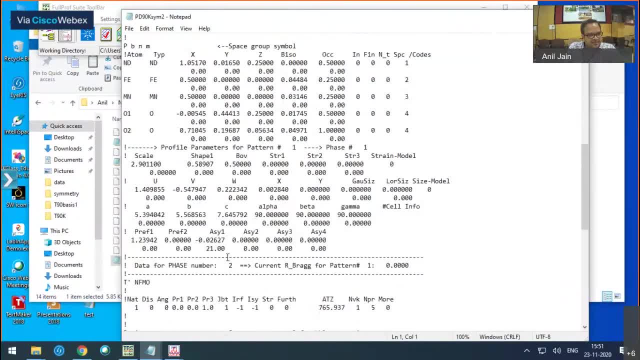 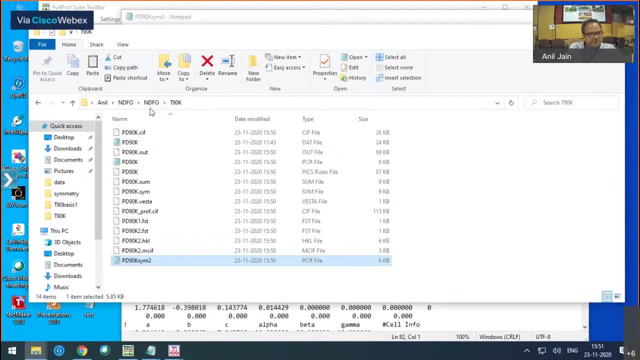 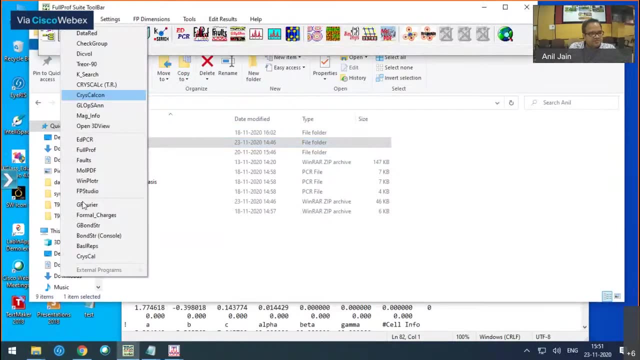 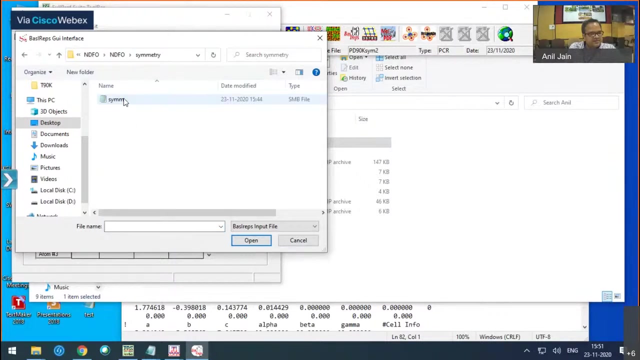 When I go again here- SIM 2, then I must change this operation. So what I do is to change this operation. I have to go in this symmetry calculation. Let me go to program base reps. open symmetry run Results. 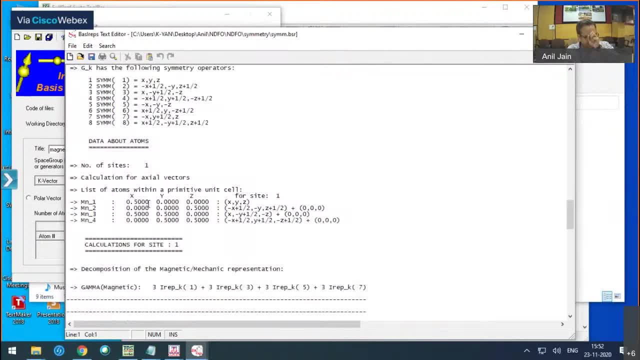 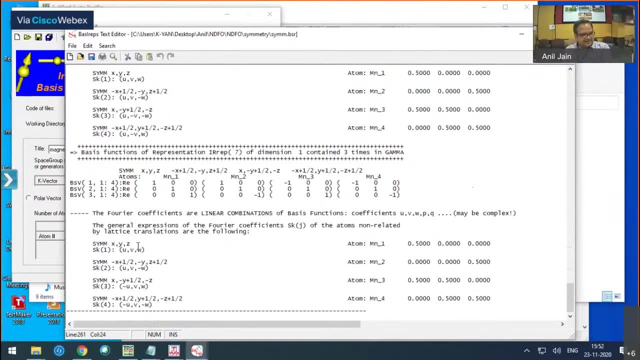 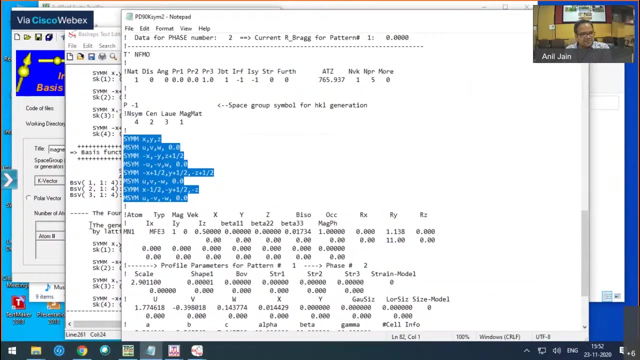 So we have done the exercise with this, I believe. Now let's go to this extreme end, This how it looks like. For this, what I have to do is I will have to change this, close this part, This part. I should change it. 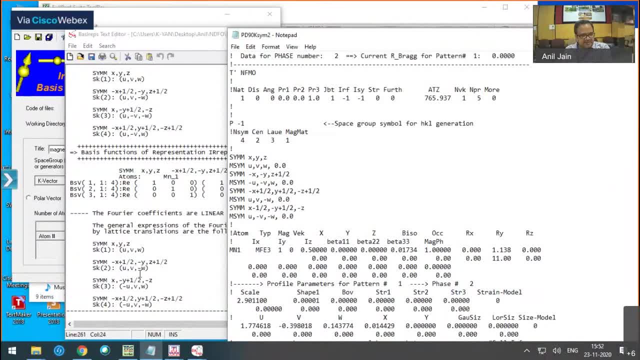 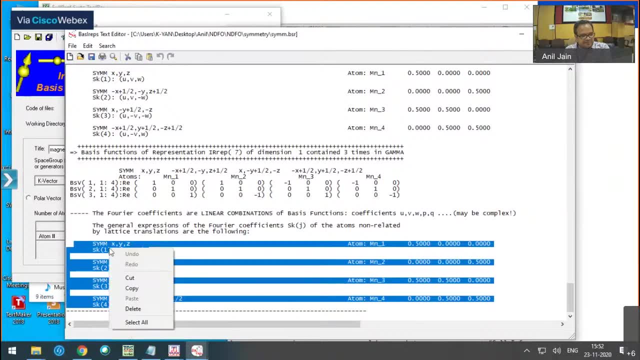 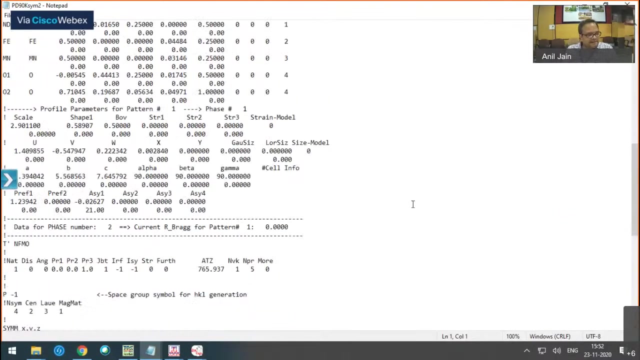 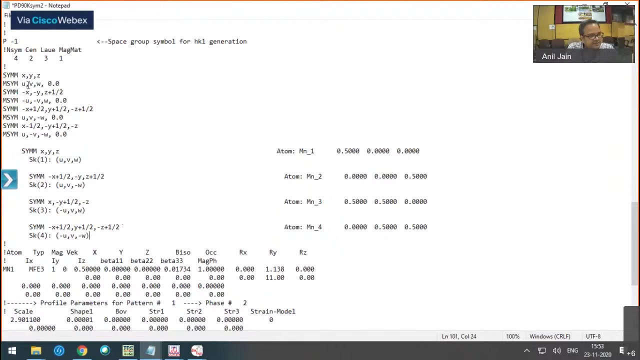 What I have is XYZ is YZ. Okay, Okay, Okay, Okay, Okay, Okay. And Oh, where is my PCR file? You paste it here And generally, this is so. this is UVW and this I put it as a second operation. here I put this: 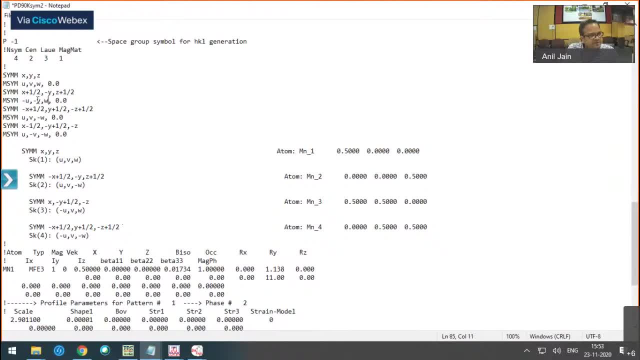 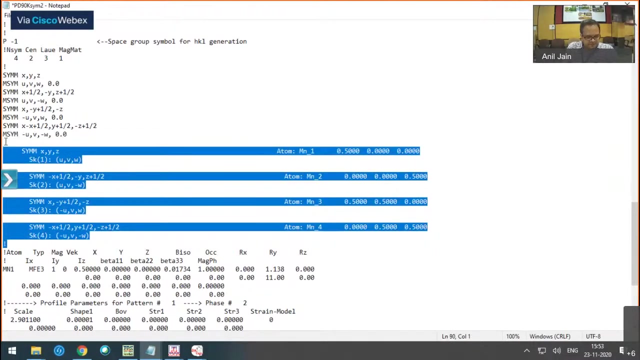 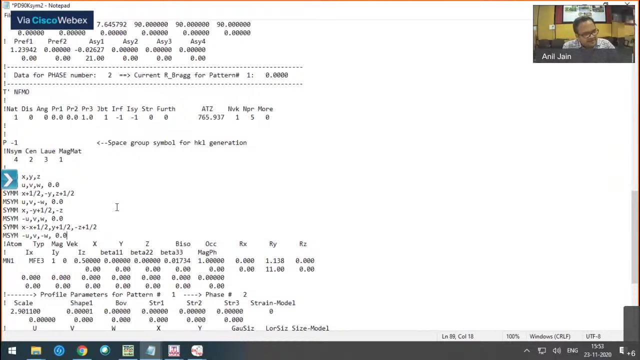 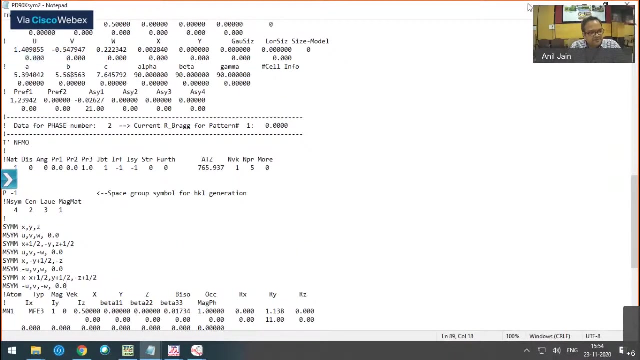 corresponding codes UVW here. similarly, this is the operation number 3 and these are the codes UVW. and okay, so now I have copied, paste all this information so I can delete now this part. rest. everything remains again the same. and let me see now what happens with this representation. so I do it now. I save it, close it, let me. 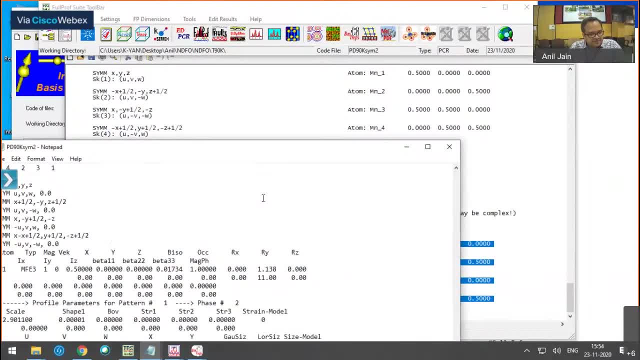 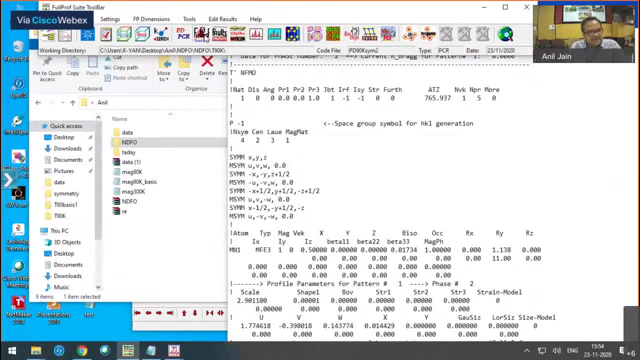 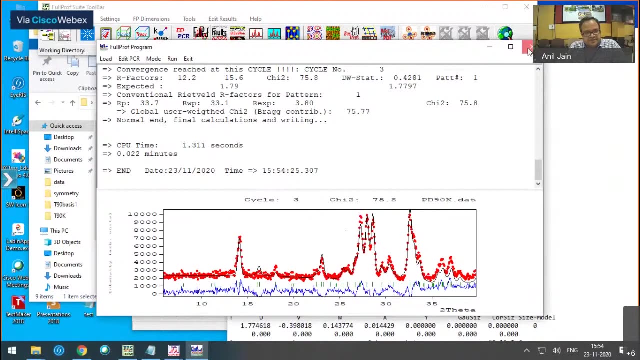 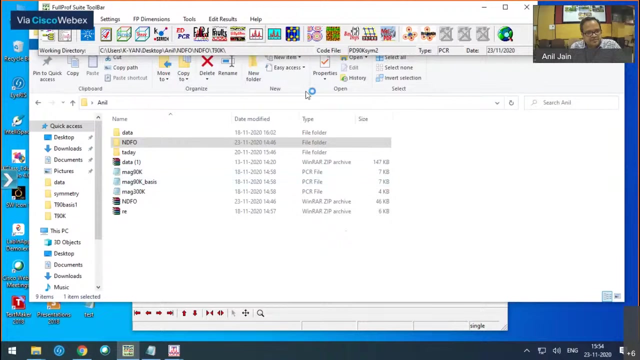 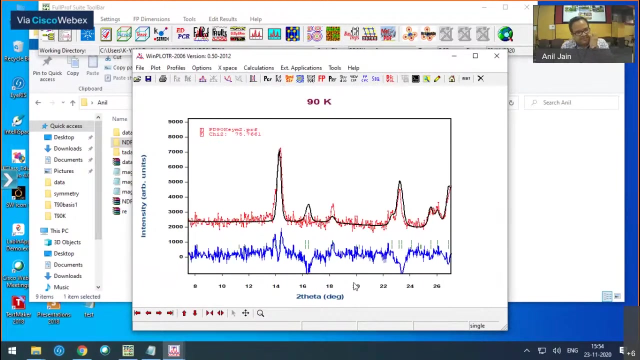 just open this file again and see it okay. so I close this now and I try to run it. so in this representation, if you see I The problem is. problem here now is with this representation. of course you are getting the intensity for the first peak, but this kind of magnetic structure is also giving you some 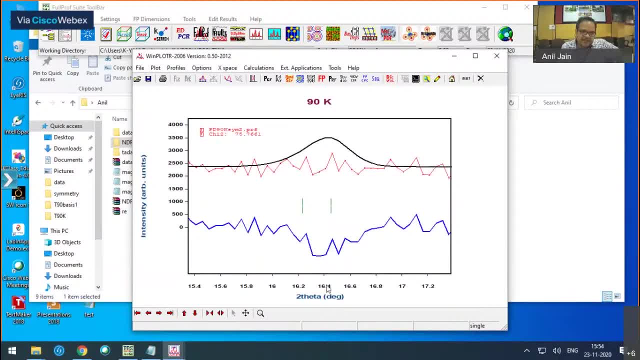 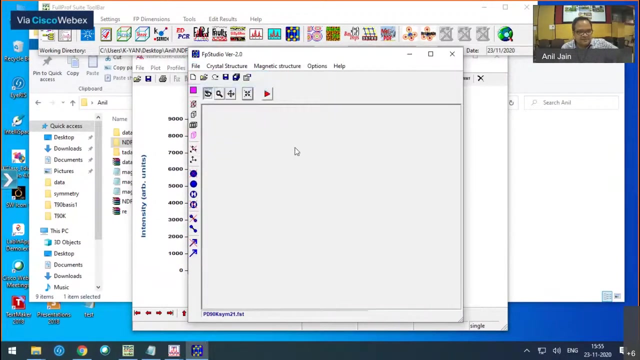 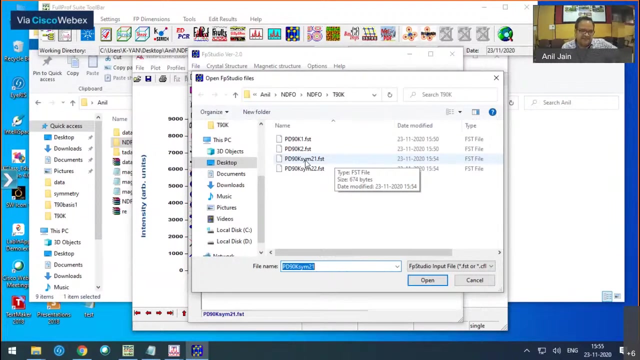 intensity for this second peak which is shown here, where in principle you have hardly any magnetic intensity. So this indicates that previous magnetic structure was better than this. So this I have done for the second and you can see how the magnetic structure looks now Open. So it creates this two way full prop studio file. First one is generally for 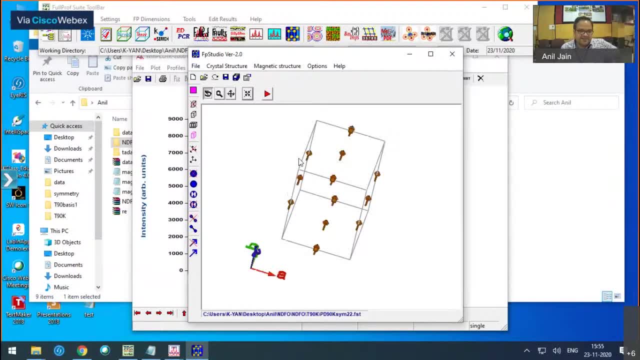 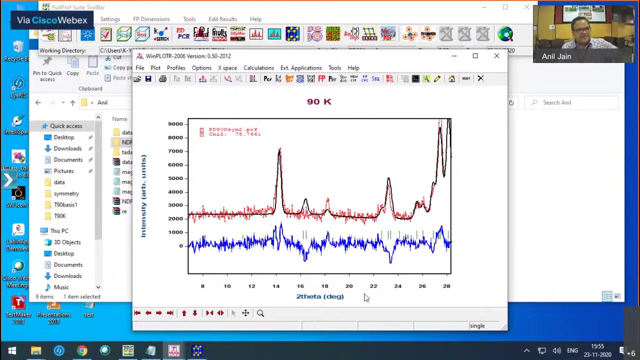 the structural, and second one is for the magnetic phase. So this is the another file. So this is how you can see how this magnetic moment are arranged and whether this observed intensity gives this satisfactory diffraction pattern as what you have observed in the experiment. So I have done it for this second representation. 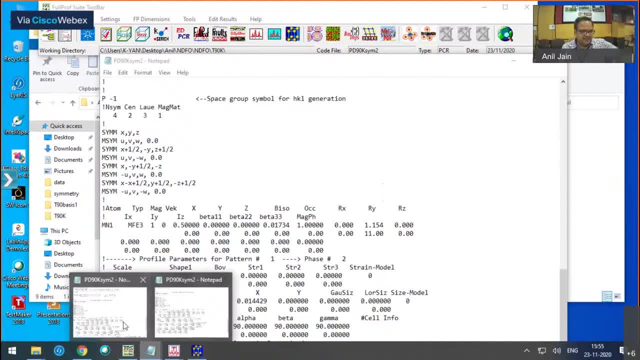 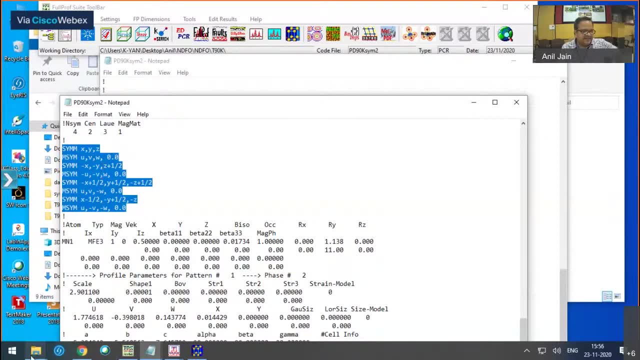 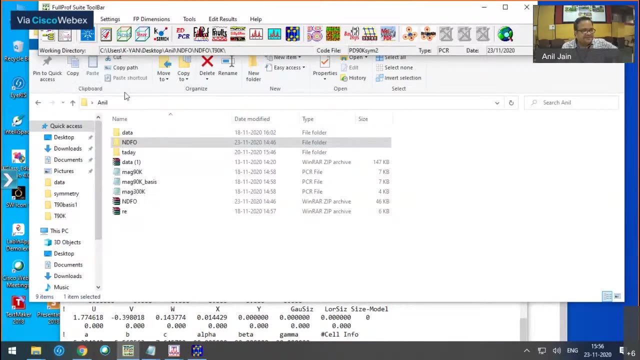 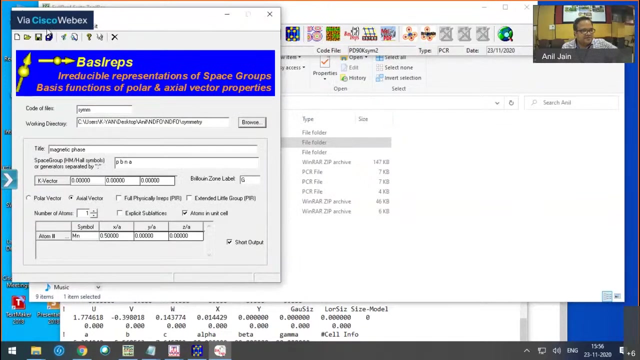 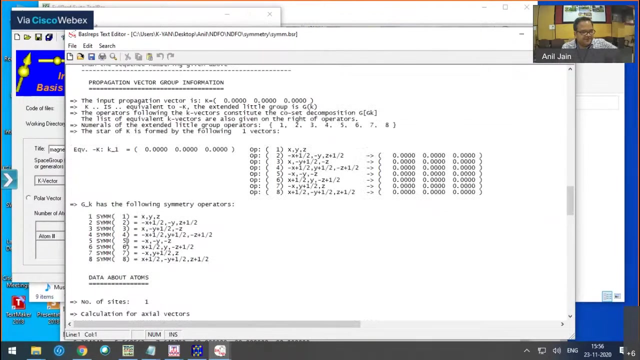 Similarly, you can go ahead and do it for this number three, Number three also, in which case I have to modify these three lines and replace them what has been given by this base reps. So base reps again can open it. This was my symmetry analysis. I can run it just to make sure things are all right And then we have worked for. 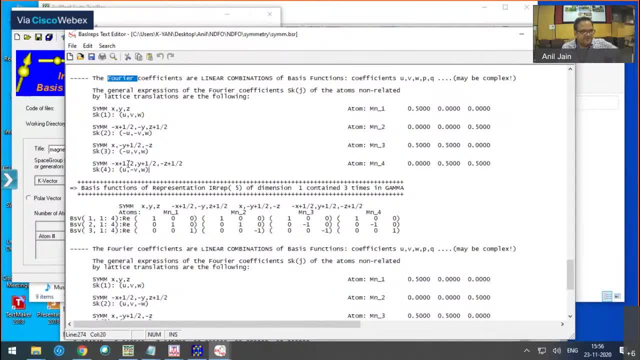 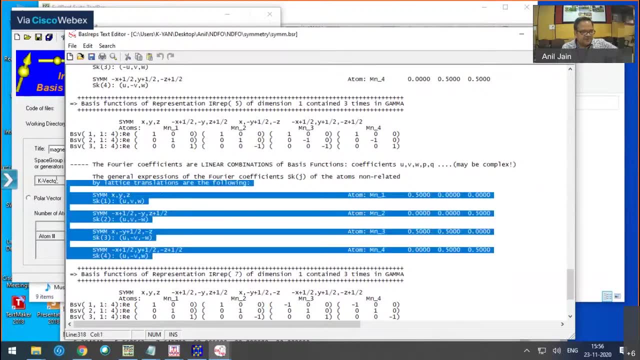 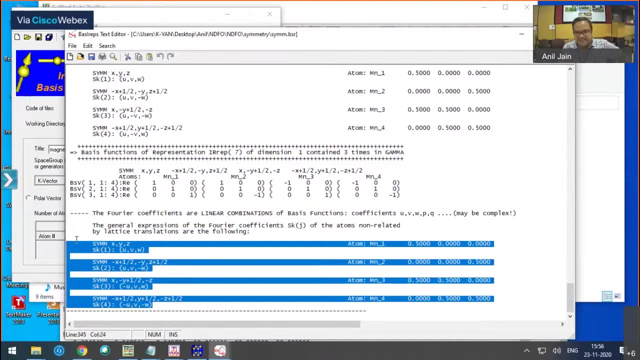 this. Sorry, Number three, Number one, which was giving good fit. Number two was not good. Similarly, you can go ahead. Sorry, This was number two. Similarly, you can go ahead and try for this other representation and try to see whether you are getting magnetic intensity or not. 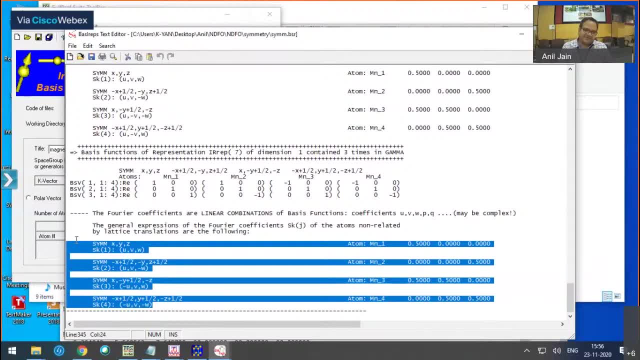 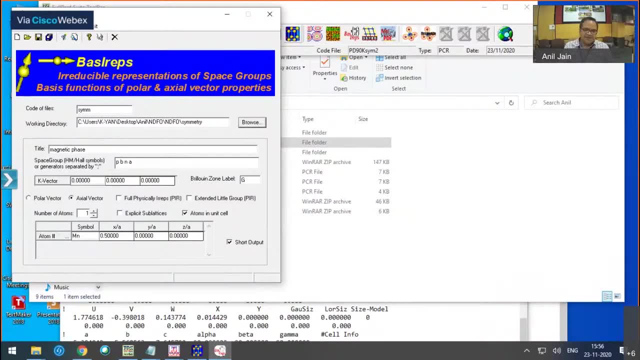 This is how we work in the determination of the magnetic structure. So with this now, I would like to stop it here and if you have some questions, you can tell me now. I think some of you have asked for this data file and that, I believe, PCR file, which now 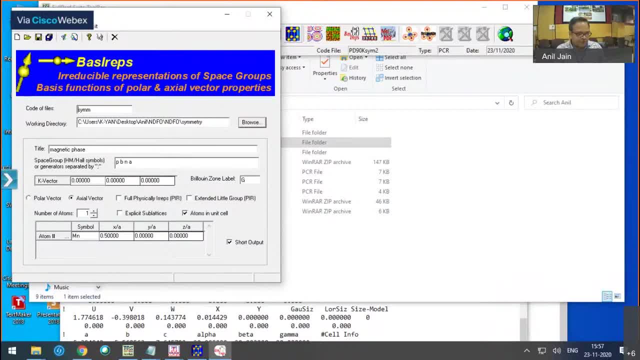 I will be sending, But I think it would be nice if all of who you needed can send the email so that I can fix it. Okay, So I think it's a good suggestion, So I will try to give by today evening or tomorrow. 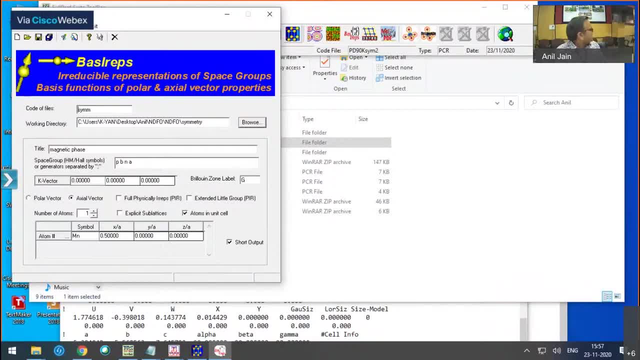 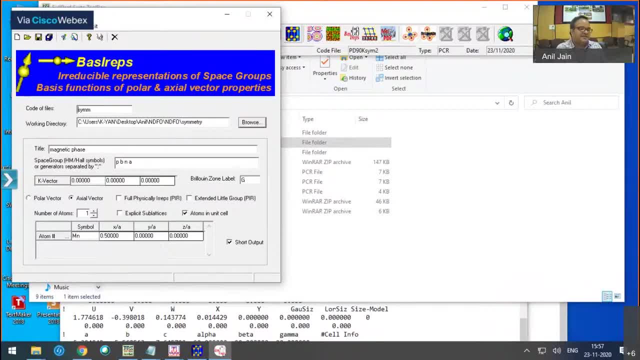 You can download, and I will put this PCR file also and probably this file for this BAS-REPS, which file is called SMB file. So the file which is opened in this BAS-REPS program has extension SMB and what you can do is, in future, for your magnetic structure, you can only modify. 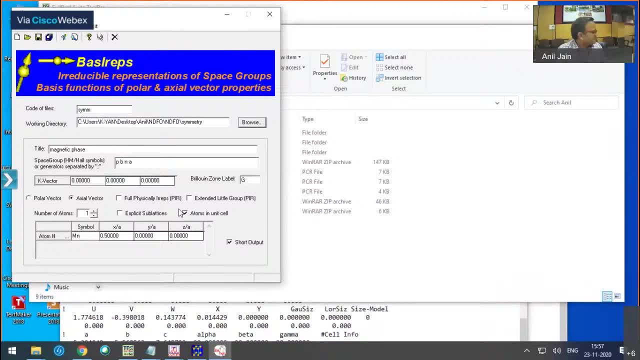 this file and then try to see this representation. And also they have not given us SMB into the data. Trust me, Only a part for the your one. many of you have also not submitted the assignments for the theory of neutron scattering. you are requested to submit it as soon as possible. i would like to upload.